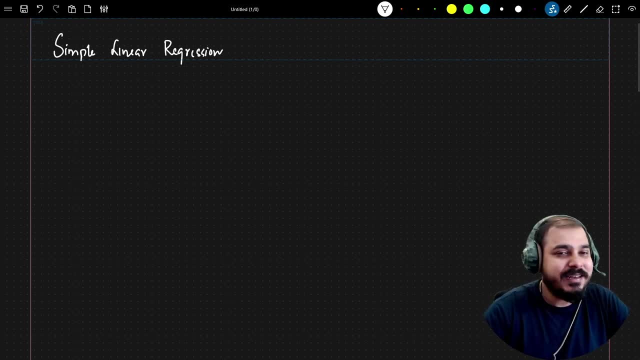 We'll learn our first machine learning algorithm, which is called a simple linear regression. This is a super important algorithm because the techniques that we are going to learn in this will also be applicable in deep learning, when you're probably learning the first neural network, which is called an artificial neural network, right? So it is super important. we try. 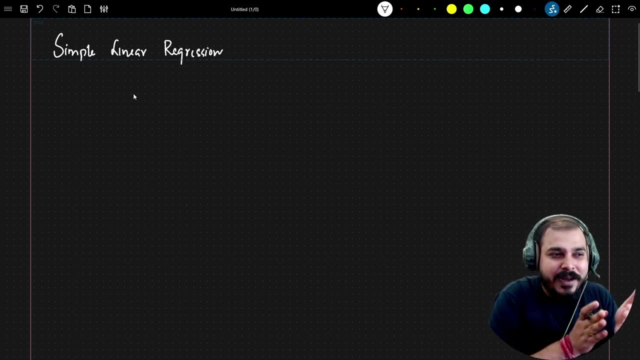 to understand this And remember this machine learning algorithm. I'll try to break down this into separate, separate modules so that you can understand it in a better way. Now, what kind of problem statements do we solve with simple linear regression, As the name suggests, regression. 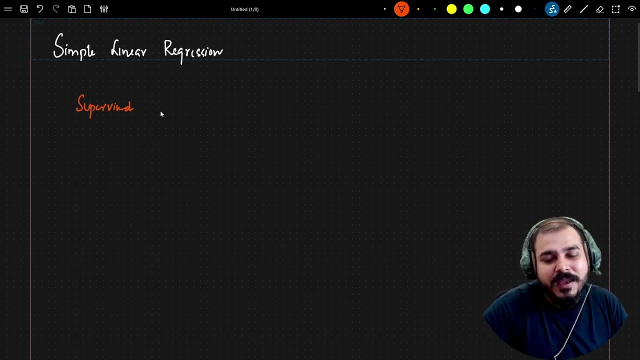 so definitely in supervised machine learning technique. if you have a regression problem statement, we can definitely solve it with the help of simple linear regression. Now what exactly simple linear regression algorithm is all about? Let's say that I have a specific and easy data. 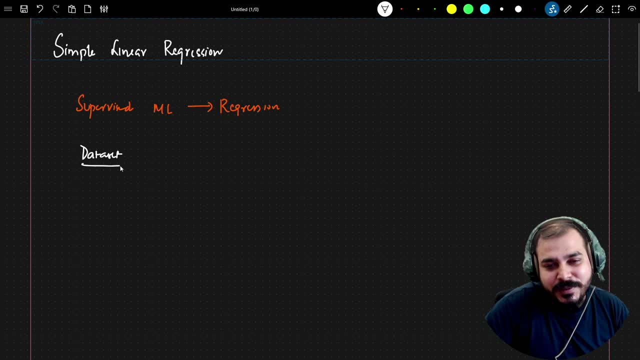 set. okay, Let's say I have a data set and this particular data set has features like age and- problem, Probably- weight. or instead of writing age and weight, let's basically just write something like weight and height. okay Now, as I said, regression problem statement. obviously I will be having some. 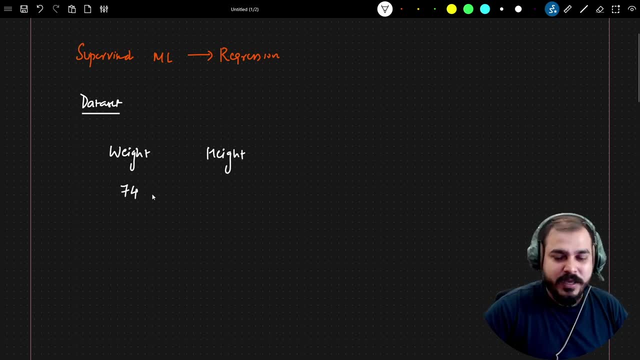 data parts. Let's say, if the weight is somewhere around 74 kgs, my height may be 170 centimeters. If the weight is 80 kgs, the height may be 180 centimeters If the weight is somewhere around 75. 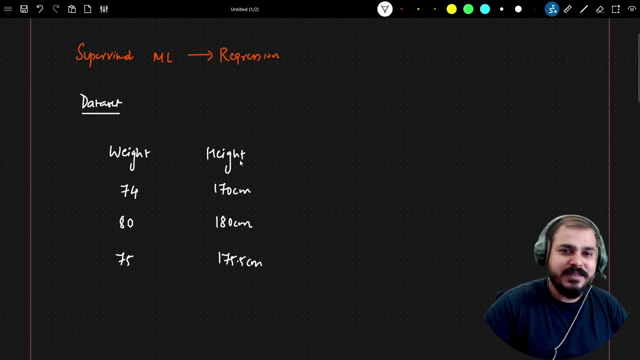 kgs, the height may be 180 centimeters. If the weight is somewhere around 75 kgs, the height may be 175.5 centimeters. Let's say this kind of data set I have. okay, Now, in this particular data set, 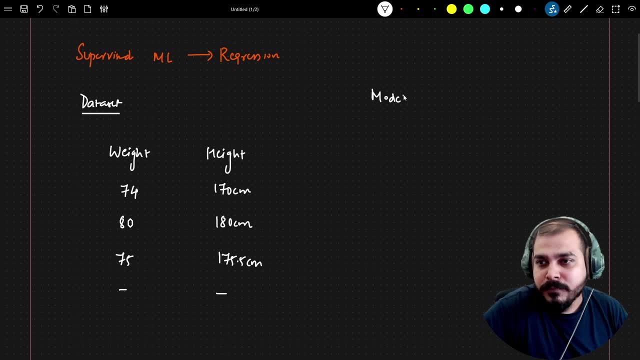 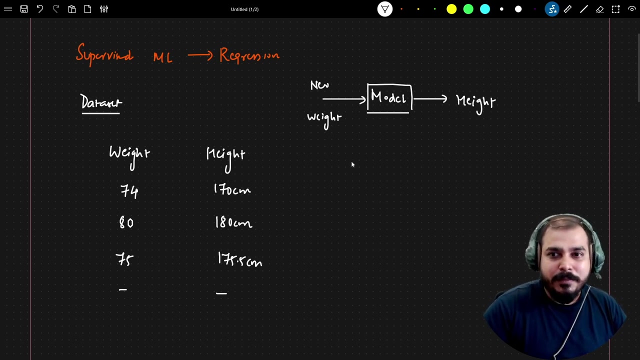 our main aim is that we need to train a model and this specific model. whenever we give our new weight, new weight, it should be able to predict the height. okay, This should be able to predict the height, And now you just see this? okay, So this feature is basically our. 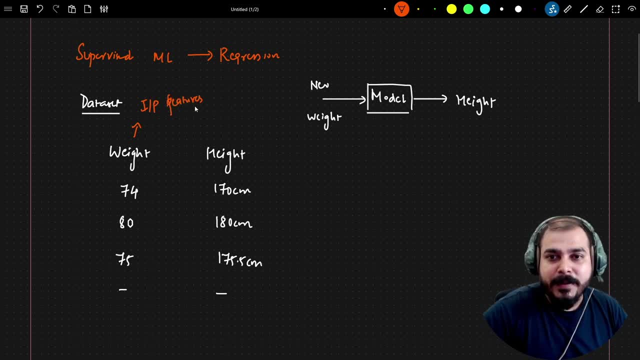 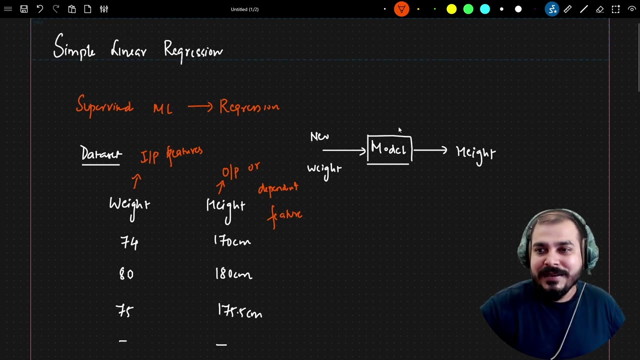 independent features: Independent features, and this feature is specifically our output or dependent feature. okay, Dependent feature. So this is what we are planning to do, and this model that we are going to train is with the help of simple linear regression. okay, Simple. 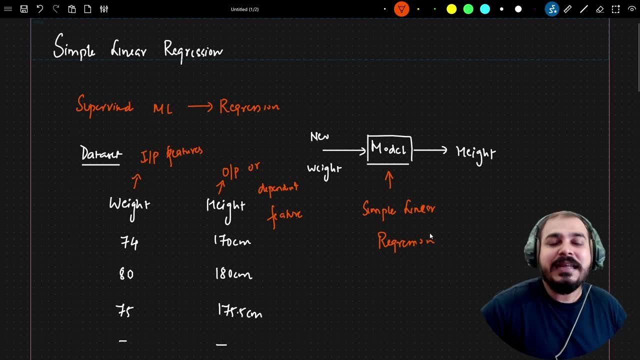 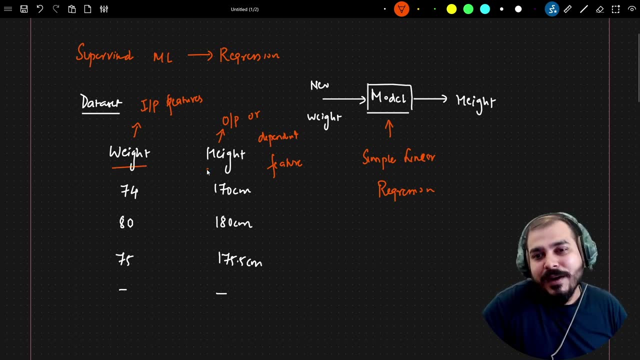 linear regression. Now, why do we say it as simple: linear regression? Understand over here. how many input features are there in this model? How many input features are there in this model? How many features we have over here? We just have one input feature and one output feature. Whenever we just. 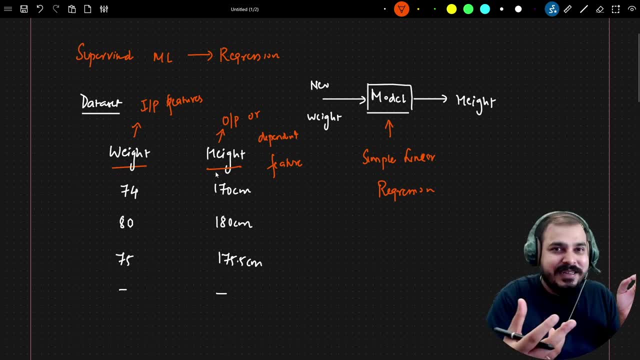 have one input feature, then we say it as simple linear regression. If we probably have multiple input feature, then we can basically call it as multiple linear regression. But it is very important to just understand simple linear regression. then automatically, whatever terminologies and maths that you probably will learn in this will get applied to multiple linear 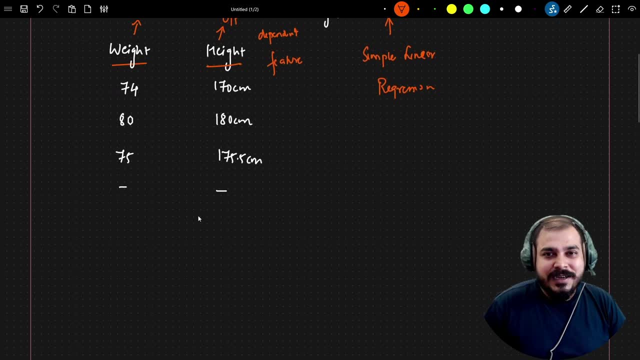 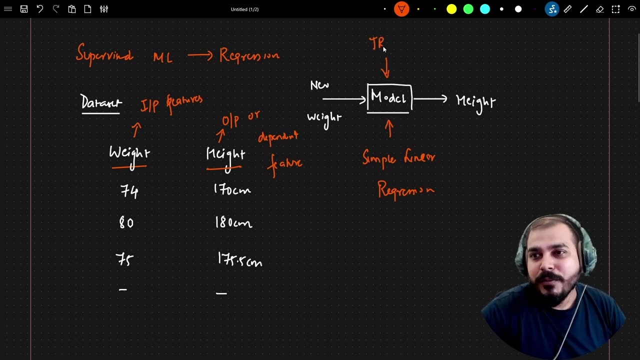 regression also, okay. So, in short, what are we trying to do? As I said, for this specific model, we will train it. We will train it with this specific data, okay, And later on, this model whenever it takes new weight. 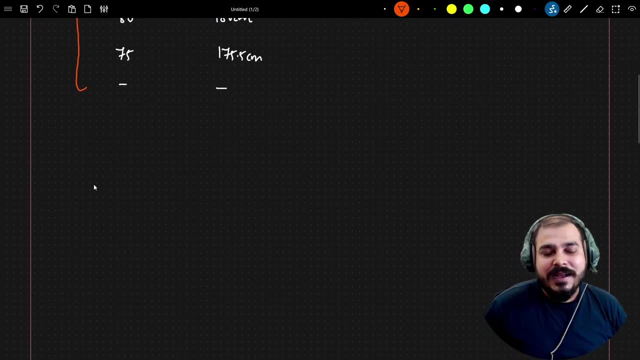 should be able to predict the height. okay, If I really want to show you in a geometric way what are we trying to do, Let's say: this is my weight and this is my height. Okay, Now, with respect to this particular dataset, let me plot some points. Let's say there are some. 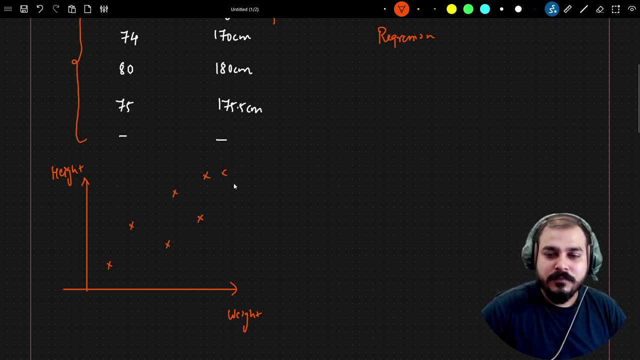 points which are plotted like this. okay, So, with the help of simple linear regression, what we are trying to do is that we'll try to create a best fit line, okay, And this best fit line will actually help us to do the prediction for the new weight. So let's say: how does the prediction happen? 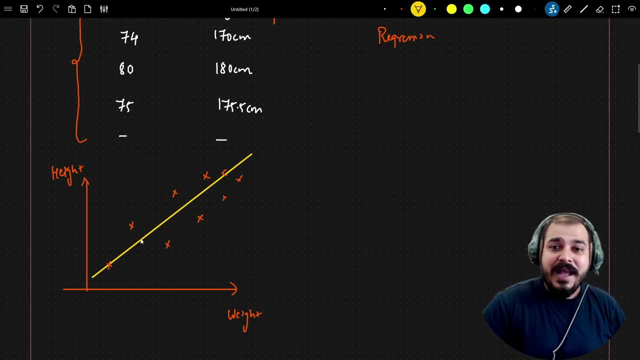 Let's say, once we get this best fit line, okay, And this best fit line should be created in such a way that you know that distance between the true true points- So true points, basically means these are my true output, right, These are all of my true output. 170. 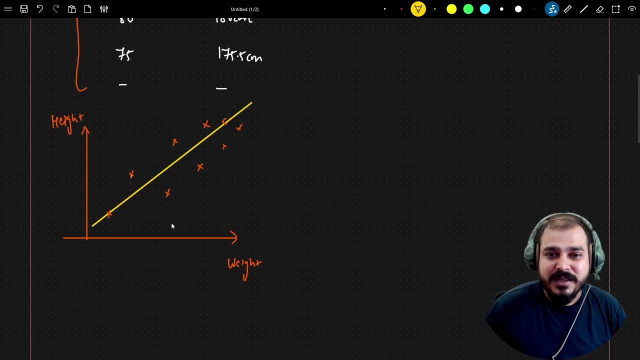 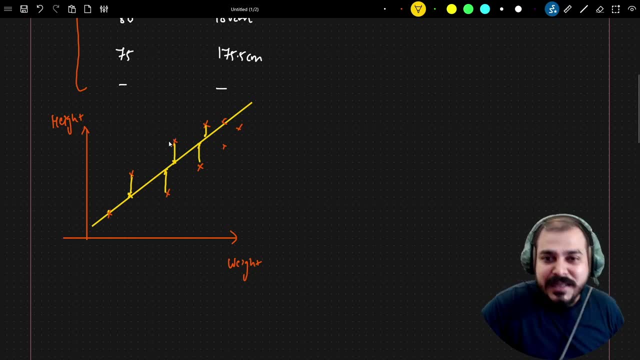 all this distance and this is basically the error, right? Because these are my true points and these are my predicted points. So right now, just understand. till here. I will again explain in more detail, right? So this distance should be: if I do the summation of this distance, it should be minimal, And that is the technique we. 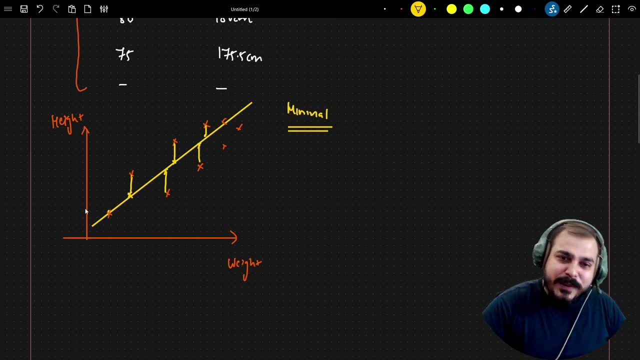 basically use to select the best fit line. Now, once we create this best fit line, whenever we get a new data point, let's say with respect to this particular weight, how do we predict our output? What should be the height? All we do is that we try to. 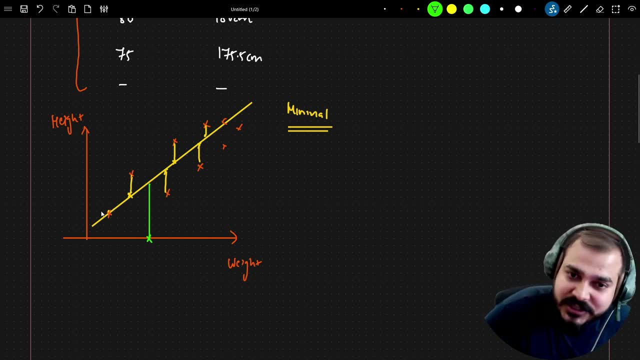 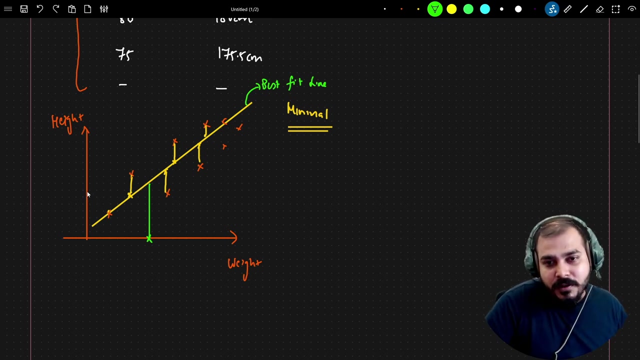 just put this line on this particular C and we just try to see where this point meets this particular line, which is my best fit line. This is basically my best fit line, Okay, And then we try to see where in the Y axis it is basically meeting. Okay, So suppose, if it is meeting at this, 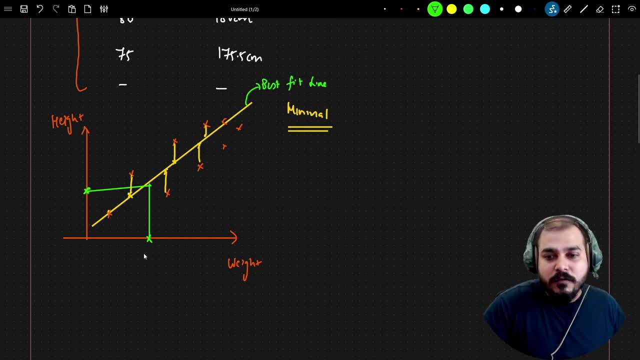 particular point. so this specific is my output for this specific weight. This is what we actually do in simple linear regression. Okay, Over here, the main is that we just try to create a best fit line, such in, whenever we give our new weight, we should be able to: 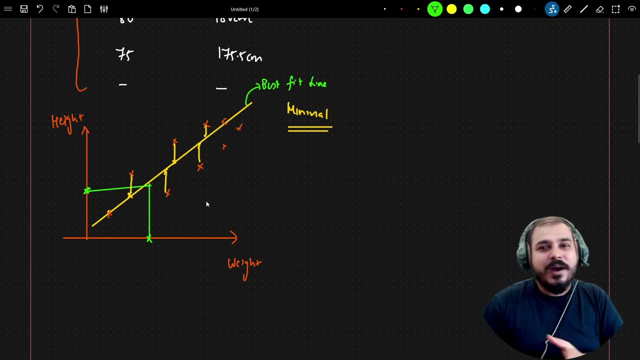 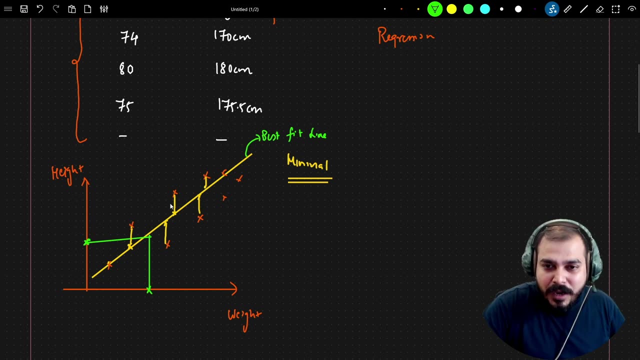 predict what should be the height. Okay, Now, as we go ahead, let's understand what is the mathematical equation of this particular best fit line. And when I spoke about this error, what is this specific error? we'll also try to understand And we'll try to understand in a very 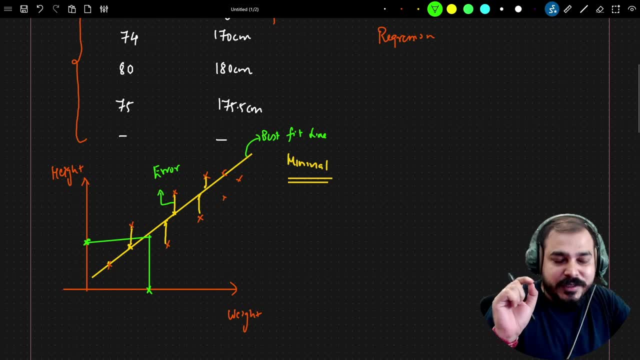 amazing way, Okay. So, guys, we are going to continue the discussion with respect to simple linear regression. We have understood, you know, what is our main aim, what we are actually trying to do with the help of simple linear regression. We are 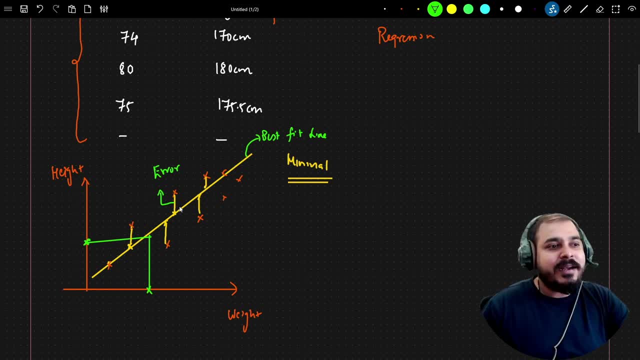 actually trying to create the best fit line, But before we go ahead and understand the maths behind it, we really need to understand some of the notations that I'm actually going to use while explaining this entire machine learning algorithm. So let me go ahead and let me again consider this. 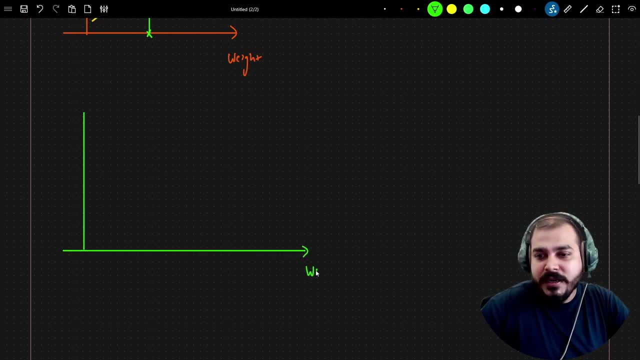 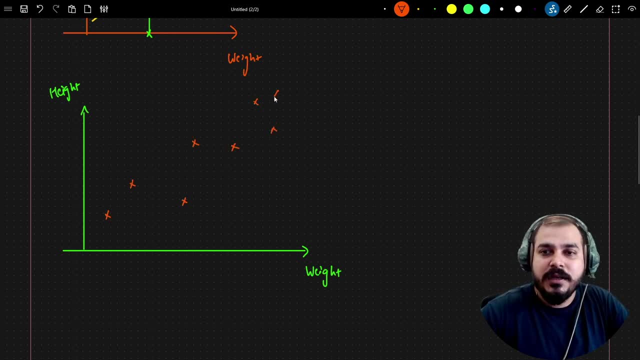 which are like this. let's say, I've just randomly created some points, And this points basically mentioned our data set right, Whatever data set we have, Right, And this points only. we are going to train our specific model, you know, uh, and what we are planning to do is: 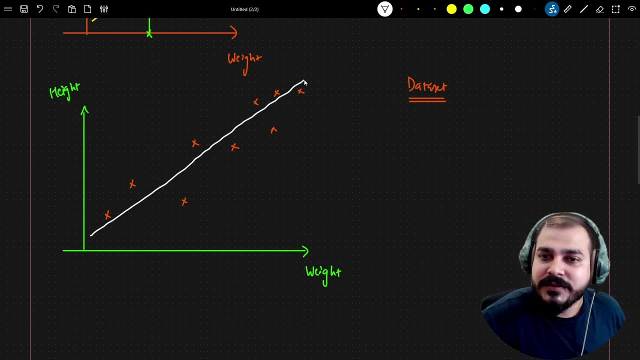 that we are planning to create a best fit line In this right we are trying to create this best fit line. Now, in order to create this best fit line, we basically provide some equations to this best fit line. you know, you can basically use the equation of a straight line like: y is equal to mx. 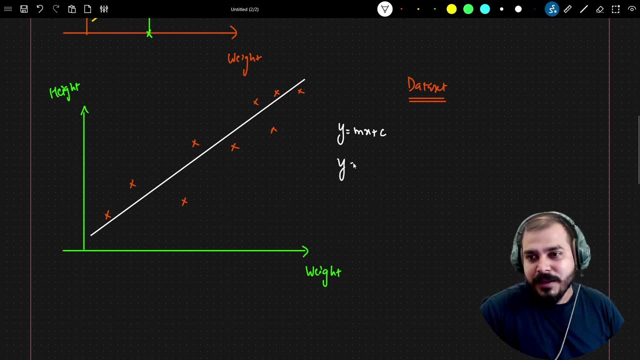 plus c, or, if you have seen some of the research paper they may also use, something like: y is equal to beta 0 plus beta 1 multiplied by x. you know um. and you may also have another equation, uh, which, uh, you know. andrew ng also uses this specific equation when he teaches it, you know. so he uses. 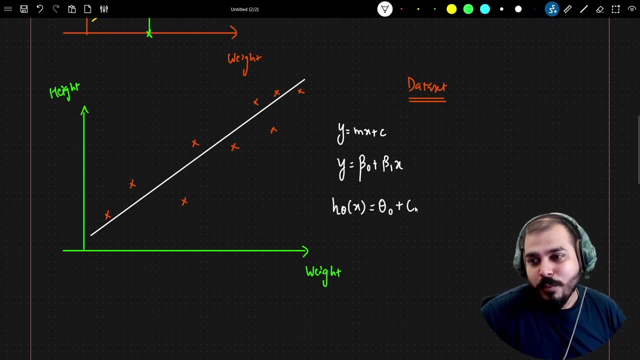 h, theta of x, which is nothing but theta 0 plus theta 1 into x, right? so this equation, so in this entire simple linear regression that i'm actually explaining again, some amount of credits- yes, definitely goes to andrew ng- is quite amazing with respect to teaching any kind of topics, so i will. 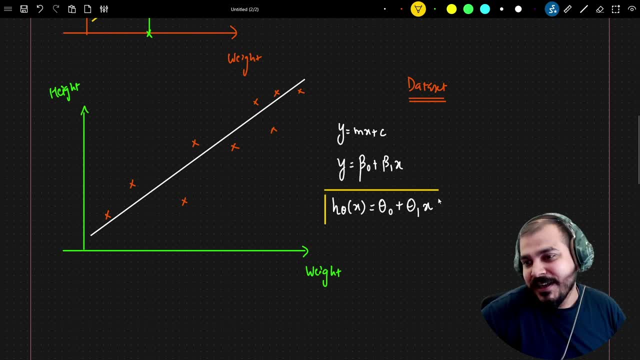 also be using this specific notation, which is basically nothing but h. theta of x is equal to theta 0 plus theta 1 into x. okay, now, here, if i talk about x, x basically means my independent feature. now, in this particular case, it is weight. okay, now let's go ahead and let's try to understand what is theta. 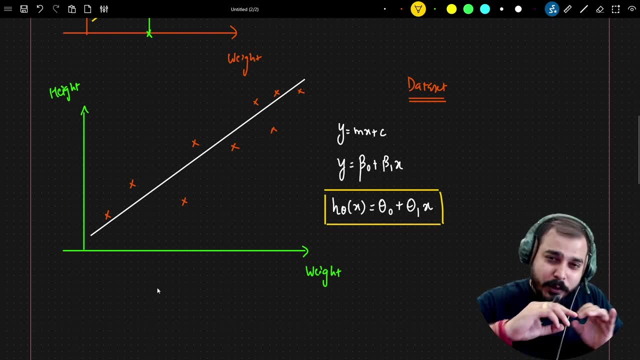 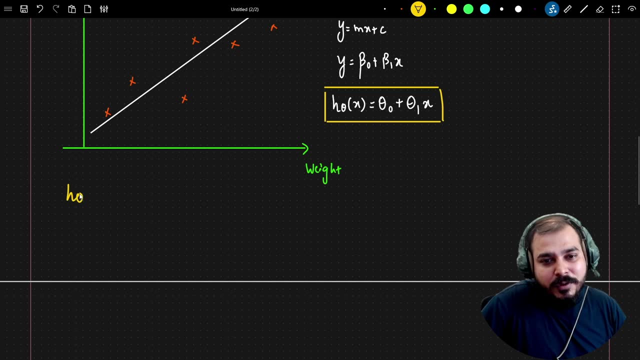 0 and what is theta 1? that is the most important thing that you really need to understand in this best fit line. okay, and what is this? h theta of x. okay, so over here let me write down the equation: h theta of x is equal to theta 0 plus theta 1 into x. now, first of all, what exactly is theta 0? 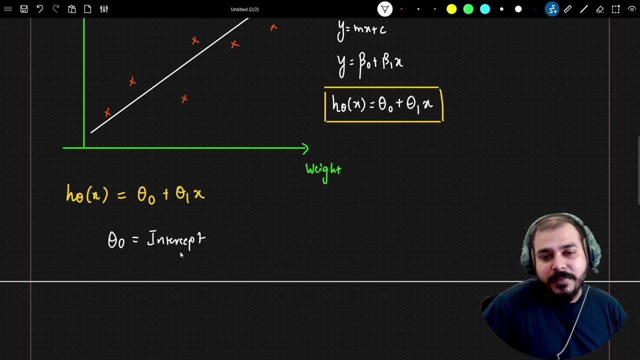 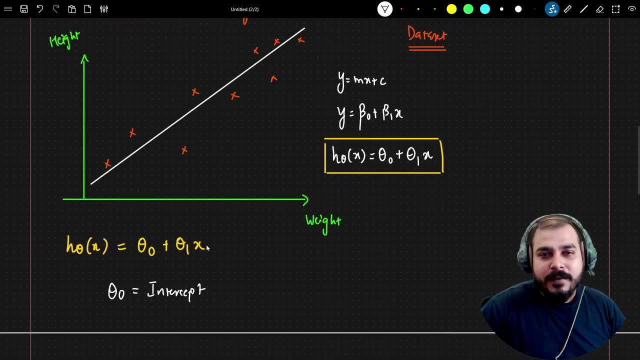 so theta 0. we can definitely say it as intercept. why do we say it as intercept, intercept? in short, let's consider that if my x value is 0, then what will happen? if my x value becomes 0, then what happens? h theta of x is nothing but theta 0. now, this basically indicates that 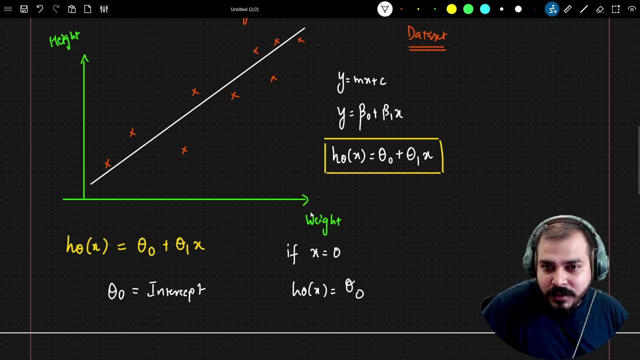 when my x value in this particular- uh, you know in this line that i am actually drawn right- weight is my x in the x-axis, right? so when weight is 0, where does this particular line meet at the y-axis? okay, so this particular line, you will be seeing it, meets somewhere here at the 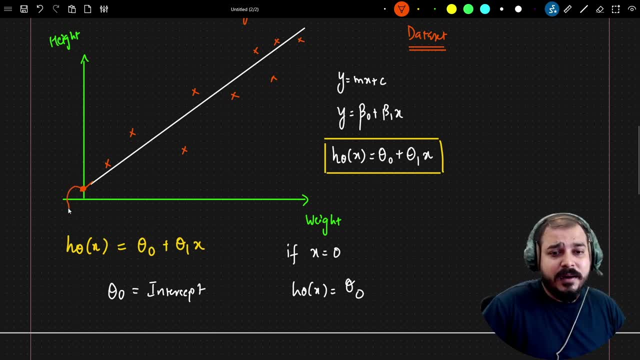 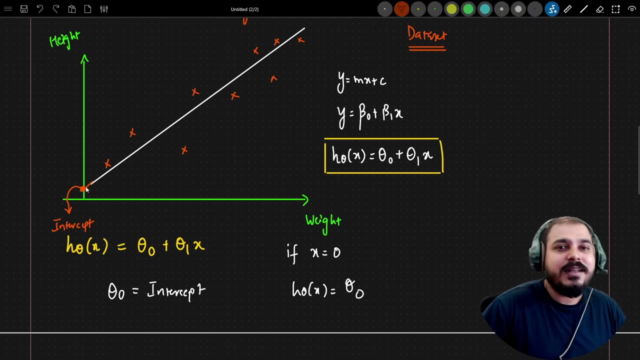 y-axis. so this particular point is nothing, but this particular point is mentioned as intercept. so, in short, what does theta 0 basically indicate? it basically indicates the intercept. that basically means, when x is 0, what is the value of theta 0? okay, so theta 0 wherever it is meeting the y-axis. 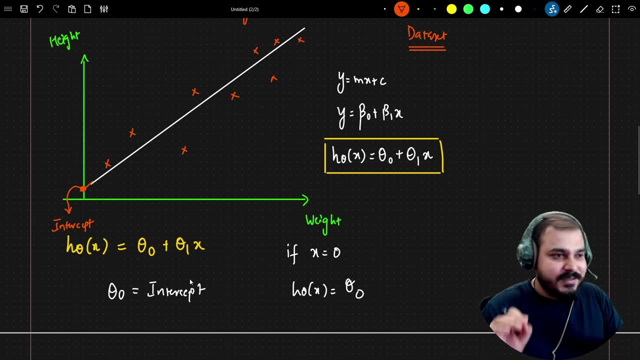 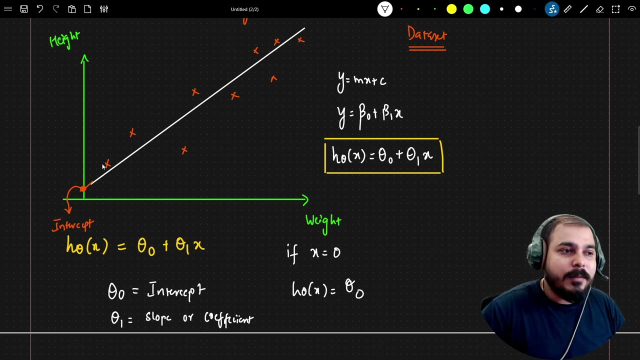 that is basically called as intercept. okay, so this is the first thing that you really need to know, very, very important. now let's go and understand what is theta 1. theta 1 is nothing, but it is called a slope or coefficient. okay, now, whenever i talk about slope or coefficient, what does this? 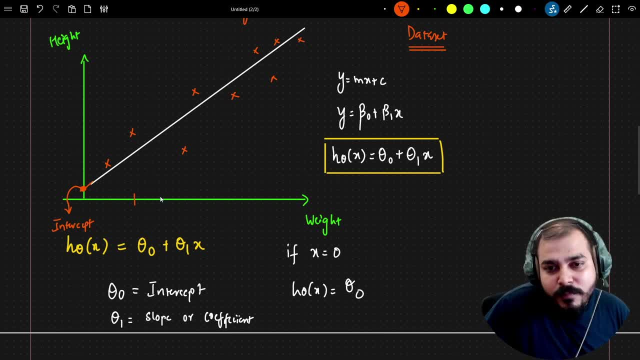 basically indicate? this basically indicates that with the unit movement in x-axis, suppose, if there is a unit movement in x-axis, so if i try to plot this over here in the y-axis, we are just going to try to see that what is the, what is the movement in x-axis? so if i plot this over here in the y-axis, 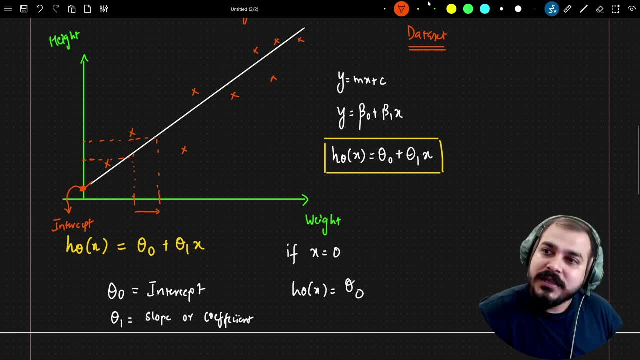 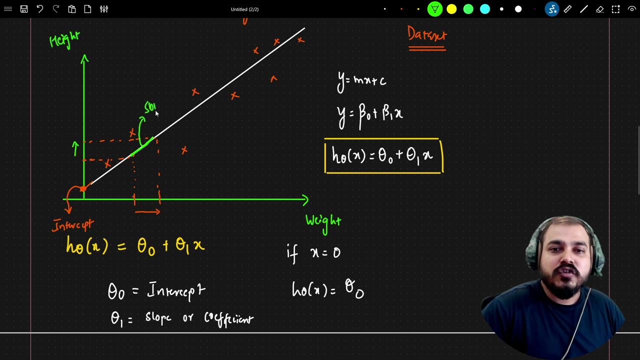 with respect to the y-axis. so, in short, what is this slope movement? okay, so this is the movement that we are trying to see. so, with the unit movement in the x-axis, what is the movement with respect to the y-axis? that indicates something called as slope. okay, so very simple. 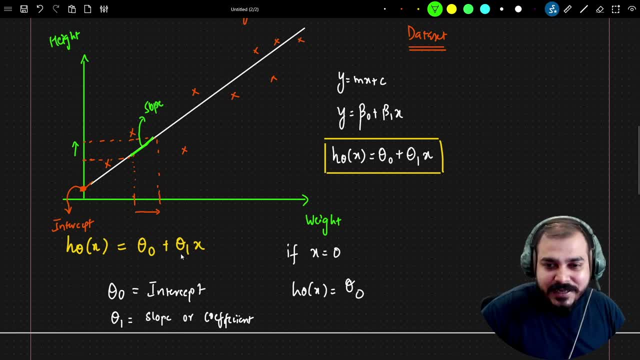 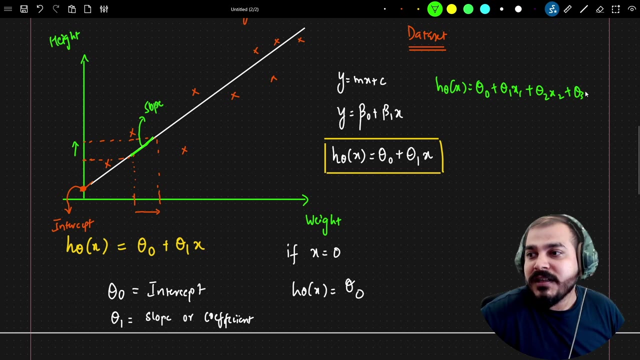 this is also called a slope or coefficient. that is basically indicated by theta one. okay, suppose, if i have many, many independent features, then this equation becomes something like this: h theta of x is equal to theta zero plus theta one x one plus theta two x two plus theta three x three. 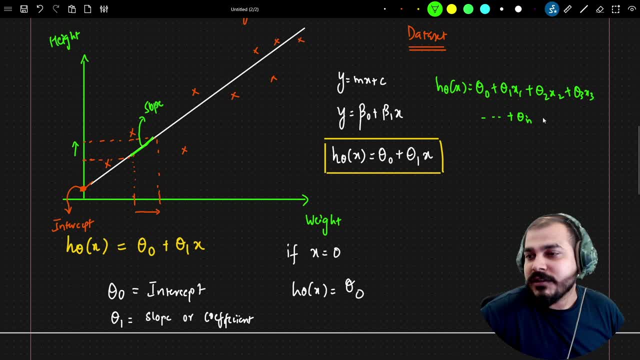 like this up to theta and xn, so i can just write theta and xn. so this basically indicates that i have many, many features. so definitely i'll be having that many number of slopes like theta one, theta two, theta three till theta n. but here, since i just have one independent feature, so i'm just 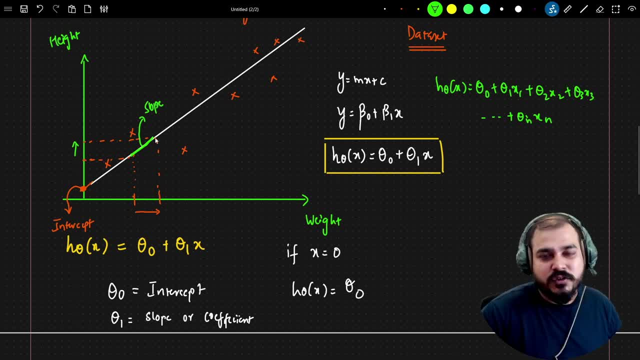 going to basically say that, okay, i have just one slope, okay, one slope. now. this is the basic understanding with respect to theta zero plus theta one x. right, so x is nothing but my data points with respect to the x-axis. now one more very super important thing now, as i said, that once we create a westward line, 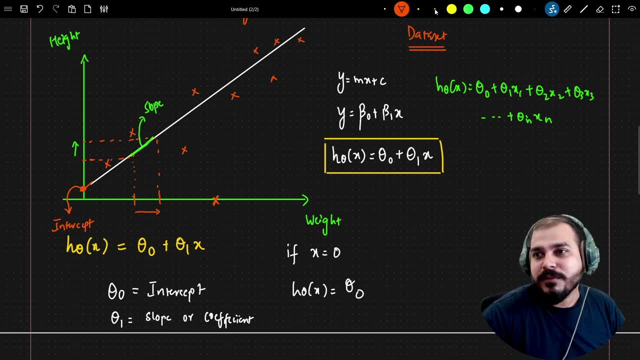 whenever i get a new data point, let's say, this is my new data point with respect to weight. okay, with respect to weight, this is my new data point. then how do i predict my height? all i do is that i try to project this over here and i try to basically see what is my y value. okay, so this is basically my y value. so this point. 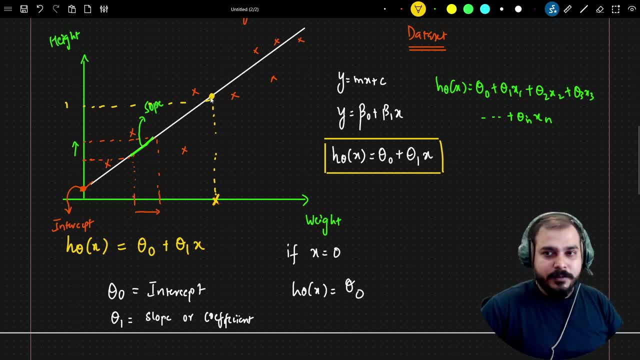 i can say: this is my predicted point, right, predicted point. so whatever points i'm actually predicting over here, that is mentioned by h theta of x. so h? theta of x is nothing, but this is basically my predicted point. let me give one more notation. this notation is nothing but y hat. okay. 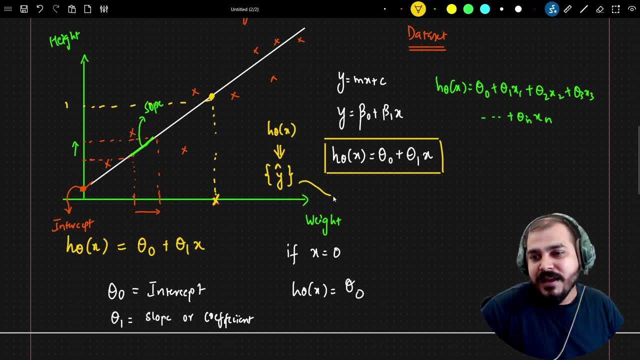 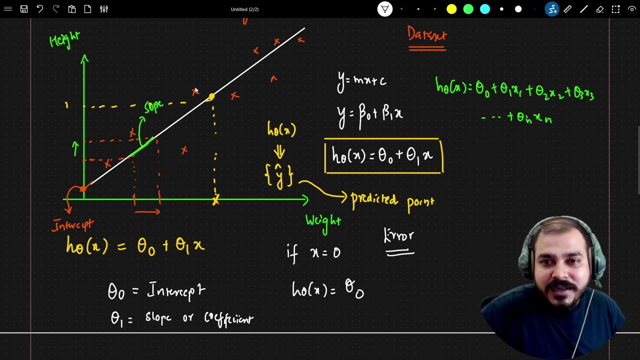 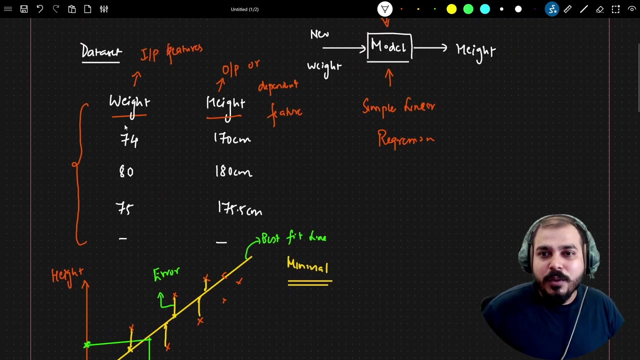 so y hat i'll be using to basically specify my predicted points. okay, predicted points, very simple. okay, now let's go and understand what exactly is error. can i say error over here is nothing, but the difference between see this orange point is nothing by y point, right, y point why i'm saying because over here in my data, right, this is my. 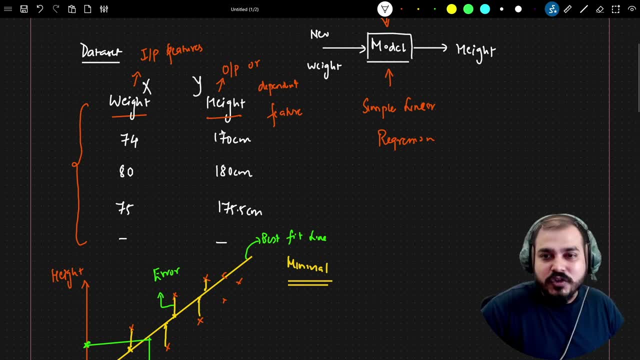 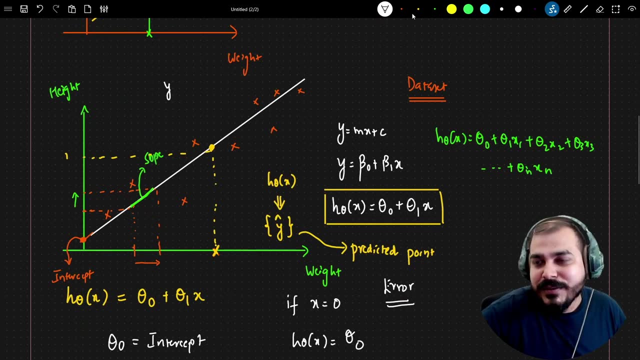 output. let's consider: this is x, this is y right. so this basically is my output right and the points that i probably get. let's say this is my y point and let's say, with respect to this, my true point is some. my predicted point is somewhere here. 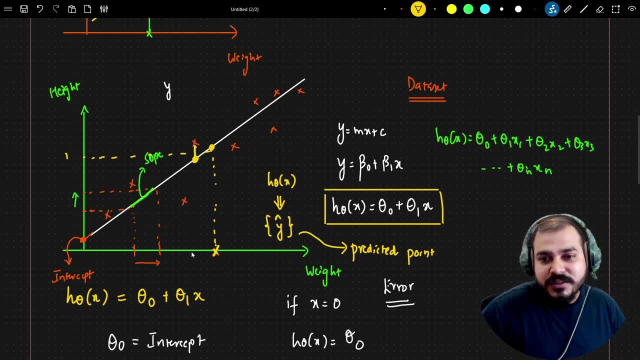 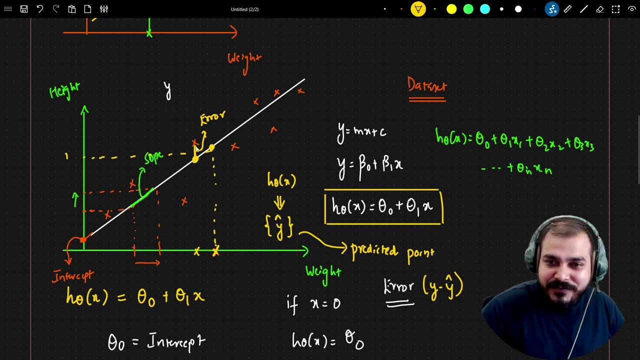 right. so if i do this difference, then, with respect to this specific data point, this should be my error, right, this should be my error. so error over here. nothing what i'm doing. i'm just subtracting y minus y hat right, y minus y hat. so, in short, i'm just trying to find out the difference between: 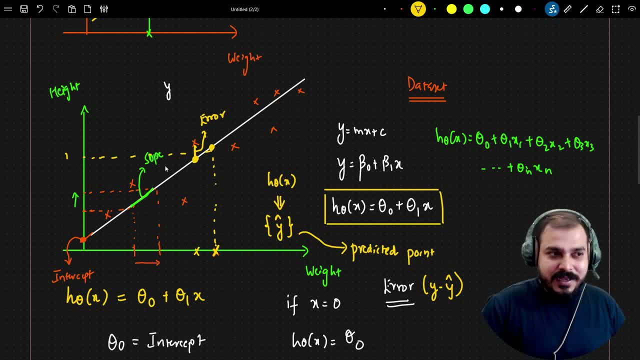 these two points, and that actually specifies my error. again, let me tell, talk about, like: what is our main aim? our main aim is to basically come up with a best fit line wherein, when i try to calculate or do the summation of all this error, it should be minimal. if it is not minimal, suppose 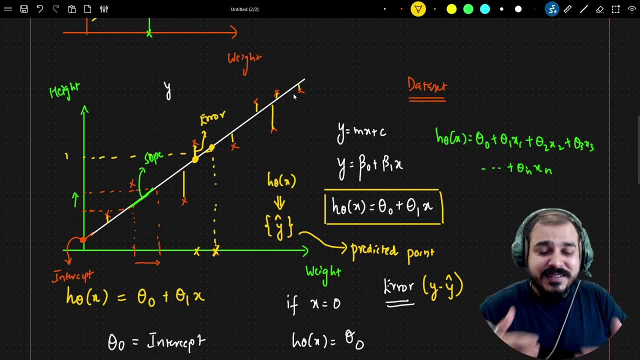 there is another best fit line that actually brings up this error or minimizes this error. i'm just going to select that specific best fit line. okay, so i hope you have got the idea about error. what's h? theta of x is why, what y hat is and what all? uh, with respect to theta zero, what is theta? 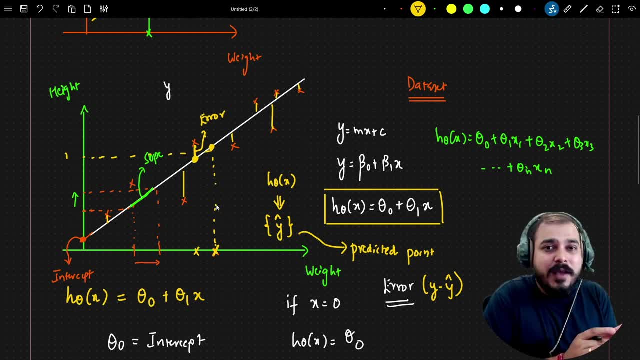 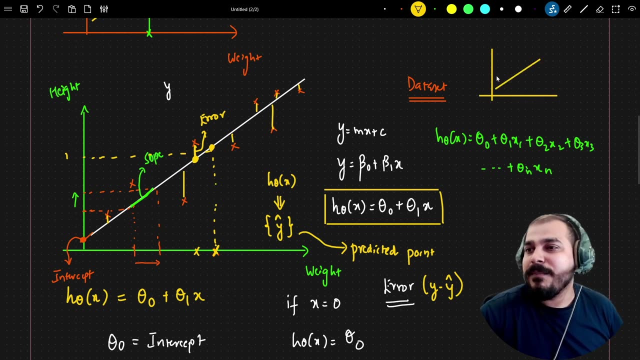 right. so this was some of the notations that you really need to know when we start learning about the simple linear regression. now, as we go ahead, we will try to understand how this best fit line is basically created, because we cannot just go ahead and randomly create many best fit line. 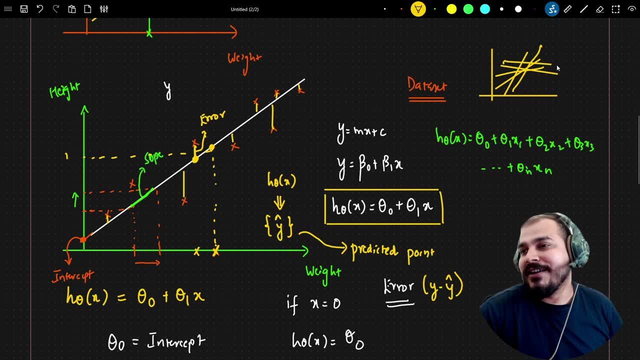 and then probably try to check each and every. you know, uh, what is the error? if, once, i do all the summation of the error, which is less, which is less, and then try to select a best fit line. no, this is not efficient. so we'll try to find out an optimized way wherein, first of all, we will try to 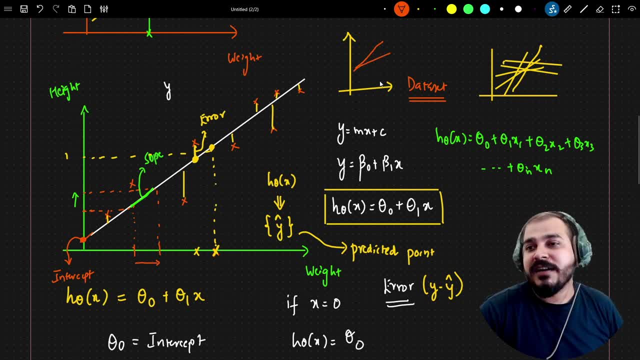 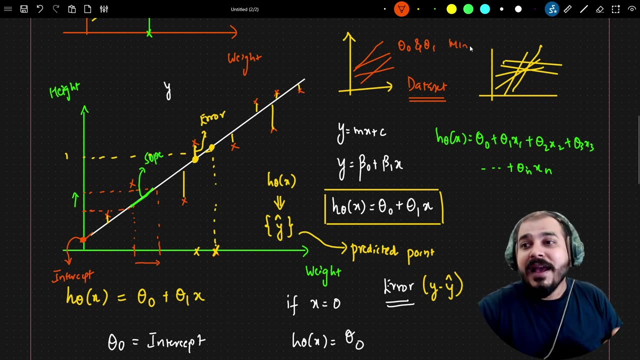 create one best fit line and then we'll try to rotate this best fit line by changing the values of intercept and coefficient. right, we are going to change this value of theta zero and theta one, theta zero and theta one, and then try to find out the best fit line with minimal error, right. 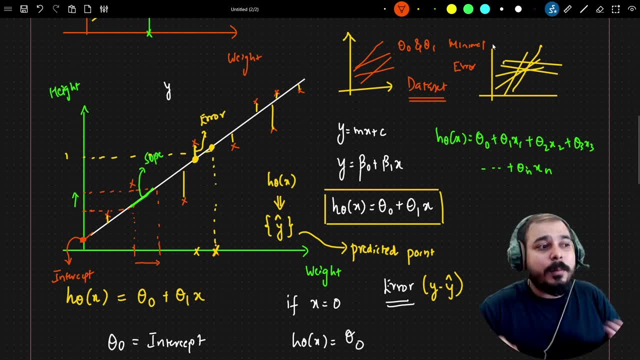 so this is what we are going to learn, and we'll try to see how this optimization technique will end and how we are going to perform all these things. so, guys, we are going to continue our discussion with respect to the simple linear regression, and in our previous video we have 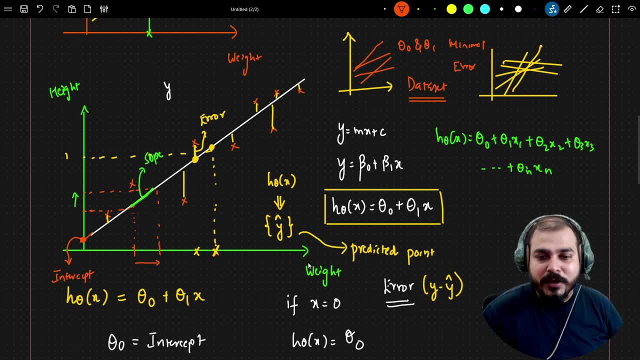 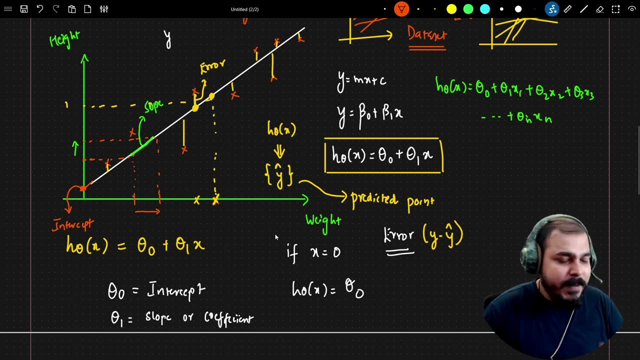 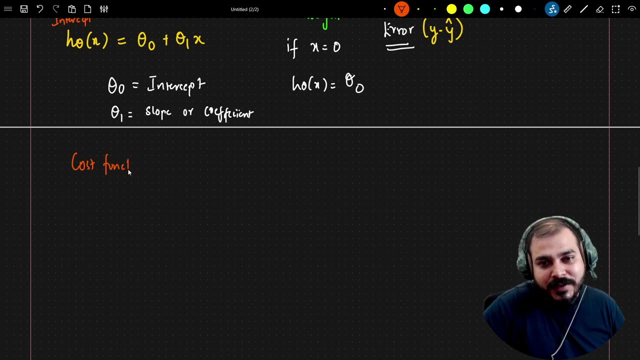 already seen what is our main aim, and we have understood about the notation and we also found out that, okay, let's try to find out an optimized way to actually get the best fit line. okay, now for this. uh, we will be using a cost function. now here i'm just going to mention about this specific cost. 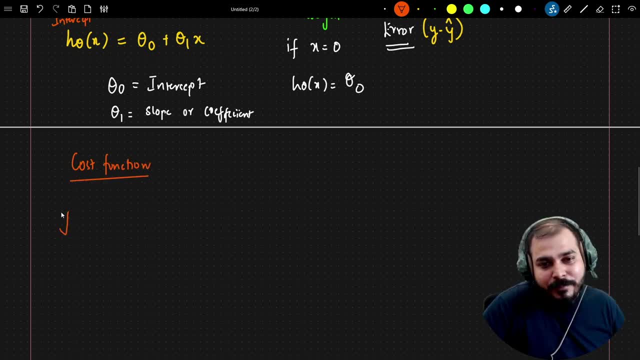 function, and this cost function is basically given by a notation. let's consider this specific notation: j, theta 0 comma. theta 1 is nothing but 1 by 2m, summation of i is equal to 1, 2 m. h theta of x of i minus y of i, whole square. 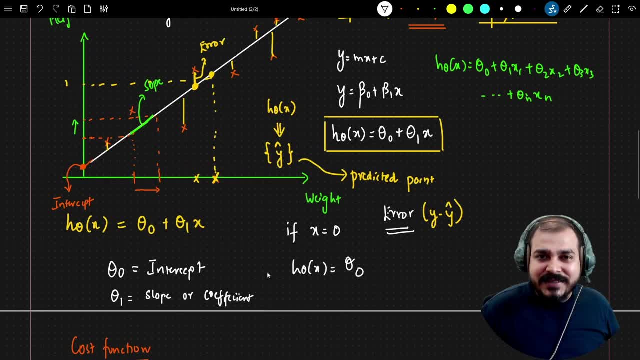 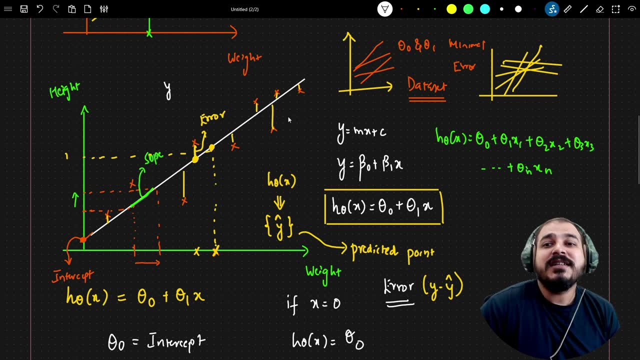 now what is h theta of x of i minus y of i whole square? as i said that we have to make sure that we have to create a best fit line in such a way that when we are going to create the best fit line, we do the summation of all these specific errors. it should be minimal. so that is the reason we are. 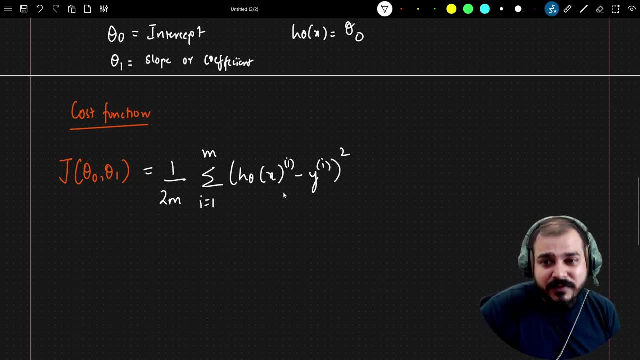 taking up this cost function in this specific way. h theta of x of i is nothing, but these are my predicted points. right, these are my predicted points and these are my truth points. so, basically, the true output- right, and i'm going to do the summation- means basically, do this: uh, when we do, 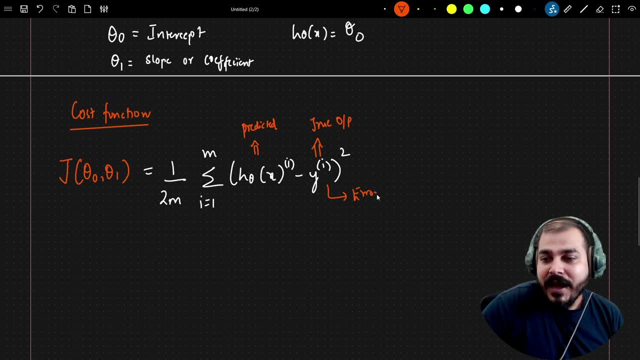 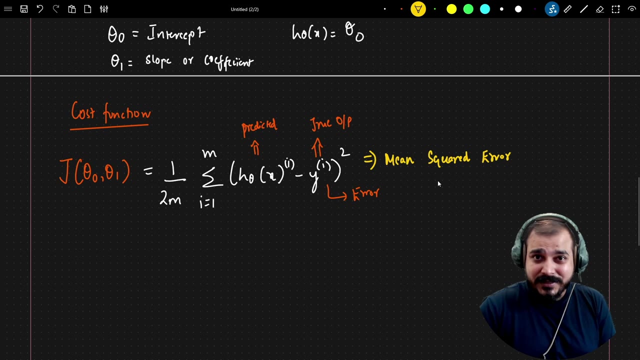 the subtraction, we basically get the error value and the reason we are squaring it because, uh, the the cost function that we are using this. we basically say this cost function as mean squared error, okay, mean squared error. and there are a lot of advantages of using mean squared error, which we will probably discuss as we go ahead. now you may be thinking krish. 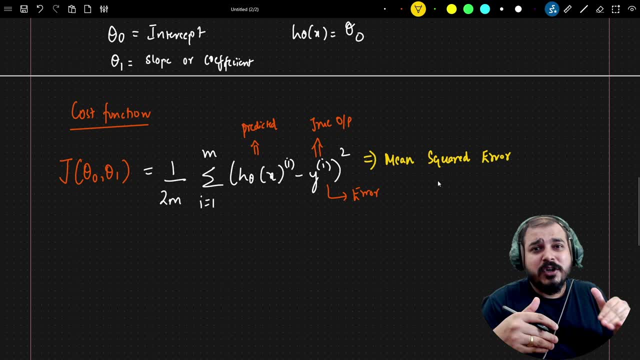 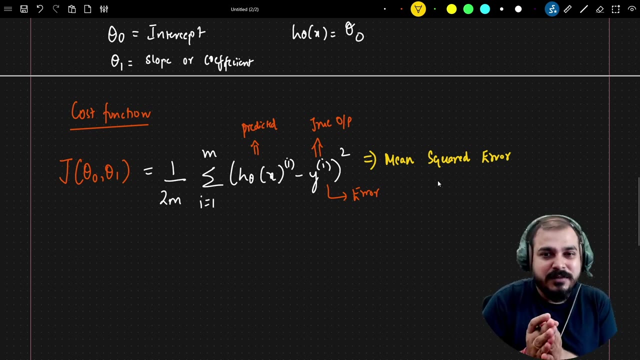 is there different kind of cost function also used? yes, absolutely. you also have something called as mean absolute error root, mean squared error. we will all try to discuss about all this kind of cost function and what is the advantage and disadvantage with an aspect to that. okay, but here right now, the reason i'm taking up this cost function, because we really 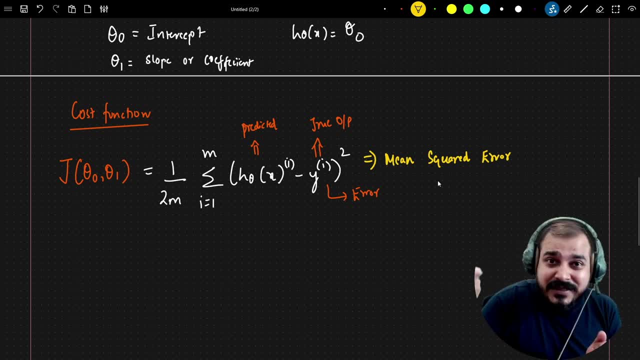 need to minimize this cost function, and we need to minimize in such a way by changing the theta zero and theta one value. theta zero basically tells us about the intercept and theta one basically talks about the slope. okay, so what is our final aim? i'm just going to write out. 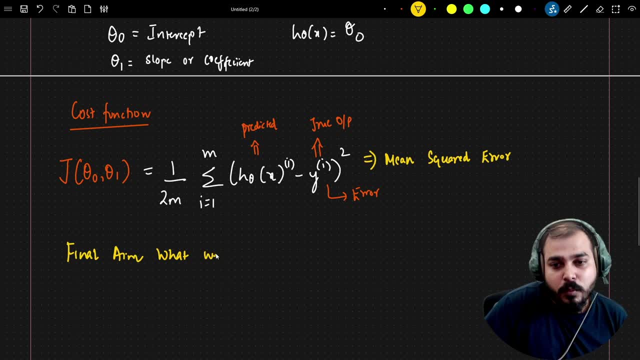 finally, what we need to solve, okay, what we need to solve. okay, what we need to solve, me solution, bounding mu, bounding, looping, loop along, swearing Сейчас, so so that we get delta. i super Ergebnis Castaki's Fул 인. now, what i want to do is: we want to use this cost function. okay, there's super economy and 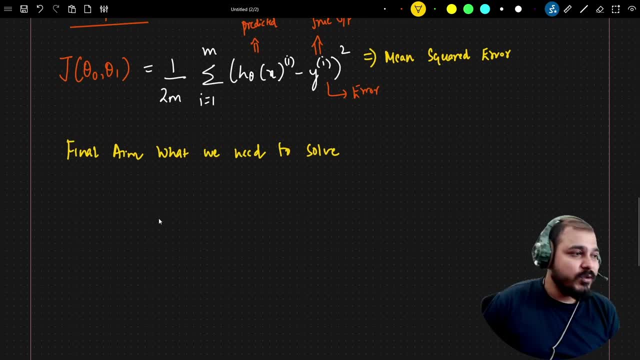 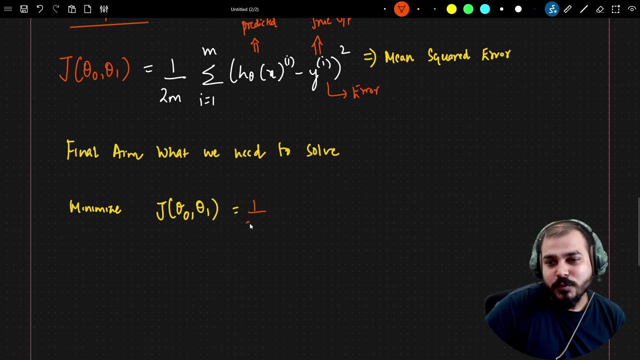 This is super important. Then, only here, I basically use the cost function. So our main aim is basically to minimize the cost function. j, theta 0, theta 1, which is basically denoted by this specific equation, That is, 1 by 2m. summation of i is equal to 1 to m. h theta of x of i minus y of i. okay, whole square. 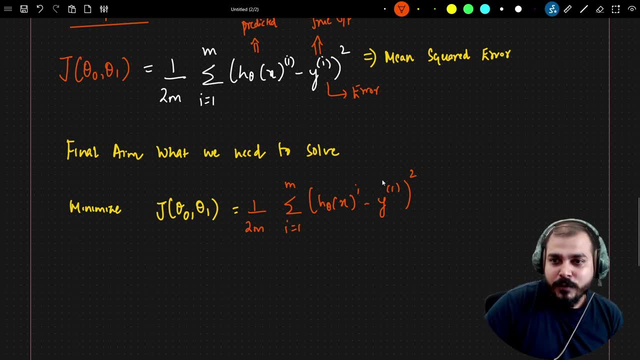 Okay, since we are dividing by m, so we are getting this as mean right mean squared error. We basically say this cost function as mean squared error And how we are going to minimize this by changing the value of theta 0 and theta 1.. 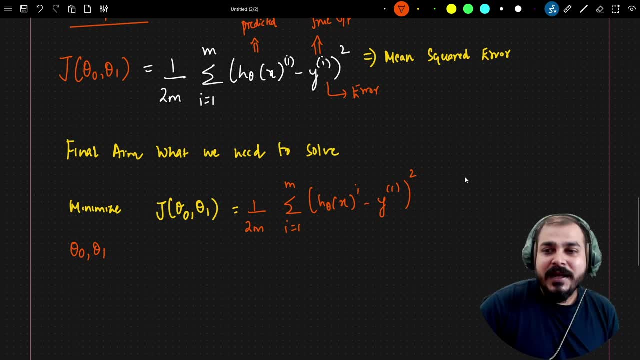 So we really need to continuously change this theta 0 and theta 1 and try to find out the best fit line wherein we do the summation of this particular error, And this should be minimal, okay, minimal as possible, Okay. so this is what is our final aim, that we are. 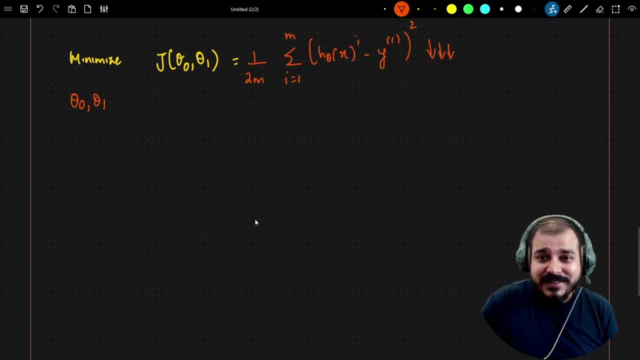 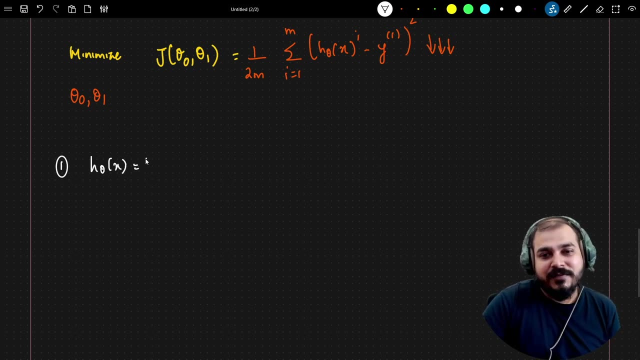 Looking at okay, and how we are going to do this. Let's try to discuss about it Now. I hope everybody knows what is the equation of my straight line. This is nothing but h, theta of x, theta 0 plus theta 1 into x. 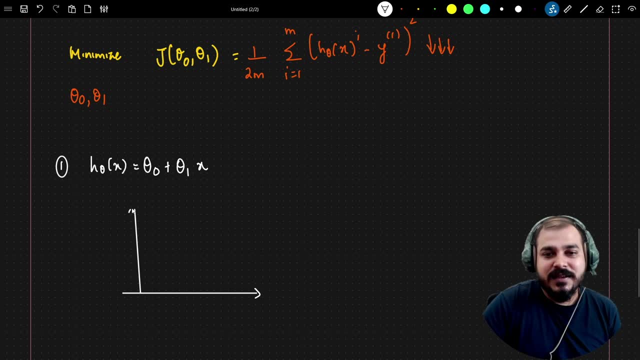 So that basically means, if I probably consider this okay, the best fit line, whatever straight line I'm actually getting, Let's consider that I'm getting this specific straight fit line, So this line is basically indicated by this equation. Now one important thing. 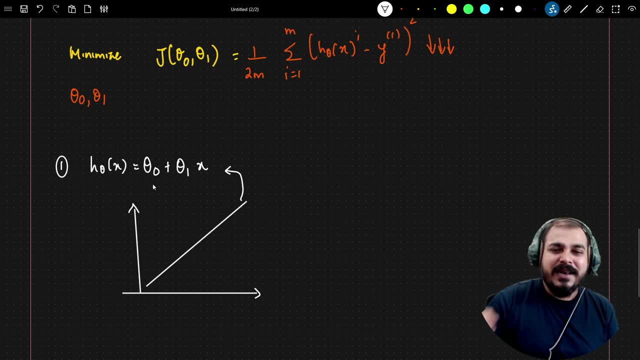 Since there are two variables like theta 0 and theta 1, let's consider that theta 0 is 0.. Okay, let's consider. there is a reason why I'm saying because I really wanted to show you everything by drawing it in a 2D diagram. 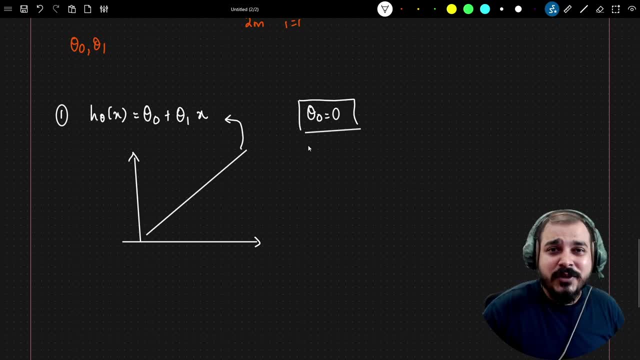 So let's consider theta 0 is equal to 0. If I say theta 0 is equal to 0, that basically means when my x value is 0, it is basically passing through the origin, right? This line is basically passing through the origin. 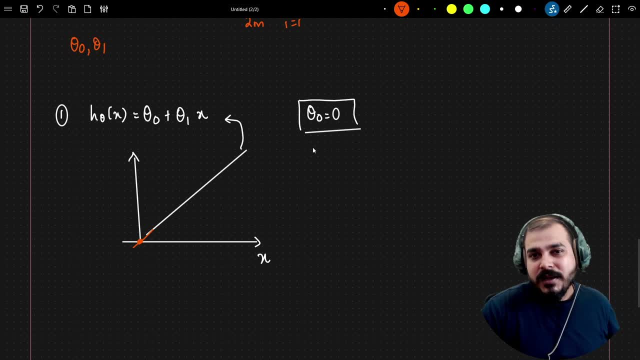 So this intercept Is exactly 0.. Okay, so now my equation becomes: h, theta of x is equal to theta 1 multiplied by x. Let's consider that. what I'm doing over here, My intercept, is basically passing through the origin. I'm just considering it so that I can draw a cool 2D diagram to make you understand more in depth. 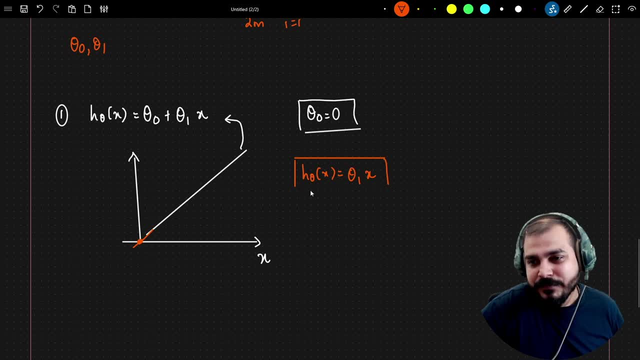 So currently I'm going to just use this specific equation. Okay, now let's consider some of the data points. Let's say this is my x and y. I'm just going to write 1.. 1, 2, 2 and 3, 3.. 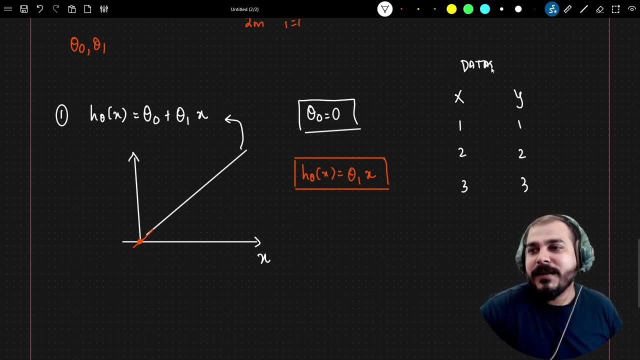 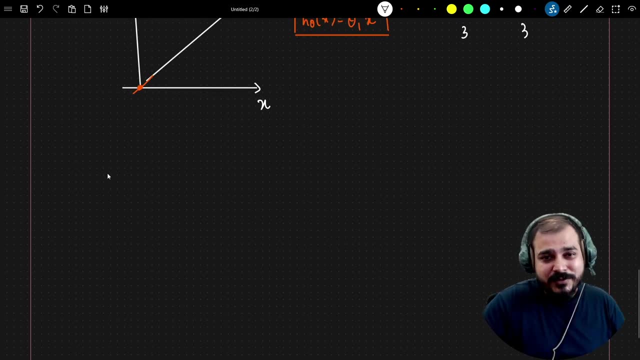 Okay, let's consider that this is my entire data set And for this particular data set, I really need to create a best fit line, Because this will give you a clear idea that what we are trying to do, So what we will do. we will just try to create this line like this: 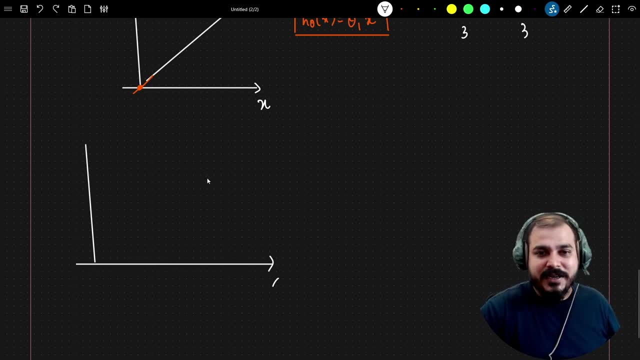 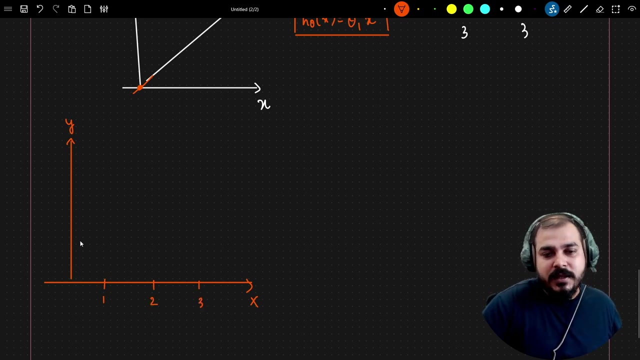 Okay, this is my x, This is my y, So let me create it a little bit straight so that it looks cooler and good. So this is my x and this is my. this is my x And this is my y. Let's say, these are my values, like 1,, 2,, 3.. 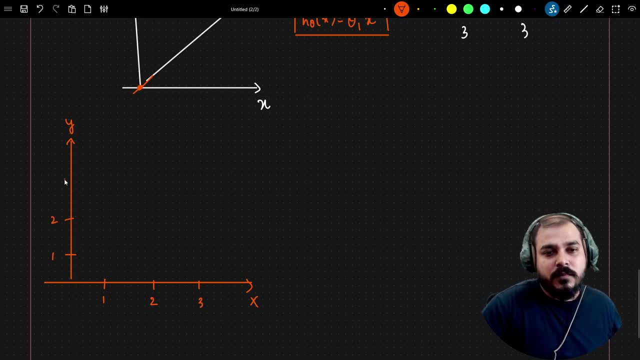 And with respect to x, y also. I have 1,, 2 and 3.. Okay, now let's start. Okay, and obviously everybody knows what is the equation. It is nothing, but htheta of x is equal to theta 1 multiplied by x. 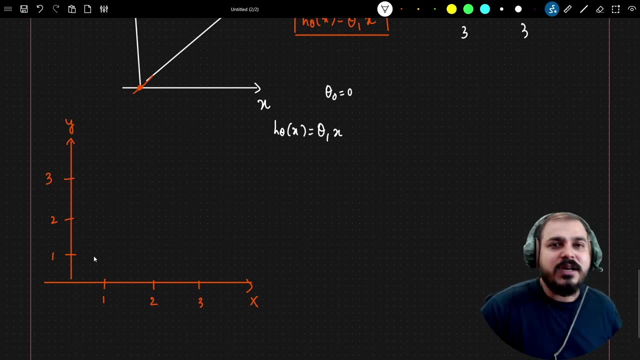 Why? Because theta 0 is equal to 0. because we are considering it passes through the origin. Okay, so I have my data points. My data points are 1, 1., 2, 2.. 3, 3.. 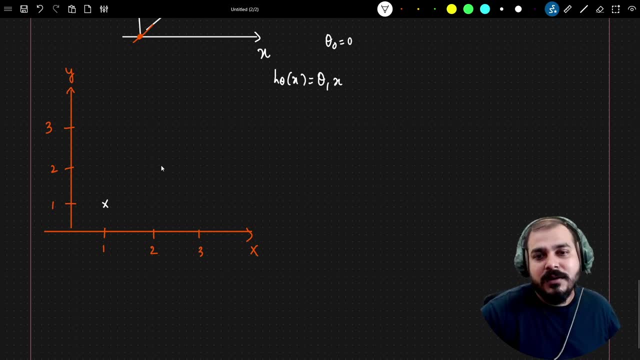 So let's go ahead and plot it. Okay, so here is 1, 1.. Then this is 2, 2.. And this is basically 3, 3.. Okay, now, if I have this particular data points, I am going to use this equation of a straight line to make sure that I plot my best straight line. 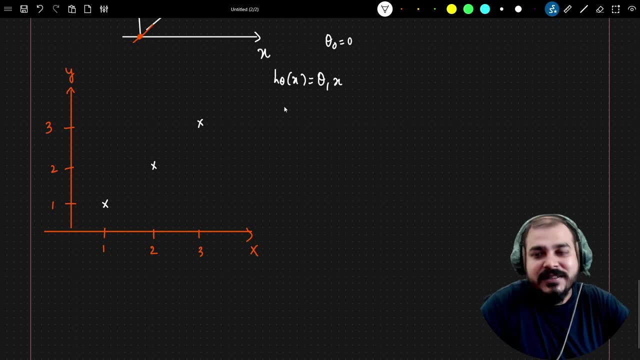 Okay, now let's consider we need to initialize theta 1, right with something. So let's consider let theta 1 is equal to 1, because this is my slope Right And we have to initialize. We have to initialize the slope and later on we will keep on changing the slope to get the different, different, best straight line. 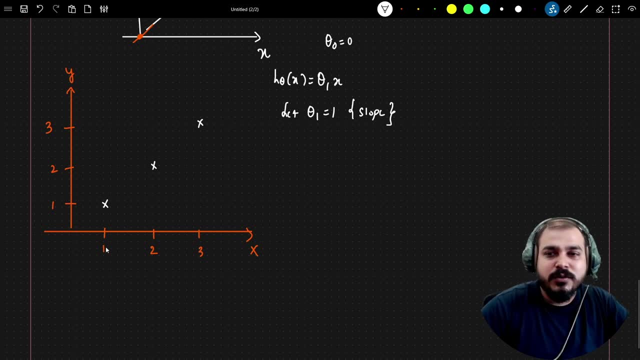 So if theta 1 is equal to 1, then when x is 1,, what will be my htheta of x? So my htheta of x will be actually 1 when my x is equal to 1.. Right, I hope this is very much clear. 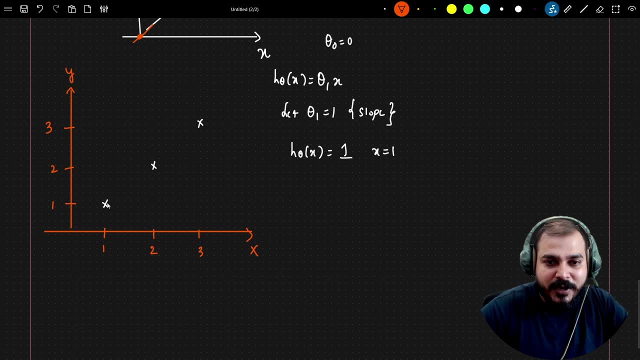 Right, So let me just put this points Then. this will be basically my predicted points over here with respect to htheta of x. Now, when x is equal to 2.. What will be my theta htheta of x? htheta of x will be, since I have initialized theta 1 as 1, when x is equal to 2, that basically means htheta of x will be 2.. 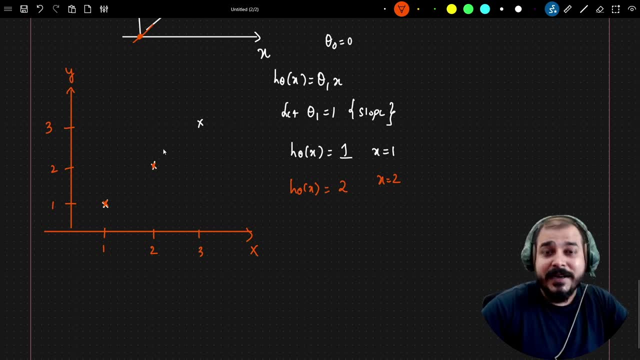 So my second point will be somewhere here. Right, The predicted point, htheta of x. Okay, And similarly, when my x is equal to 3, when theta 1 is equal to 1, that is, my slope is equal to 1, then htheta of x is equal to 3, because 3 multiplied by 1 is nothing but 3.. 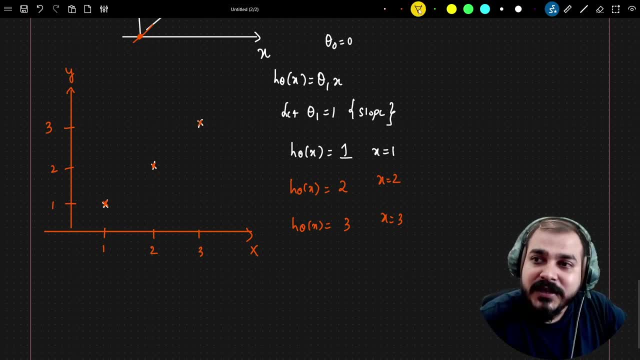 So my third point is somewhere here Now, if I try to create a best fit line. So this is going to pass through all these points, Right, All these points. So it is going to exactly pass through all these points And obviously it will also pass through the origin. 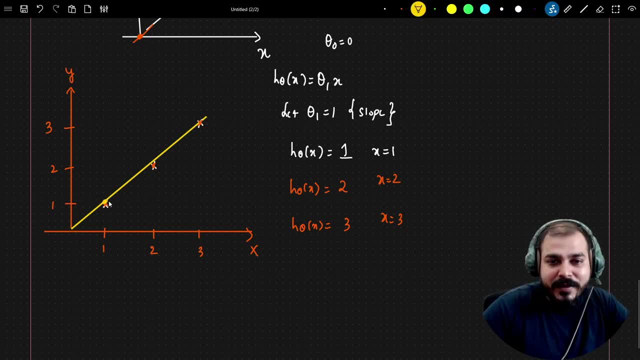 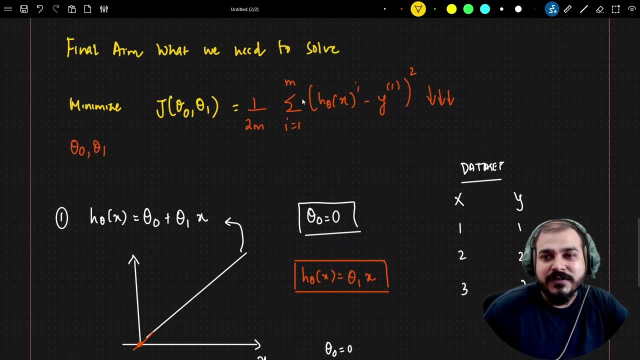 Okay, So in short, these are my predicted points, And over here I also have my truth points. Right, I also have my truth points. Now let's go ahead and apply this cost function j of theta, theta 1.. 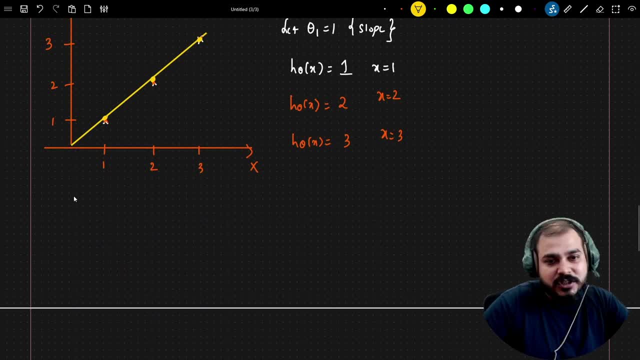 This is this entire equation. So what is my cost function over here? My cost function is very simple. I will write j theta 1, because theta 0 is 0.. Right, It is passing through the origin, So I will write 1 by 2m. summation of i is equal to 1 to m. 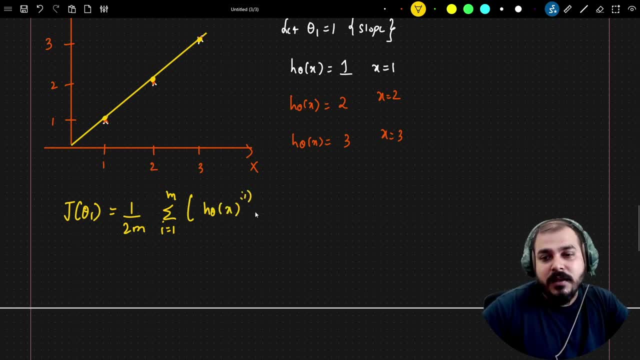 And here I will basically say: htheta of x of i minus y of i, whole square Right. So how many points I have totally? I have three points Right In my data set. I have three points: 1, 2, 3.. 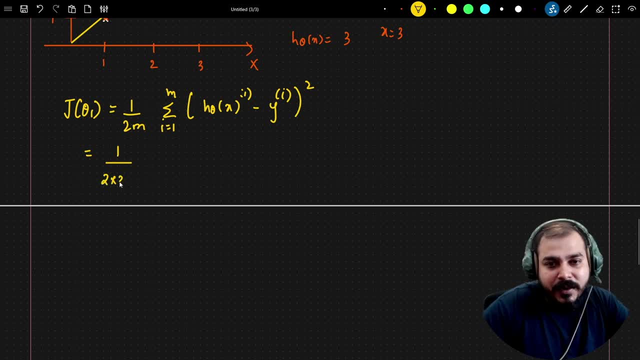 So I'm just going to basically write 1 by 2 multiplied by 3.. And I'm just going to basically say: summation of i is equal to 1, 2, 3.. Okay, So it will be the entire summation of 1, 2, 3.. 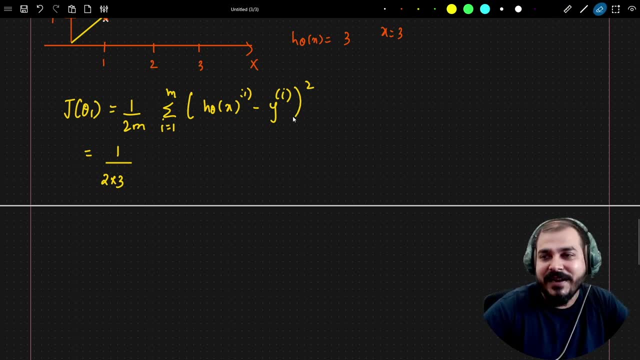 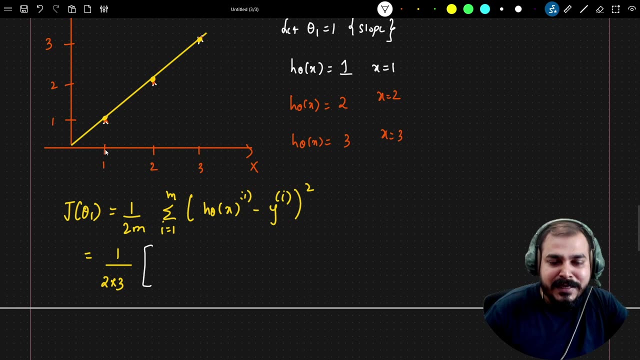 Right, So no need to write 1,, 2,, 3.. So I will start expanding this. So first thing is what? What is htheta of x of i when i is equal to 1?? So over here you can see, when i is equal to 1, htheta of x of i, the predicted point is also 1.. 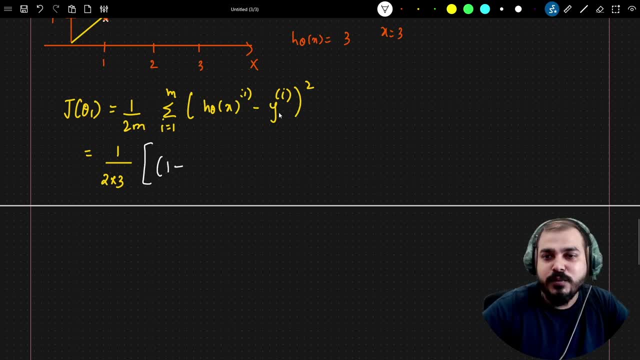 Right. So I'm just going to basically write 1 minus what is y of i at that point of time? So y of i is also 1.. And here also we have plotted it. So 1 minus 1 whole square. 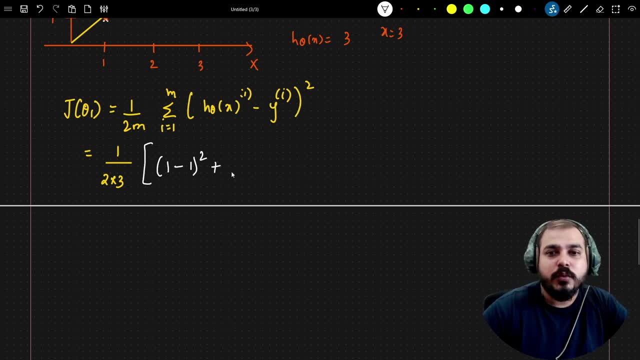 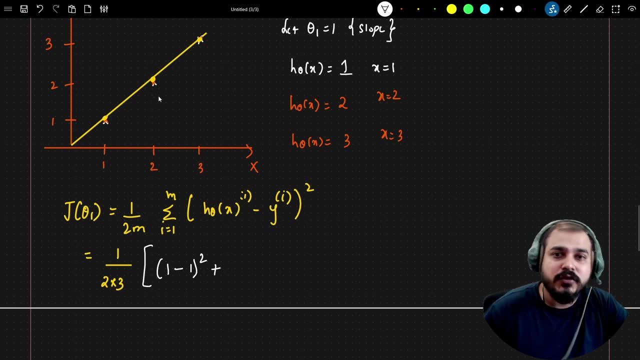 Okay, Then plus we'll go to: i is equal to 2.. i is equal to 2.. Over here you can see: when the x value is 2, htheta of x of i is also 2.. And y is also 2.. 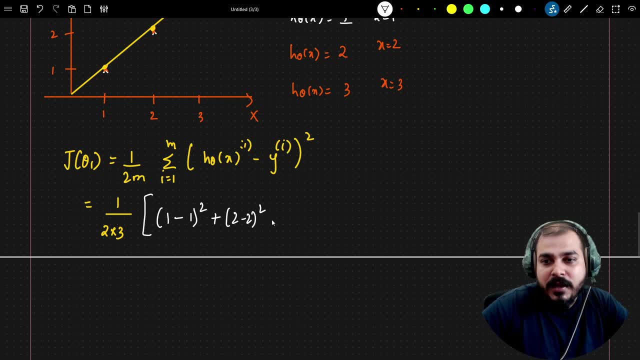 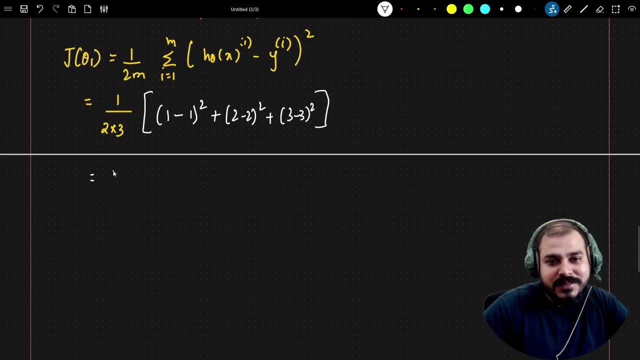 Right, So over here I'm going to write 2 minus 2 whole square, And similarly, this is 3 minus 3 whole square. Okay, So overall, if I try to find out, it is 0.. So what does this basically indicate? 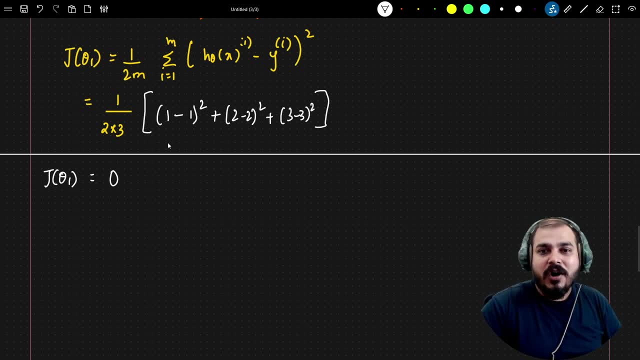 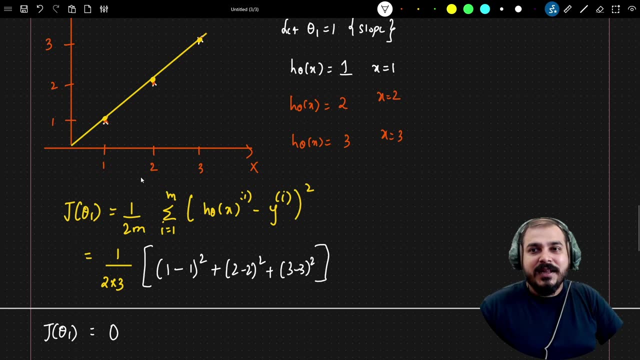 My cost function is 0.. This is absolutely right. Right, Obviously, there is no error. Exactly The best fit line passes through all the points Right Now. this is one way. Okay, Now let's go ahead and consider and let's change our theta 1 value. 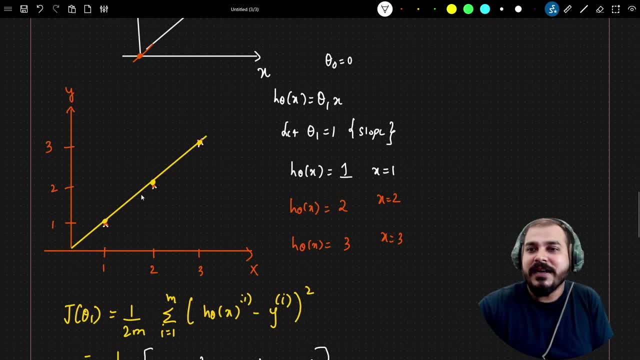 Let's say that our theta 1 value is. now let's consider that our theta 1 value, Let's say our theta 1 value is 0.5.. Now, if it is 0.5, then what will be htheta of x when, if x is equal to 1?? 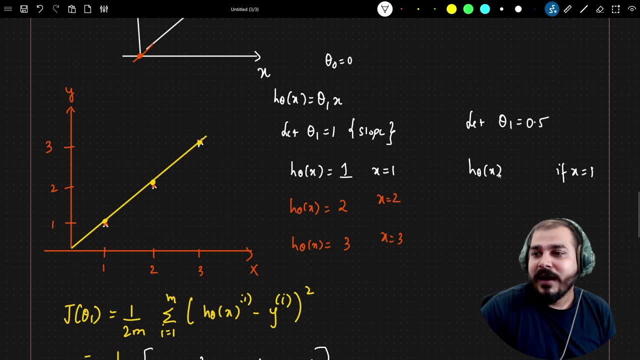 So it will be nothing but theta 1 is 0.5.. 0.5 multiplied by 1.. Right, So this is going to be 0.5.. 0.5.. Right, So, when x is 1, so my htheta of x will be 0.5.. 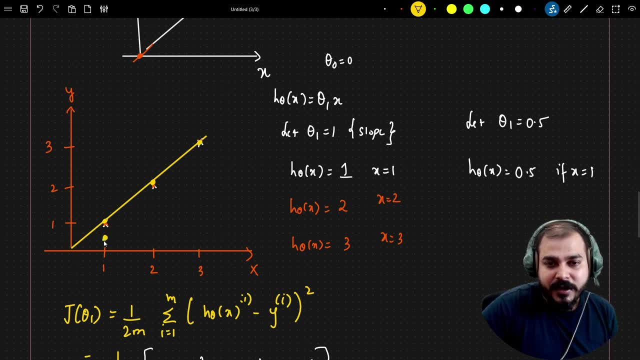 So let me just denote this particular point. over here It is 0.5.. Okay, Now, similarly, when theta 1 is 0. And if x is equal to 2, then here you will be seeing, htheta of x will be 1.. 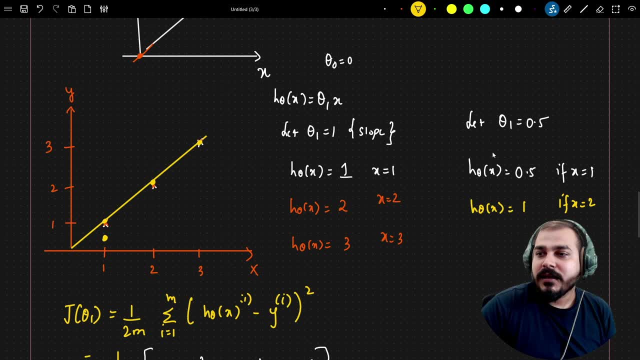 Because here we are just multiplying theta 1.. Theta 1 is nothing but 1.. Okay, 1 multiplied by 2.. Sorry, 1 multiplied by sorry, theta 1 is 0.5.. So in this equation, htheta of x. 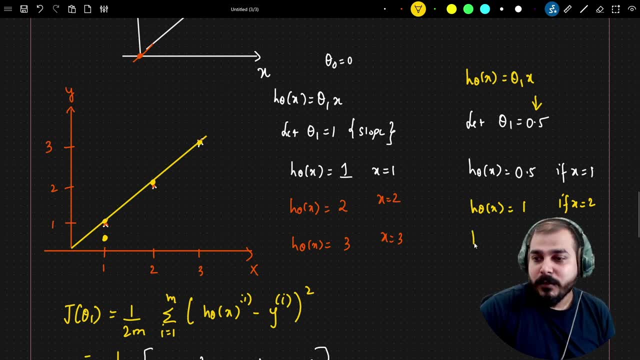 Theta 1, x, Right 0.5 multiplied by 2 is nothing but 1.. Then htheta of x is equal to. when x is equal to 3, this is going to be 1.5.. Okay, So when your x is 2, I'm actually getting 1.. 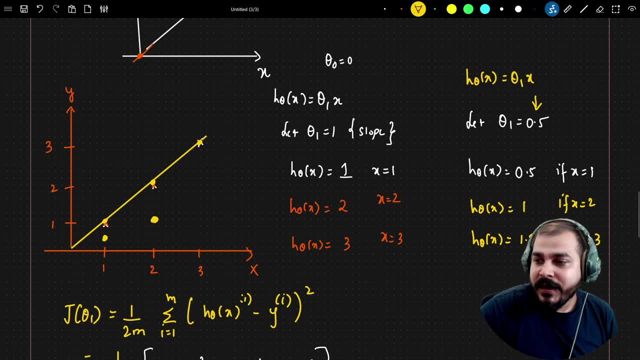 So I'm going to basically note this particular point. And when x is equal to 3, htheta of x is nothing but 1.5, which is basically mentioned at this particular point. Okay, Now, here you will be able to see that I'm just going to draw this next best-factor point. 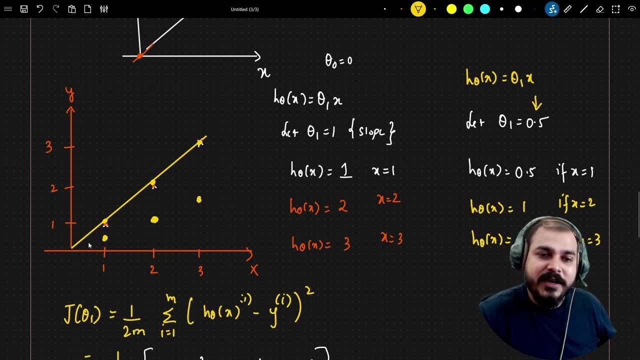 So I'll, I'll make it a little bit better so that the point is basically drawn. So this is my best-fit line for the next one Again, sorry. So 3, 5.. Okay, Now, this time I should be getting a best-fit line. 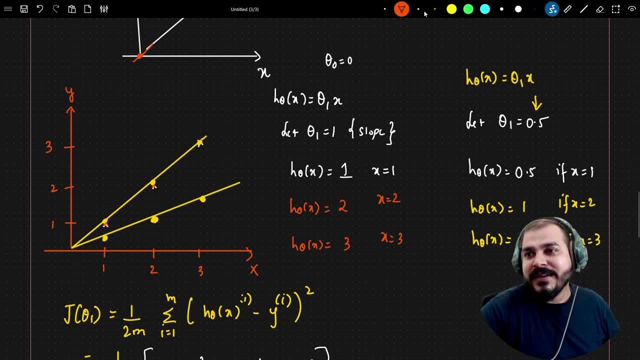 Okay, So this is my best-fit line. Okay, Now, here you should be able to understand that these are my predicted points. This, this, this are my predicted points. Okay, Now, with respect to this again, let's go ahead and calculate jtheta. 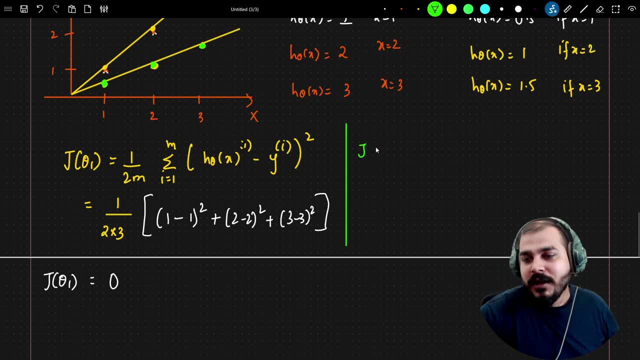 Okay, jtheta Of one. So here I'm basically going to write what is jtheta of one. jtheta of one is nothing but one by two. M again, I'll apply the same formula. So this will be one multiplied by two, one divided by two, by three. 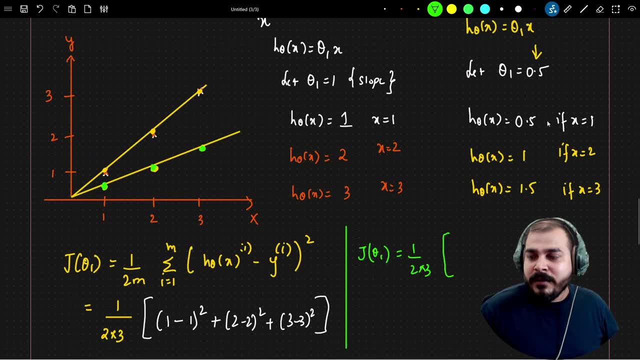 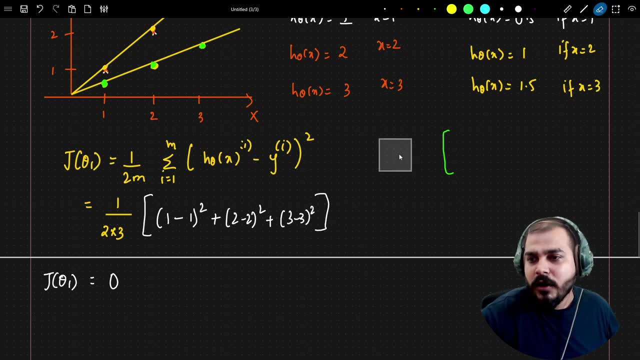 And now let's go ahead and try to find out. So, when my theta one is 0.5, let me do write it, Let me write it down below, Okay, So that you will not miss anything. Okay, So the first case, uh, uh. 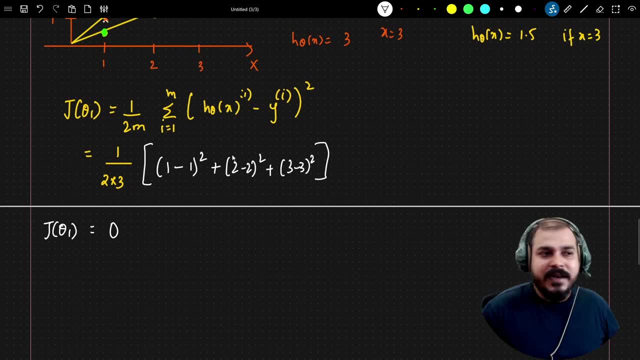 let's consider- I have also drawn this specific point and, uh, let me draw one more, uh amazing graph, Okay, And this graph will be mentioning something very important, So let's create one more graph over here and we will continue. 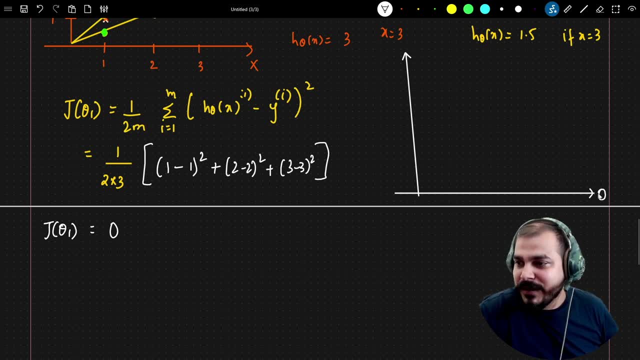 We'll continue with respect to different, different values. This graph is between theta, theta one and j of theta one. Okay, And let me denote it. some points like this: 0.5.. This is basically One, 1.5, 2.0,, 2.5, right. 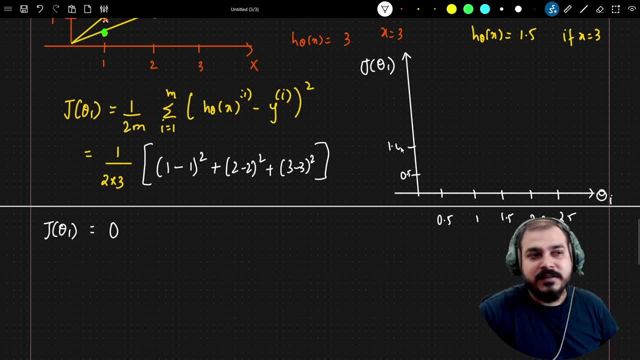 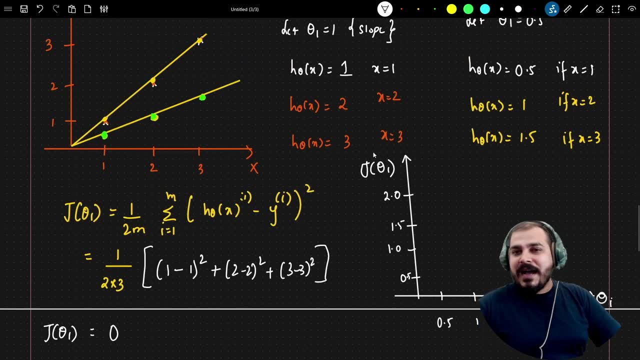 And similarly, this is 0.5, 1.0.. Okay, And this is 1.5 and this is 2.0. Okay, So this points. I'm just creating, along with this, a different graph over here. 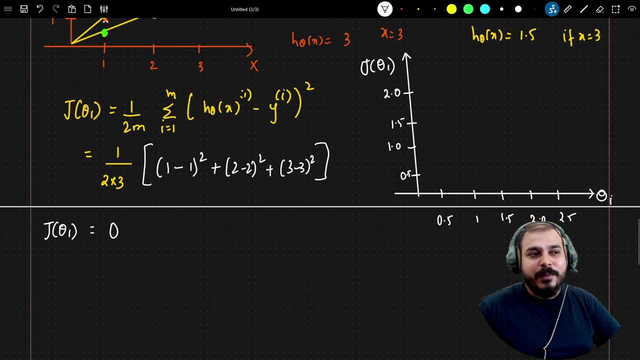 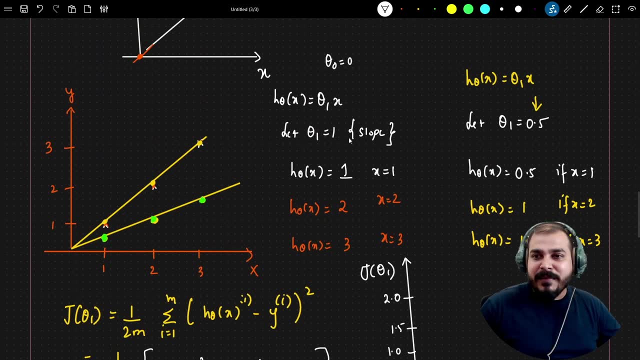 And this graph basically indicates: uh, the graph between uh theta one and j of theta one, the relationship between theta one and j of theta one. Now, in the first case, when my Theta one was one, what was my j of theta one in this particular case? 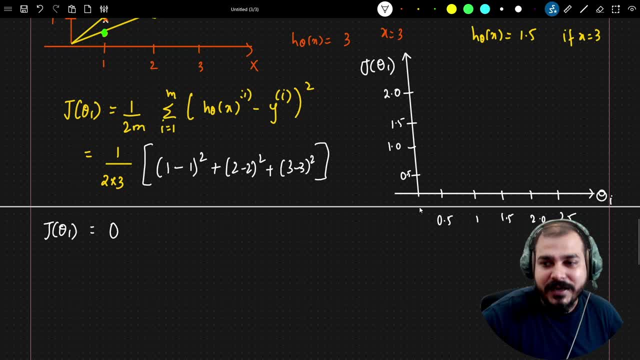 It is zero. So I am just going to basically plot this particular point. Okay, When my theta one was one- and here you can basically see- my j of theta was zero, So can I plot this particular point somewhere here? So I'm plotting it somewhere here. 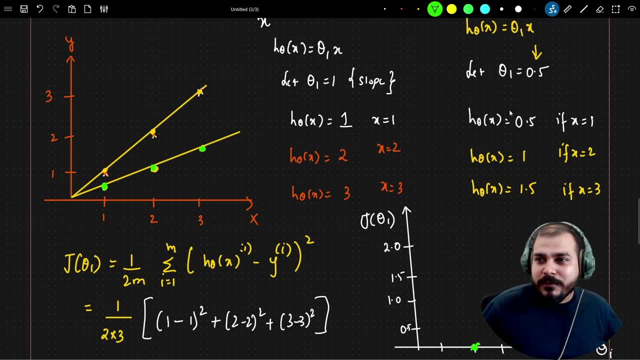 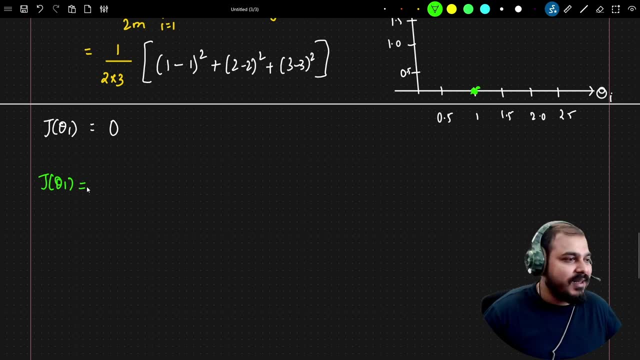 Okay, So this is my first point that I've got now with respect to theta one is 0.5.. Let's go and compute my j of theta one. So j of theta one is nothing, but I will start writing it down over here. 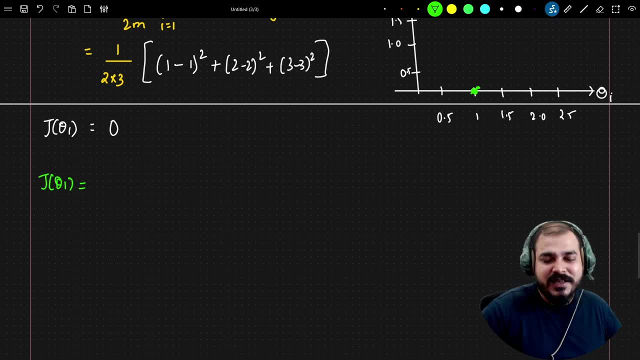 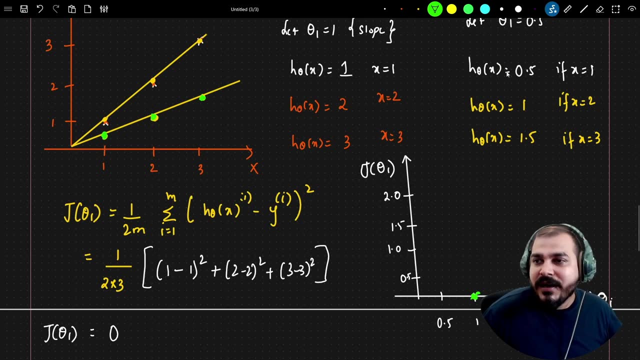 And you also make sure that you write this particular equation very much easily. So it will be nothing but one by two multiplied by three. And the first case: what is h theta of x when theta one is 0.5.. So over here you can see when, if x is equal to one, 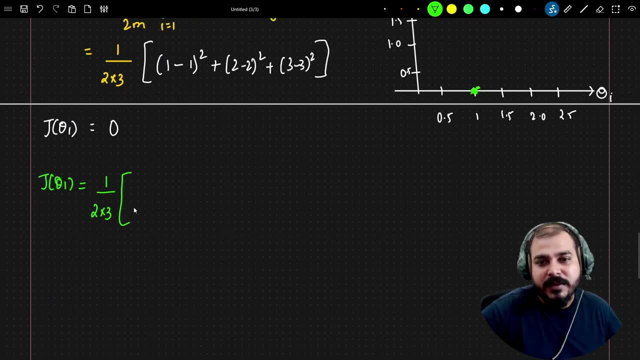 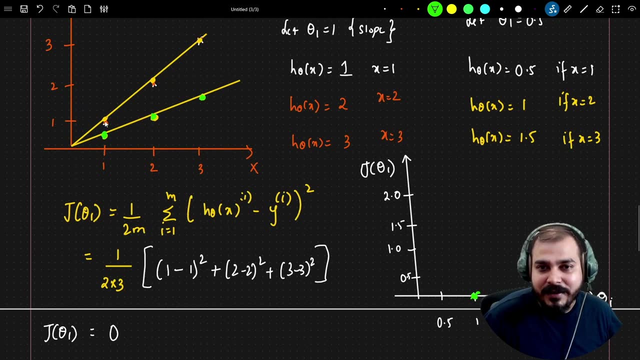 So here you can see that h theta of x is 0.5.. So here I'm going to subtract, write 0.5 minus one whole square. Okay, One how I'm getting my true value. one is over here, right. 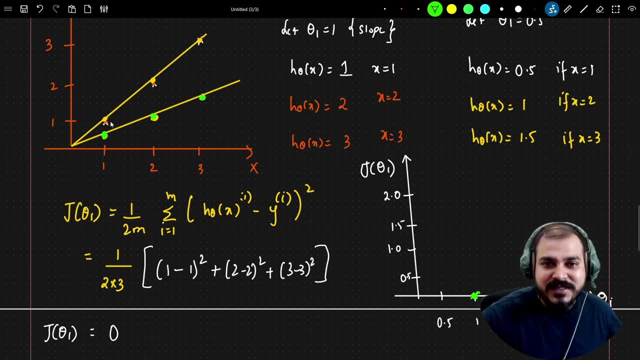 Still, my real point is over here. So 0.5 minus one. So this is the error that I'm actually getting right. Similarly, this is the error I'll be getting here, And this is the error that I'll be getting here. 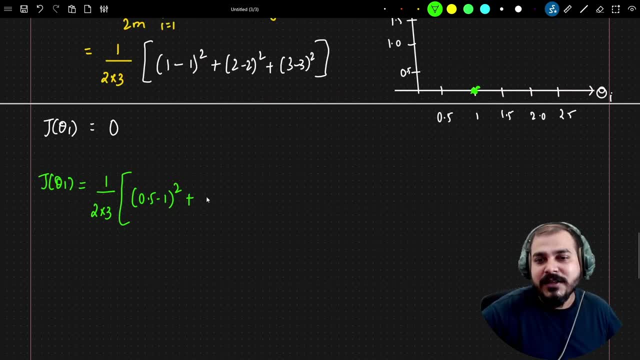 And we really need to write that specific error. So 0.5 minus one whole square, Then I have one minus two whole square plus 1.5 minus three whole square. So once I try to find it out, so this will be when my theta one is equal to 0.5, right. 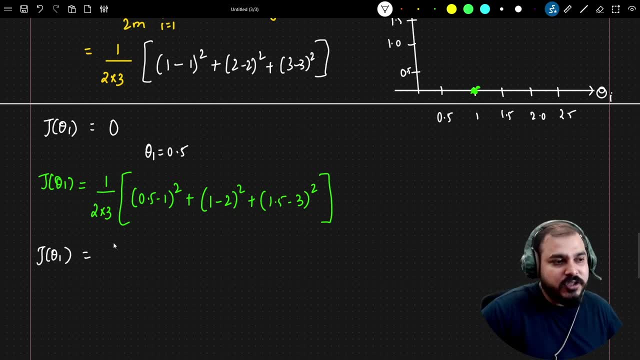 When my theta one is equal to 0.5, the j of theta one. just try to compute it, You will approximately be getting something Somewhere around 0.58.. Okay, Once you do the calculation, So over here, my, my theta one is 0.5. 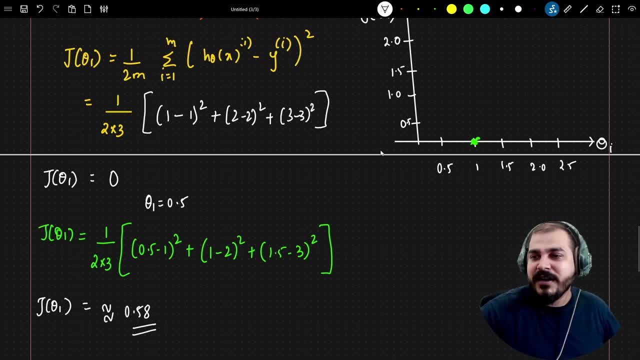 I'm just going to get j theta one as 0.58.. So 0.58 will come somewhere here. So I'm just going to make this point somewhere here, Okay, Not here, Sorry. Uh, somewhere here, with respect to theta one is 0.5. 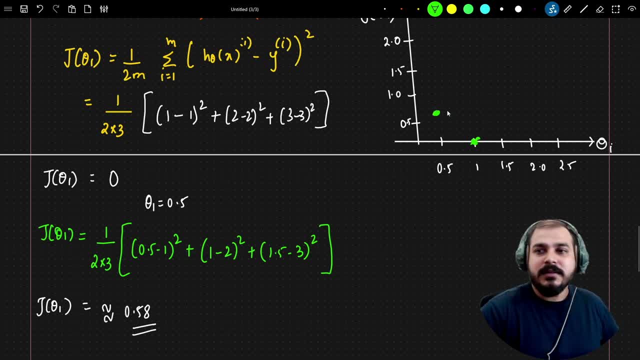 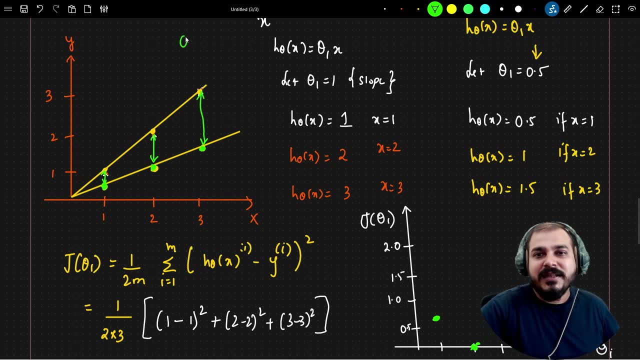 I'm going to get the point somewhere here. Okay, And this is that Okay. Now let me consider one more thing. Let's consider what will happen if I consider my theta one is equal to zero. If I consider theta one is equal to zero, that basically means when X is equal to one. that basically means what? 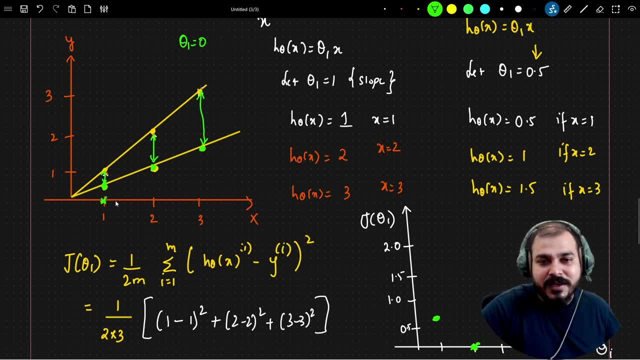 Theta one is zero. Zero multiplied by one will be zero. So my first point will be here, My second point will be here, My third point will be here, right, So this will basically be my next best fit line, And obviously the error will still be higher. 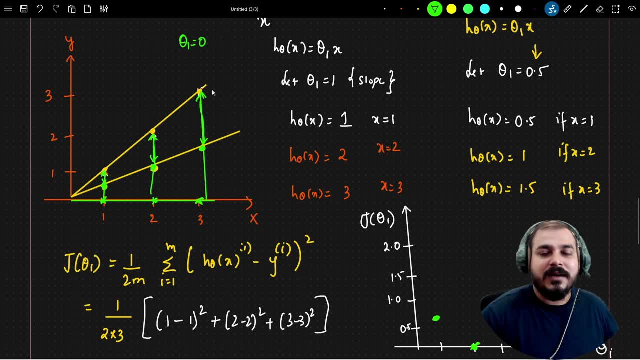 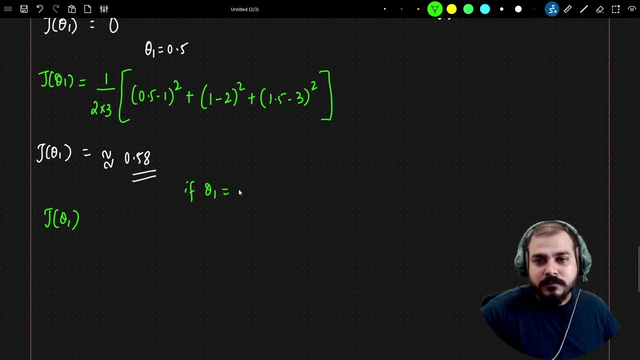 Then obviously I consider that when I probably try to calculate j of theta one, J of theta one, If my theta one is equal to zero, in this particular case, what will happen? J of theta one. Just try to compute it. Uh, it will be very simple. 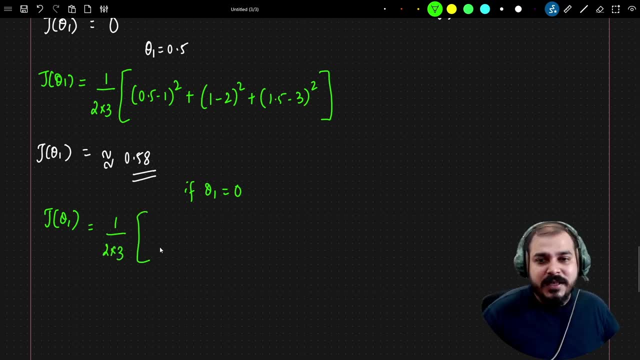 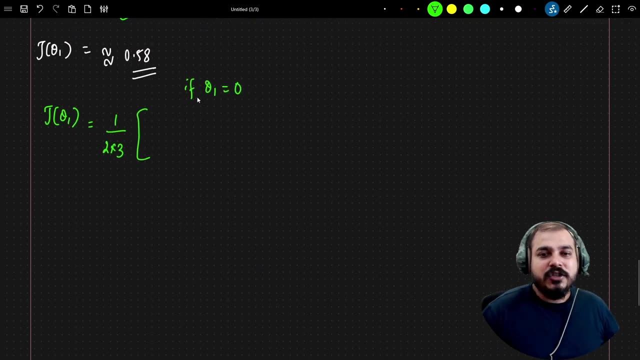 Uh, here I will write one divided by two, by two multiplied by three, and theta one is: first zero, zero minus one whole square, then zero minus two whole square, then zero minus three whole square, Right, So I'm just going to write like this: zero minus one whole square plus zero minus two whole square, plus zero minus two whole square. 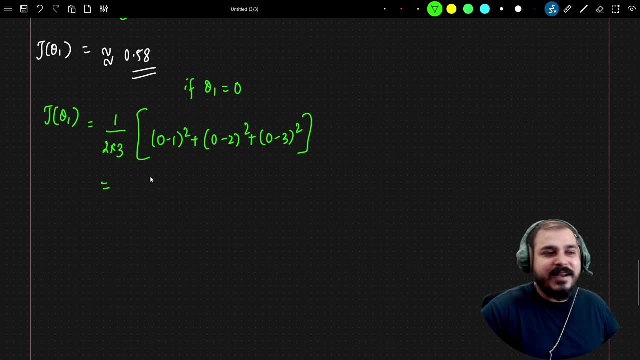 Right, 0 minus 3, whole square. Now obviously this is not the best fit line. Obviously I am going to get my error quite high, So it will be somewhere around 2.3.. So j theta 1 when theta 1 is equal. 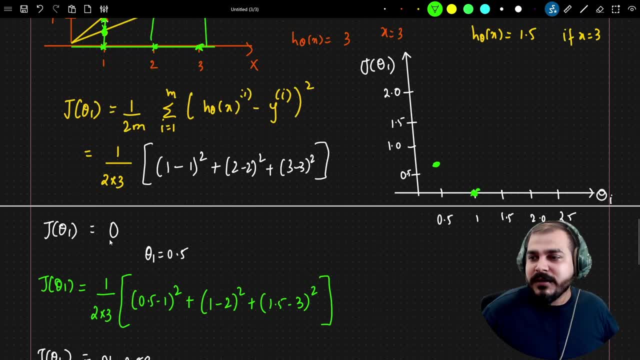 to 0, it is nothing but 2.3.. Now here, if I try to plot this, when my theta 1 is 0 and I am getting somewhere around 2.3, which is somewhere over here, right at this particular point. Now, if I keep on, 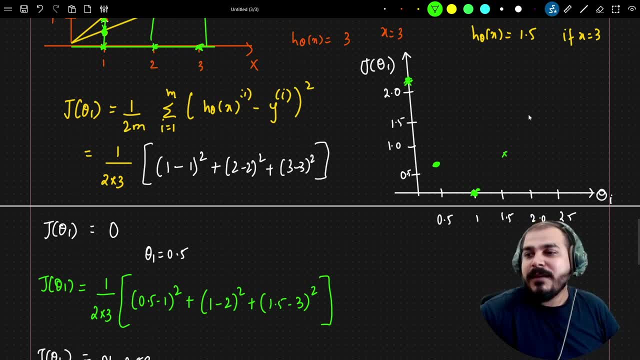 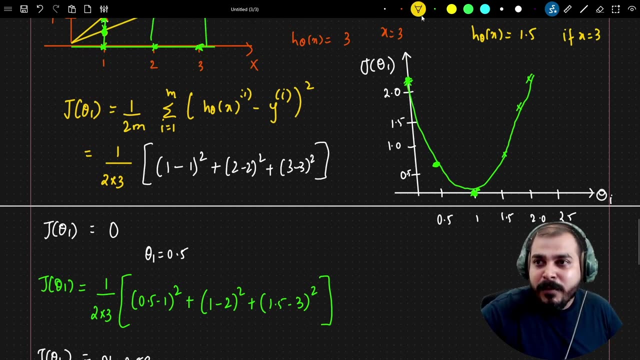 continuing doing with different, different theta 1 value. after some points you will be seeing that I will be getting this kind of curve, okay, this kind of curve, and always remember when we are trying to get this kind of curve. okay, the main point that I got over here at this particular 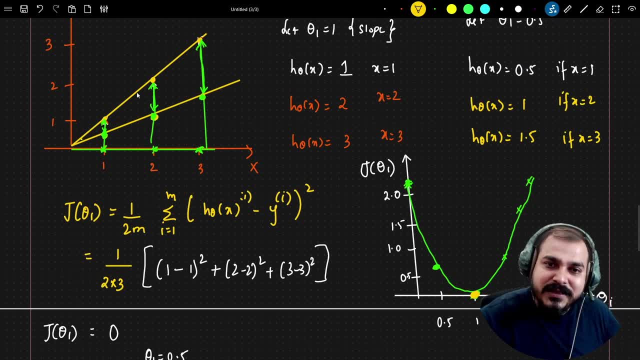 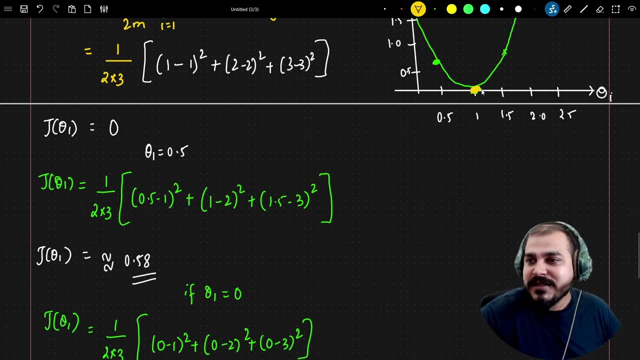 point. you know that the best fit line was this line right at this point of time. my error was very, very less, So I can definitely say: this is the point, this is the global minima, this, this point, is basically called as global minima, And we really need to achieve this particular point, or at least near to this point, to say that 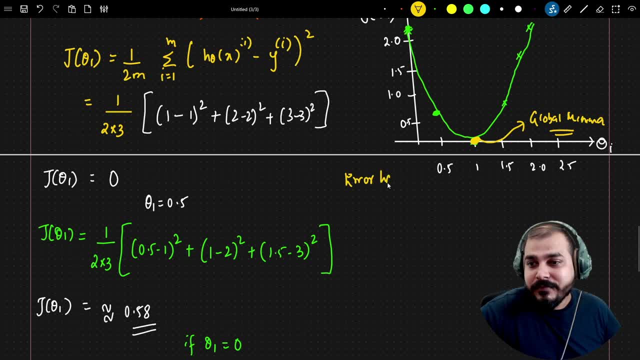 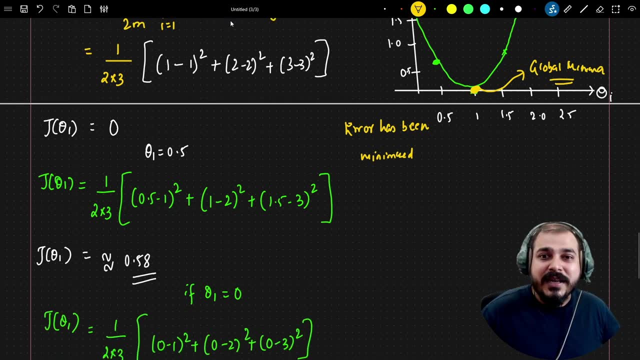 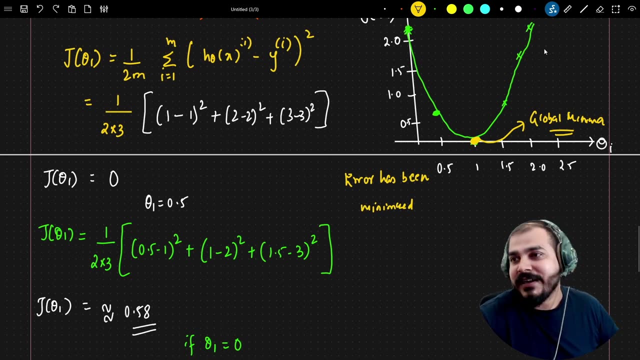 my error has definitely minimized. My error has been minimized Why? Because at this particular point I am actually getting my best fit line. So this entire curve is called as something called as gradient descent. So this curve is something called as gradient descent. 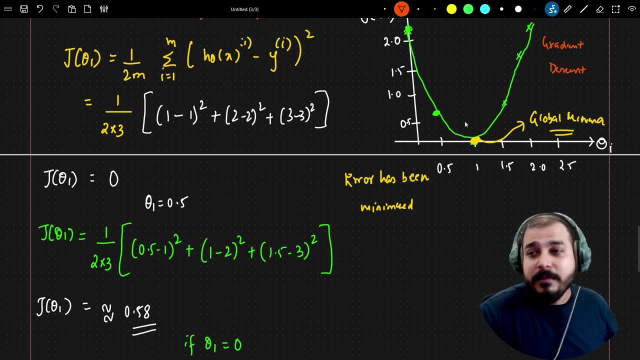 And this gradient descent is super important, even in deep learning techniques. OK, we have to come to this specific point by changing our theta one or theta zero values. OK, so, unless and until we get this particular point, that basically indicates that we are going to get our best fit line. 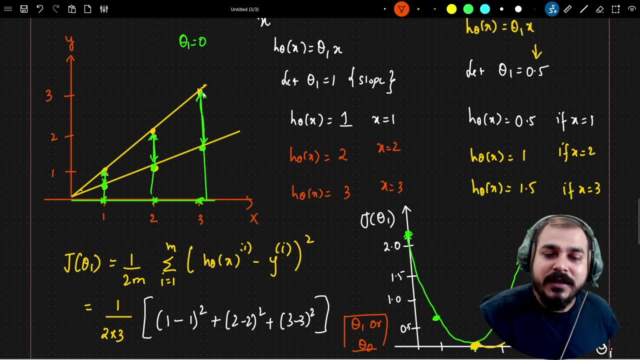 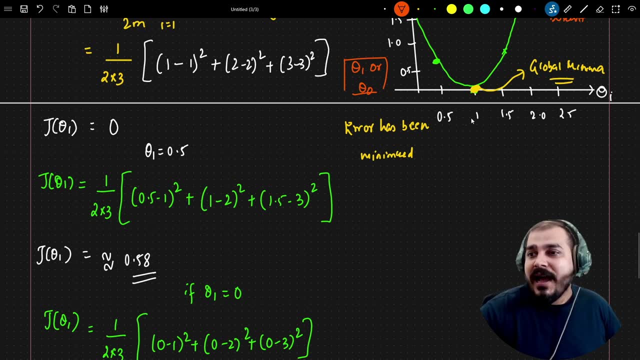 So here you can clearly see that when I had this specific point and over here the cost function was zero, So that basically indicated that I did not have to move much bit over here And this basically indicated my global minimum. OK, global minimum. 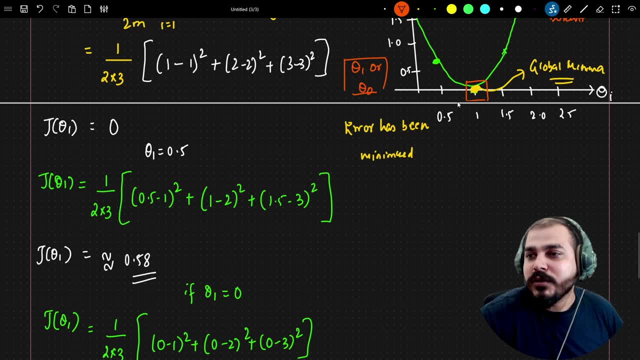 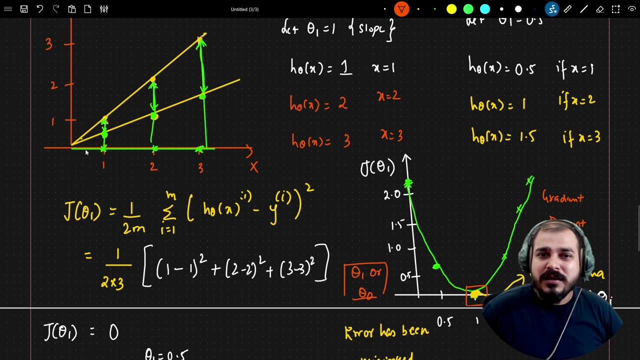 So our aim is that we should definitely try to come to this particular point by moving along this particular gradient: descent. OK, and that is how we should try to change our theta one and theta zero values Right now. since theta zero is just passing through the origin, we don't have to change it much. 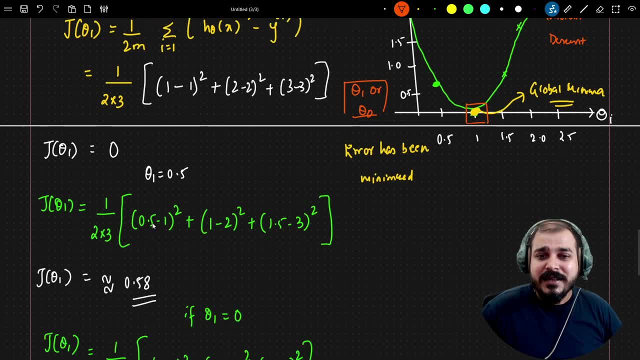 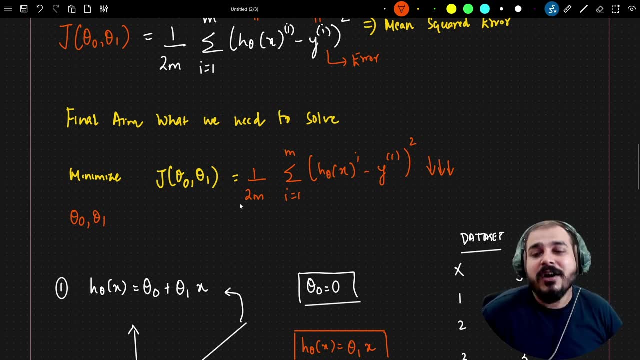 But yes, definitely got an idea about gradient descent and our aim. What would we actually plan to do? We are planning to minimize the j theta zero comma, theta one, since theta zero is zero. So I have not written theta zero specifically over here. 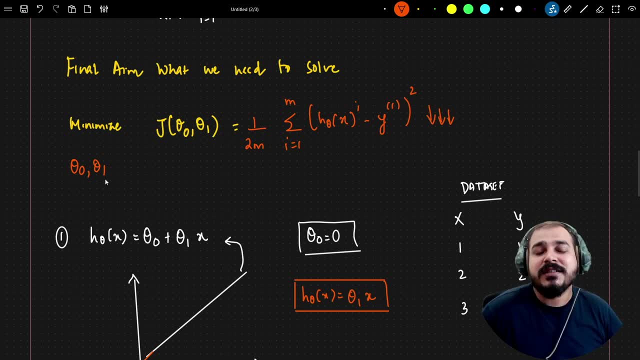 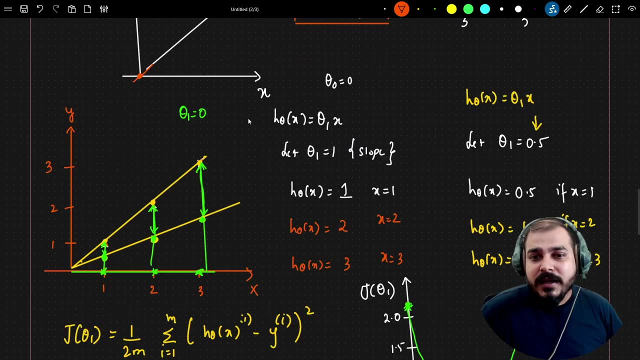 But we had to minimize this by changing the value of theta zero comma, theta one. In this particular case, theta zero was already zero, So we changed theta one value and we minimize this value Right. So here you could see that when we minimize, 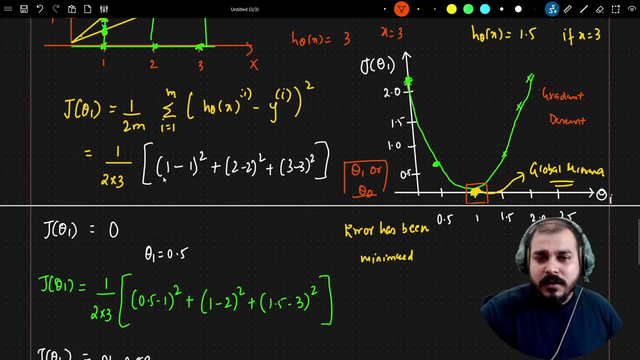 Because see, when my theta one over here, in this particular case my j of theta one- was zero, The cost function was zero. when, when my theta one was one Right. So at this specific instance I was getting my cost function as zero. 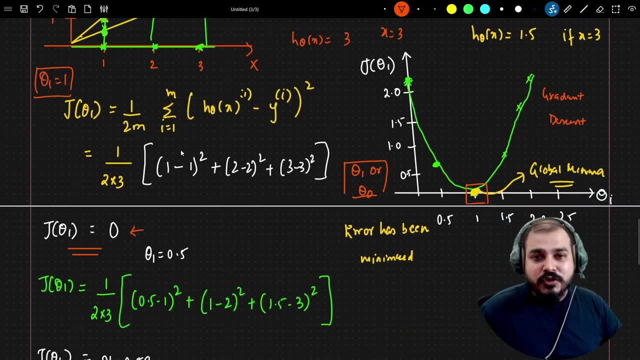 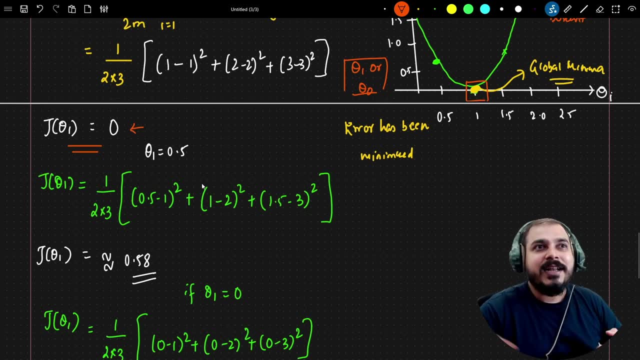 And this was the point where I got my best fit line OK. so in this way we should definitely change these things. But again, I cannot keep on just randomly selecting different, different theta, one value Right. That is not at all possible. 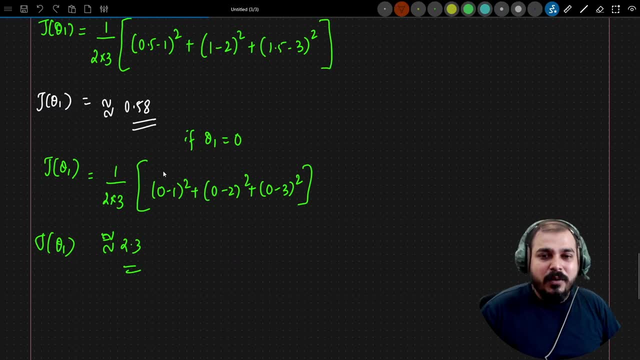 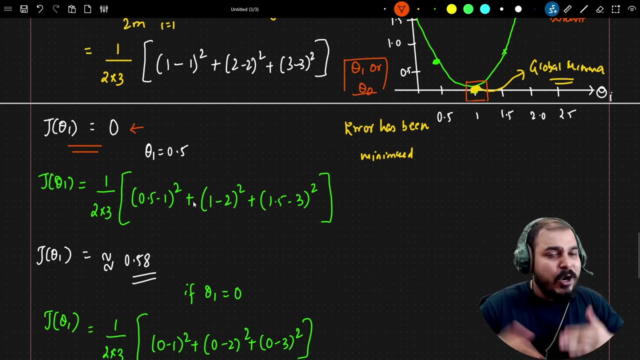 We should apply some kind of convergence algorithm. Now let's, in the next video I will try to make you understand what exactly is the convergence algorithm. Because we cannot randomly initialize theta one value. We should select one theta one value and we should try to find out a mechanism of changing those theta one value. 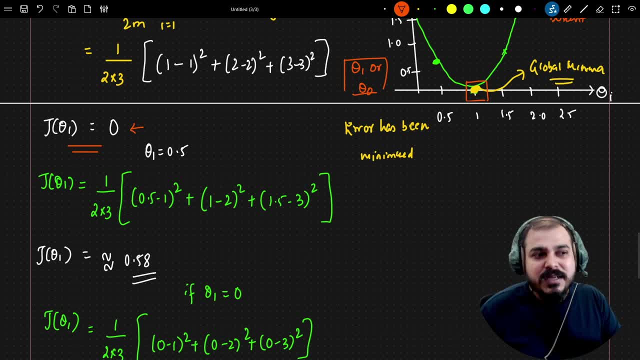 OK. So yes, in the next video we're just going to discuss about the convergence algorithm, So I hope you are liking it. I hope you are able to understand it. If you have any queries, please make sure that you write down. 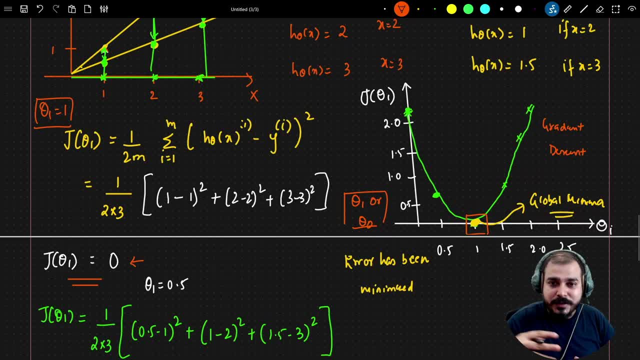 In the comments section we are going to continue the discussion with respect to simple linear regression. In our previous video we had discussed about cost function and how we could actually find out different, different cost function by changing our theta one value, And we also saw that we could form a gradient descent curve. which is this kind of curve? 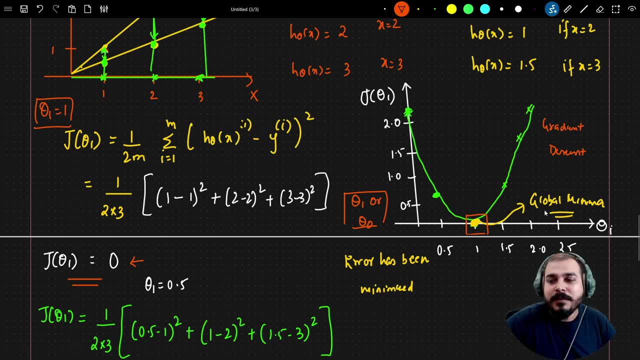 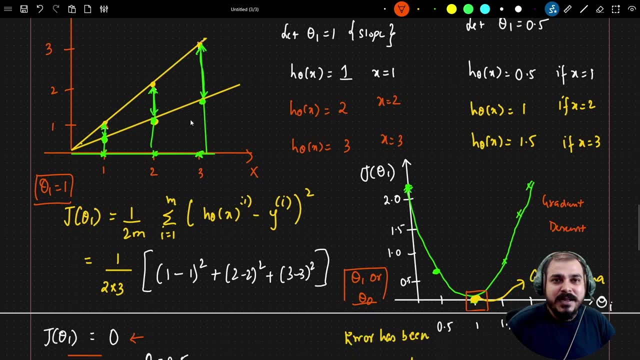 And our main aim is basically to come up to this global minima, because in this global minima, when come near this global minima, that basically means we are very much near to the best fit line Because our cost function is quite minimal. 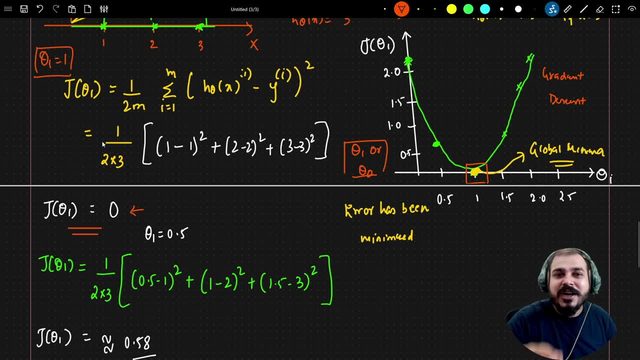 But when we are trying to find out a cost function, we were randomly changing our theta, one value which is our slope. First time I took one, then we took 0.5 and then I selected at zero. This is not an efficient technique. 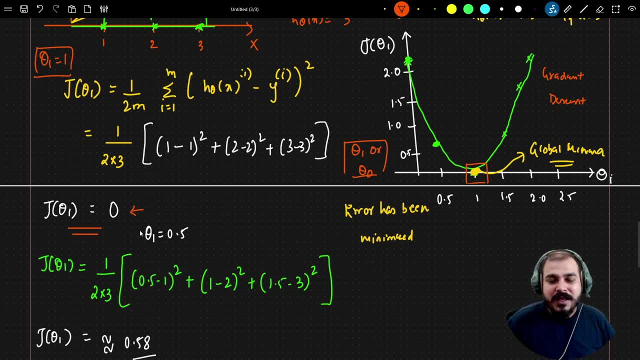 So I told you that we will be discussing about the convergence algorithm, which will actually help you to initialize one theta one value and automatically, you know, based on this gradient descent, it should be able to, you know, increase the theta one value or decrease the theta one value. 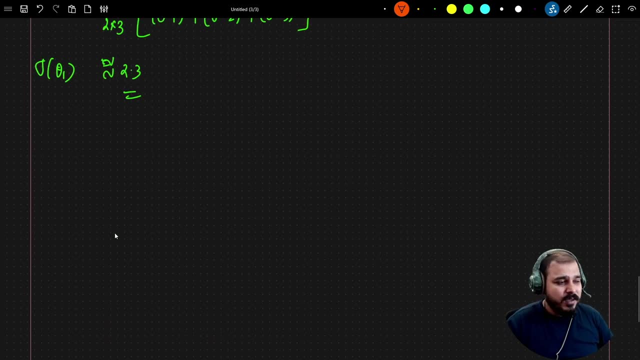 OK, So let's understand the convergence algorithm. So over here I'm just going to mention the convergence algorithm, which is super important for the optimized technique. OK, so this is the convergence algorithm, and this convergence algorithm main aim is to optimize the changes of theta- one value which is my theta, one value which is my slope in this particular problem statement. 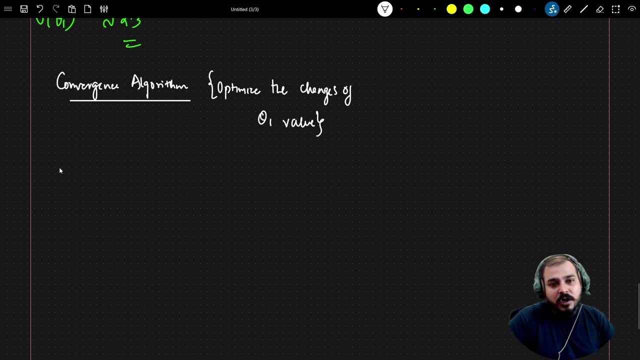 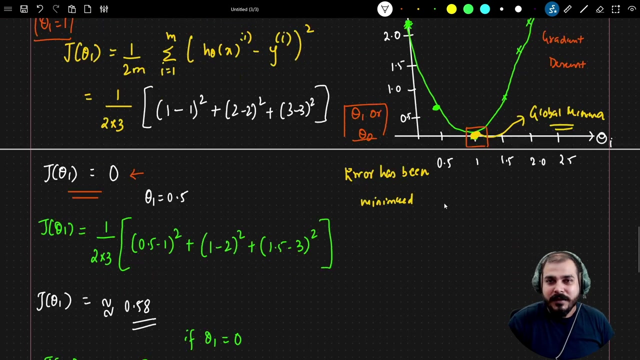 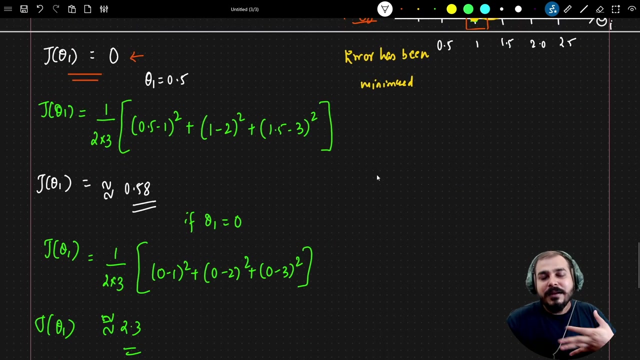 So what does convergence Algorithm basically say? convergence algorithm basically say: repeat Until convergence- OK, until convergence basically means until we reach the global minima, the specific global minima point. OK, the specific global minima point. So here you can see that when we reach this global minima point, we got the best fit line, or at least, if we come near this, we will probably get the best fit line. 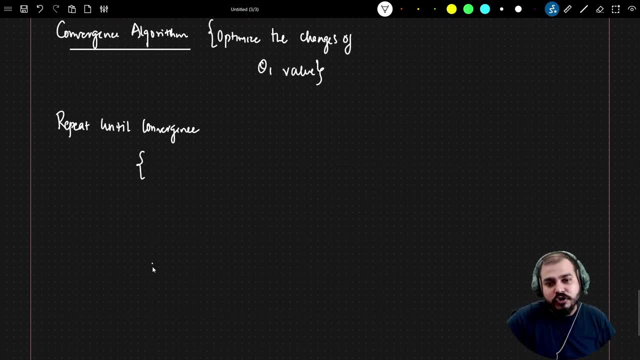 OK, so repeat until convergence. And here I'm just going to write a simple Equation which is like: theta of J. OK, theta of J is equal to theta of J minus. OK, Alpha, alpha. I'll talk about this. 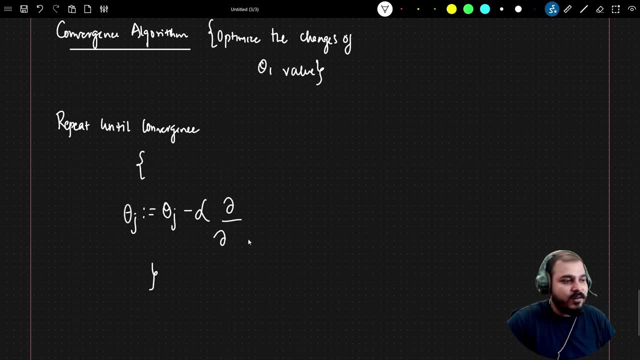 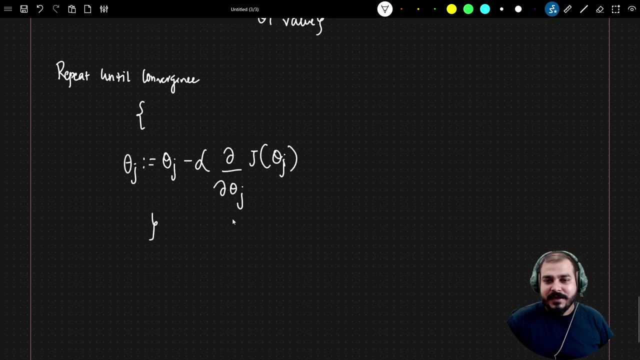 What exactly is alpha? And then we are going to basically write derivative of theta J with respect to the J theta one. OK, or here I'm just going to basically write theta J. Now, what exactly? this is OK, Now Try to understand. 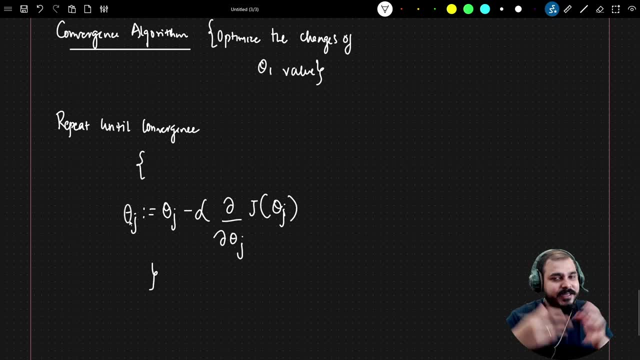 OK, this theta J initially will initialize something and then we'll try to find out the cost function. And obviously you know that with respect to the cost function, how does the cost function basically is created? So here, if I initialize and create a graph with respect to theta J and J of theta, 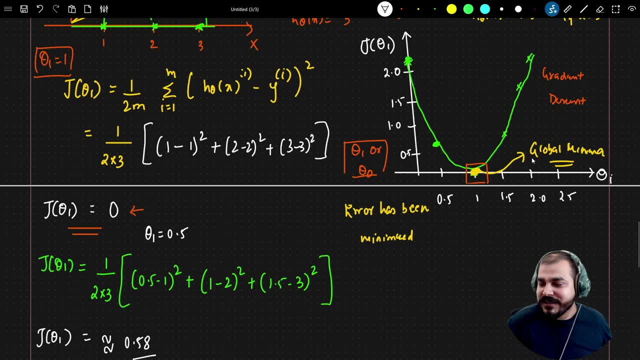 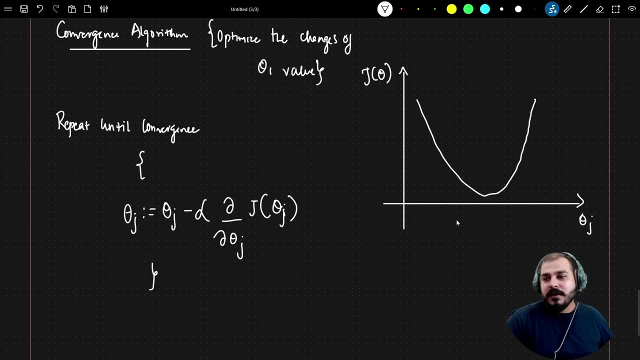 OK, so this is what we created: this graph right over here. You could see this right. You know that we usually get this kind of Gradient descent right, Let's say with respect to: and this equation will definitely work. OK, well, this equation is definitely going to work. 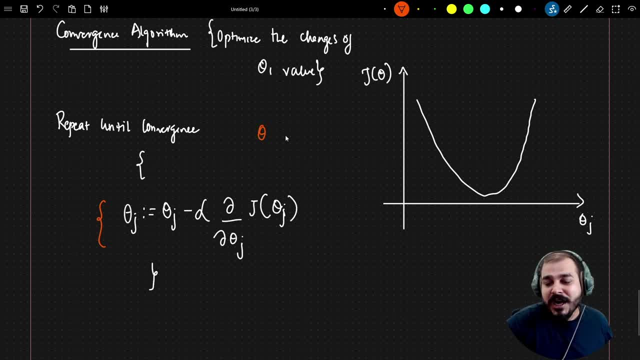 That basically means this equation actually helps us to change our theta value. specifically in our problem statement, the theta one value much more efficiently, much more efficiently. So we are going to change this theta one value much more efficiently. How OK? so let's consider my theta J value is somewhere at this specific point. 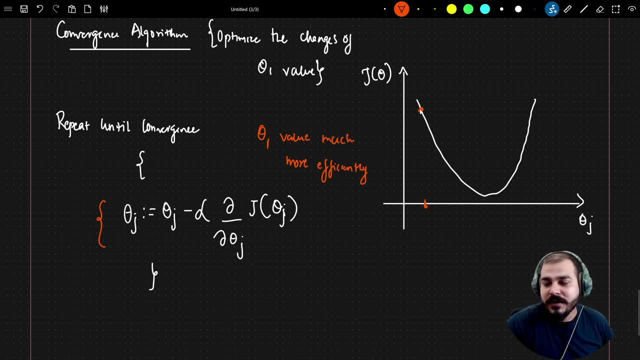 OK, So J of theta will be coming somewhere here. OK, let's consider that this is the point that I'm going to probably get. OK, now you need to understand what exactly this is. OK. derivative of theta J. derivative of theta J with respect to J of theta J. 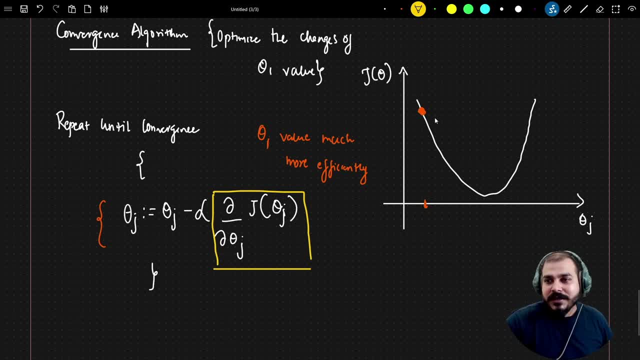 OK, with respect to that. In short, we are just trying to find out the derivative of this specific point. Now, whenever we say derivative, in short, we are going to calculate the slope. OK, Now, let's say we have initialized one theta, one value randomly at this point. 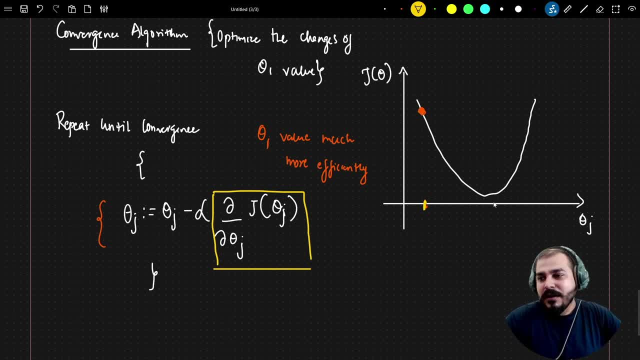 We got our J of theta at this particular point. Now our main aim is that we need to come to this specific point. OK, because why? Why this specific point? we really need to come. Let me just draw it much more betterly. 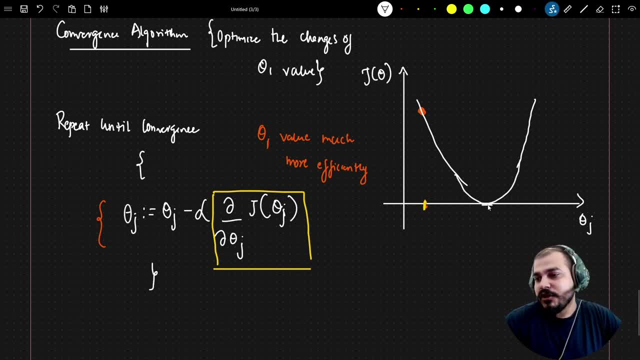 So let's, let's draw this curve like this. Our main aim is to come to this point. OK, this point is basically my global minima, or near to this point. OK, this point, if I come, which is my global minima. 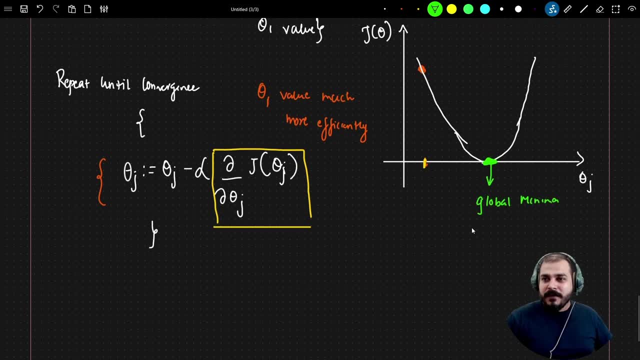 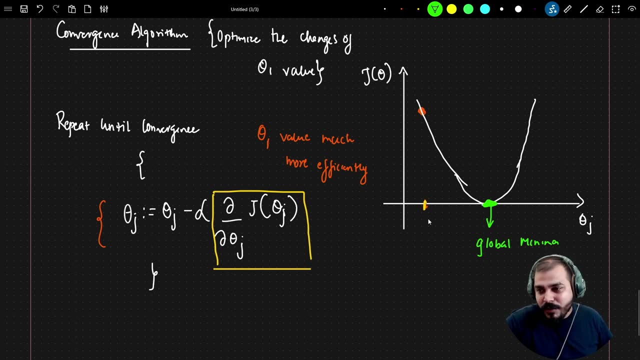 then we are basically getting our best fit line. OK Now, initially, my theta value got initialized at this particular point. I got J of theta, but I have to make sure that I come to this specific one. My J of theta should come to this point so that my cost will basically minimize. 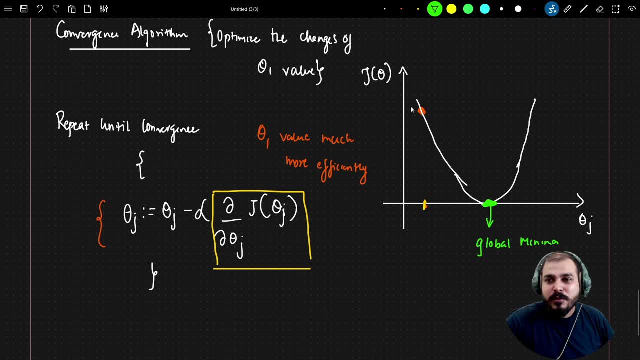 Right Now my theta of J. how do I make sure that? how do I make the changes such that my J of theta will come over here that we are going to look at Now, as soon as it comes over here, this derivative of a derivative of J of theta with respect to theta. 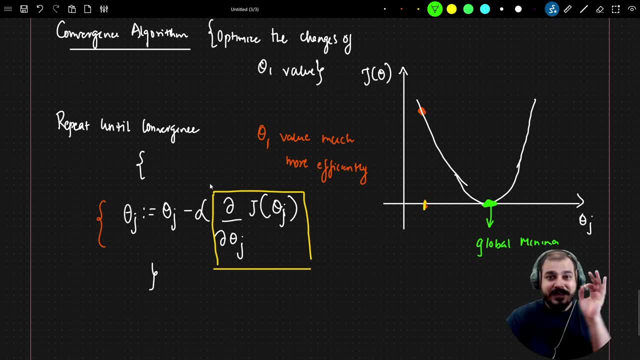 J is nothing, but we are trying to calculate the slope at this particular point. That is what derivative specifies. OK, now, in this particular case, how do we understand what is the derivative of this particular value? OK, in order to find out the derivative. 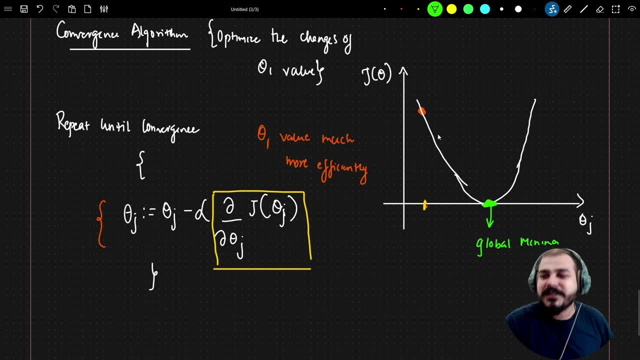 one important thing that you really need to find out is that, whether this is a positive slope or negative slope, because derivative is nothing, but we are actually trying to calculate the slope. OK, we are trying to find out the slope. OK, so, for this particular point, what we do in order to calculate the slope? 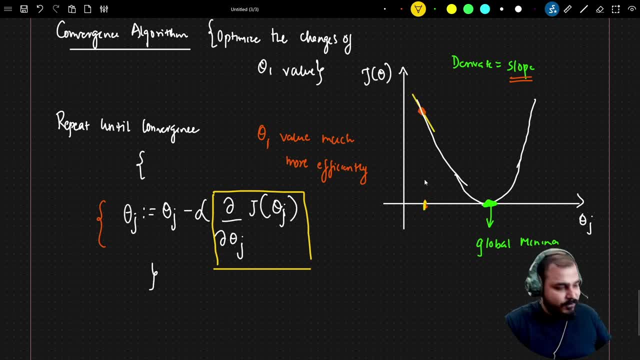 we create a tangent line like this. OK, let's say that we are creating this tangent line, So this tangent line will probably get created like this. OK, now, when we are creating this tangent line, first of all you need to find out that. see the right side of the line. 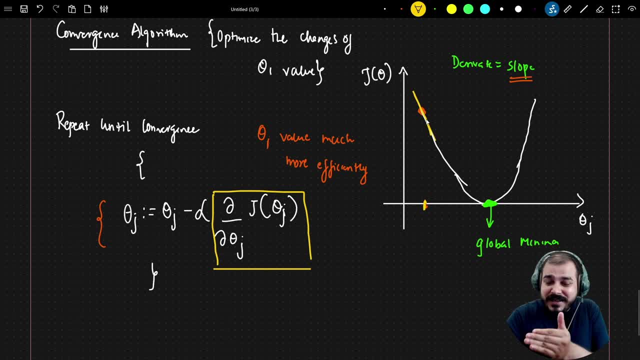 OK, because one important thing that we need to find out over here that whether it is a positive slope or a negative slope. because if we are able to find out whether it is a positive slope or negative slope, then we will be able to understand whether we have to reduce our theta j. 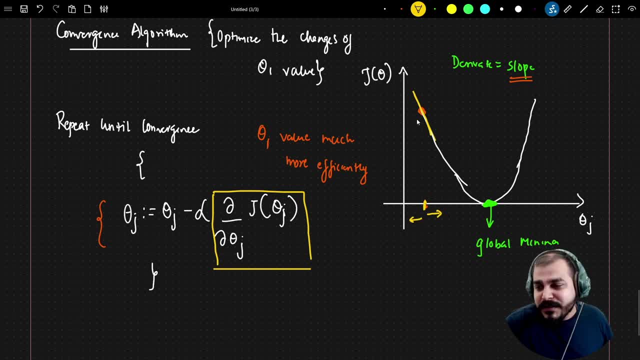 value, or whether we have to increase our theta j value. OK, now, in this particular case, at this particular point, if I really need to understand whether this is a positive or negative slope, just see the right part of the line. The right of the part of the line is facing downwards. 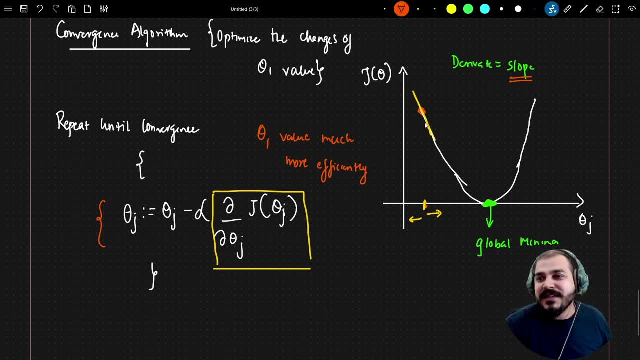 OK, if it is facing downwards, we will be seeing this as negative slope. Now, when we say negative slope, that basically means, whenever we try to find out the derivative, this value is going to be negative. OK, this value is going to be negative. 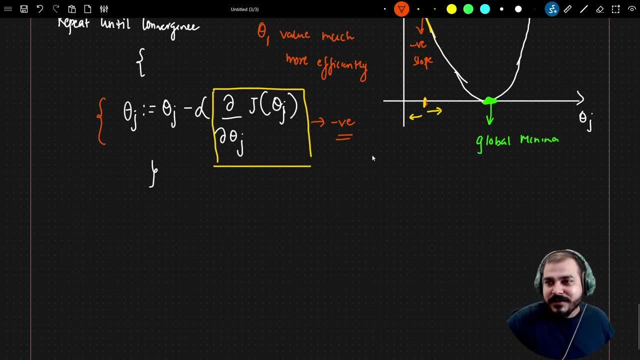 So what we are going to do is that we will just suppose I get a negative slope. So, in short, I will write: theta j is equal to theta j minus some learning rate. alpha- I'll talk about why alpha is used and this will be my negative value. 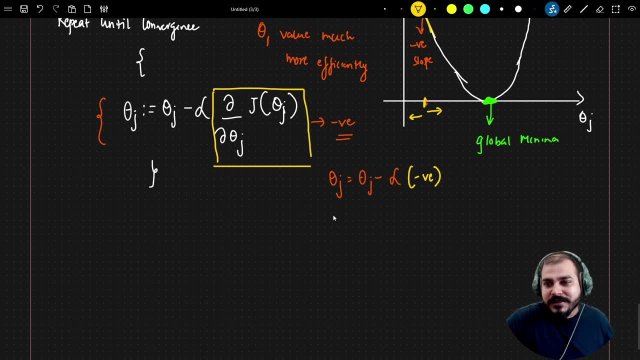 OK, this will be my negative value. So in short, this basically indicates that my theta j is negative. So if I write theta j, I have to probably add with some positive value, right, Because negative into negative will be positive. So I have to add this specific positive value. 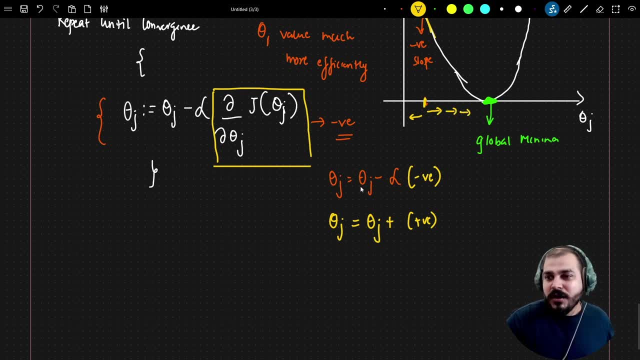 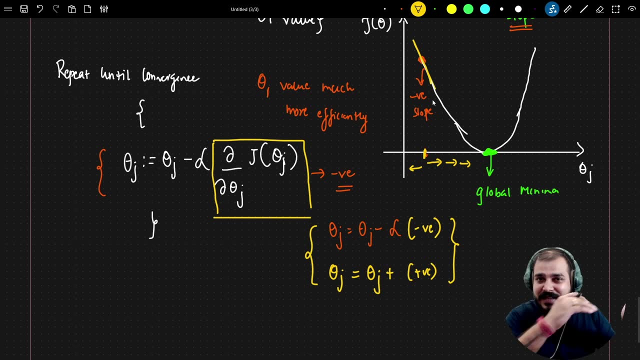 And it is true over here- because I need to basically increase my theta j value. So if I do this iterative process again and again, wherein I'm continuously getting a negative slope, that basically means I have to increase my theta j value so that I reach my global minima. So this equation is going to add some value. 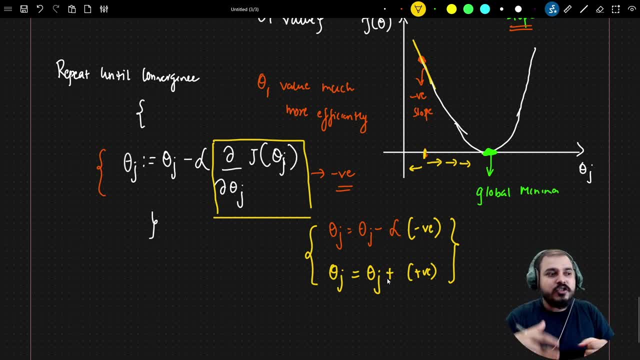 to this value? We don't know, since this is an iterative process. Our main aim is to basically optimize. optimize this process of selecting different, different theta. one value, right. So in this way, what will happen? We are incrementing or we are increasing our theta j value? 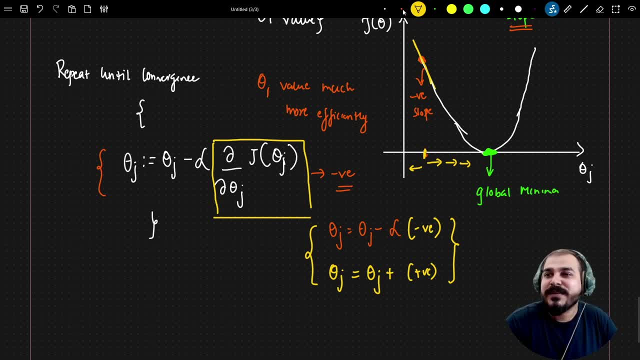 Then in the next theta j, whatever will be my cost function, Again that specific point will come over here. Let's say it is coming over here. Then again I'll try to go and find out this slope Again. if it is a negative slope, we keep on adding. 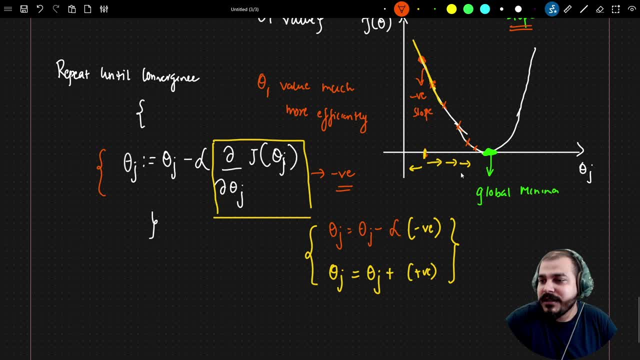 So slowly, slowly, you will be seeing that we will be able to converge it towards the global minima. OK, this is one process. What about? what about now? in this particular case, I got negative slope. What about if I get another point over here, and this particular point is: 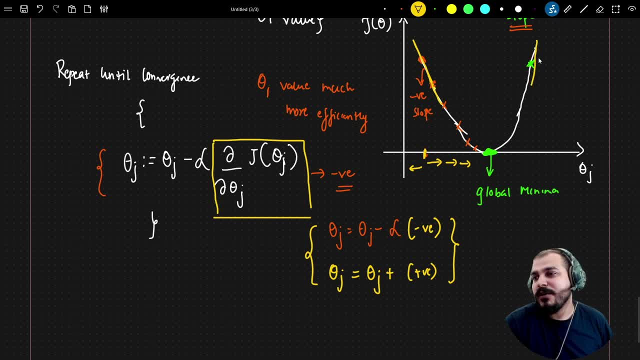 actually a positive slope. how do I get a positive slope? Because if I try to create a best, if I try to create a tangent line, just see the right part of the line. right part of the line is pointing upwards, So this becomes a positive slope. 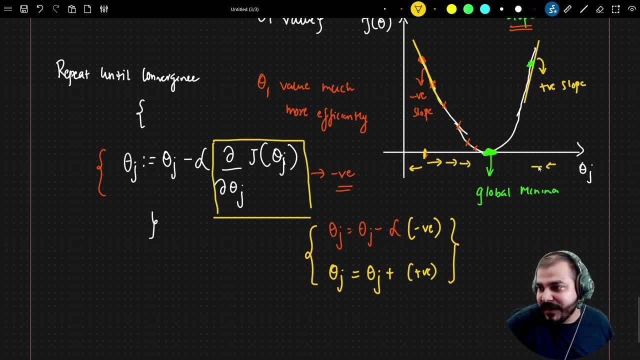 Now, in the case of positive slope, I really need to decrease my theta j value, right? Let's say that initially my theta 1 was over here and I got my j of theta 1 over here, So here I have to decrease it. 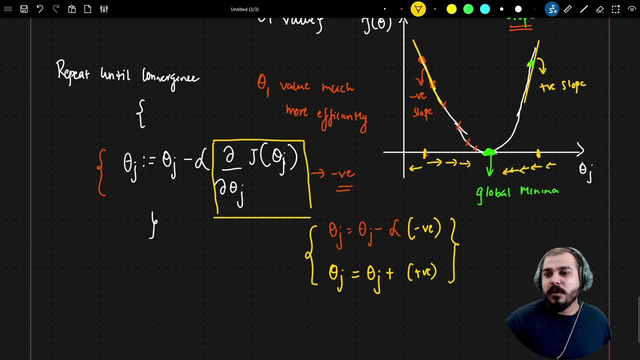 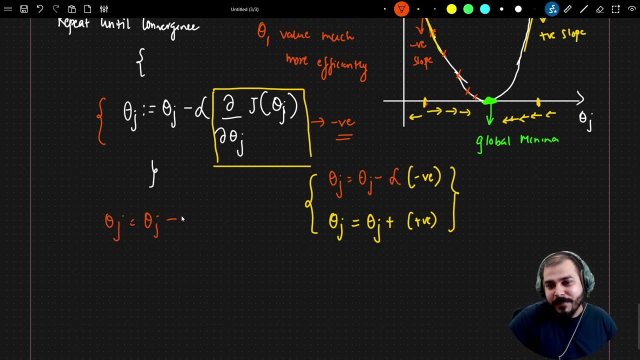 OK, I have to decrease it. Then only I'll be able to reach the global minima. So does this satisfy? Yes, it does satisfy, Because if I write now, theta j is equal to theta j minus alpha. And now this is my positive slope, right. 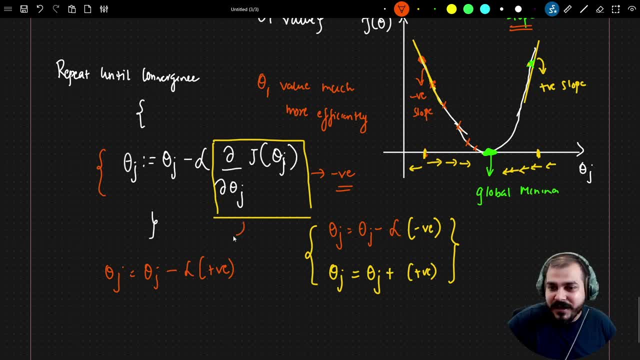 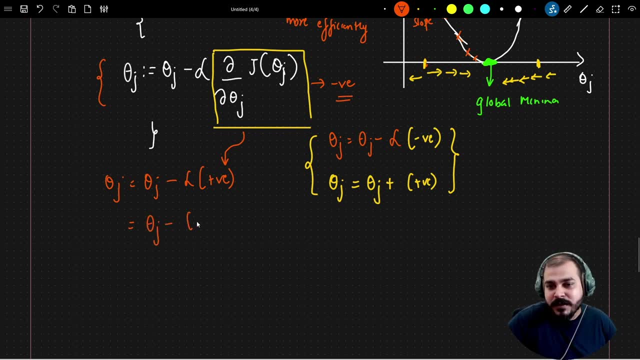 So here, with respect to this, whenever I try to find out the derivative, it is a positive slope. Now, whenever it is a positive slope, all I am actually doing I'm subtracting with some value, some positive value. When I subtract with some positive value, 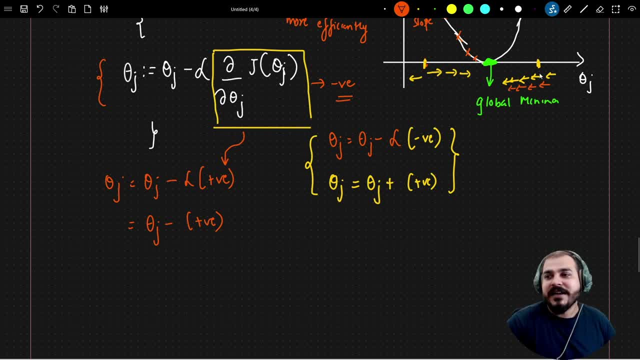 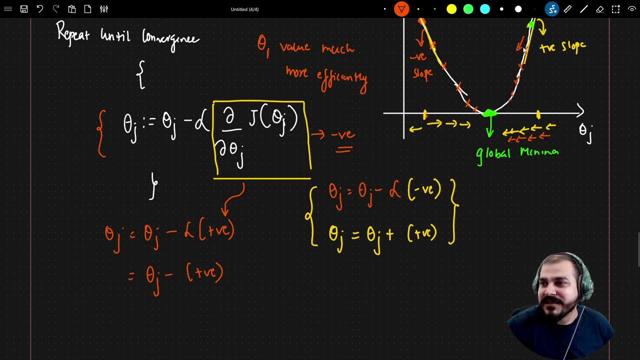 that basically means I have to basically decrease my theta j value And if I continuously perform this process, after some time you will be able to see that I am going to basically come at this specific point. OK, so obviously this convergence algorithm will obviously work because 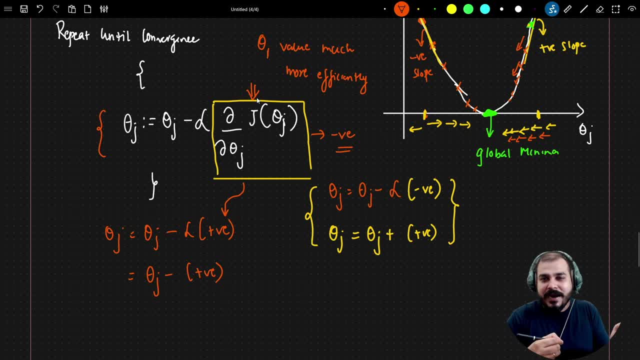 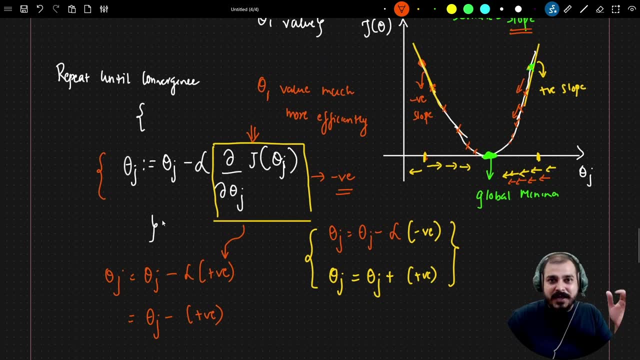 what I am actually doing is that we are trying to calculate the slope In such a way that, if it is a negative slope, the theta j value is going to increase. If it is a positive slope, the theta j value will decrease. OK, so this is what is a convergence algorithm all about. 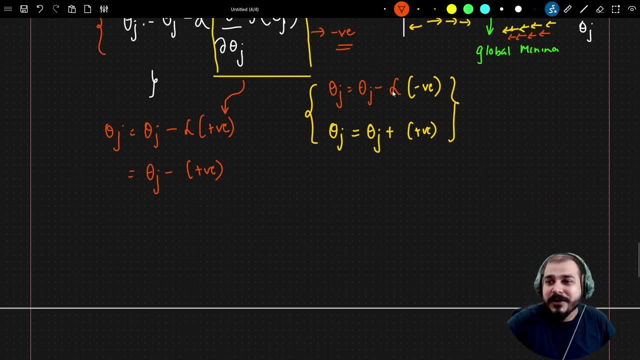 OK, now there is one important parameter that we did not discuss about is something called as alpha. So what exactly is this alpha? Alpha is nothing, but this is specifically a learning rate. Learning rate usually is a smaller value that is basically initialized. Let's consider the learning rate that may be initialized. 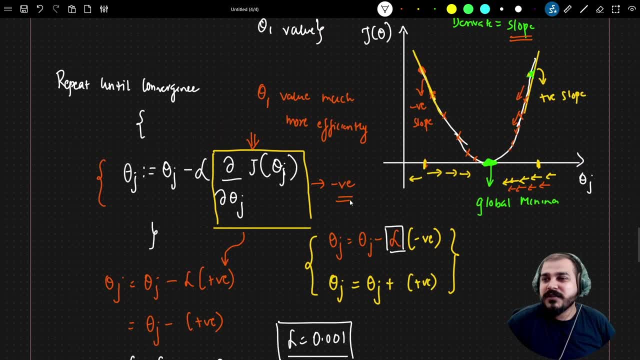 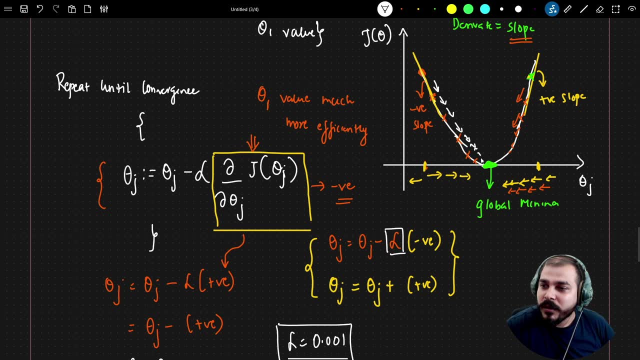 For my problem statement is 0.001.. Now, what is the importance of this learning rate? Learning rate controls the speed at which the convergence should happen. OK, if it is a very, very small value, then it will probably take more time to converge. 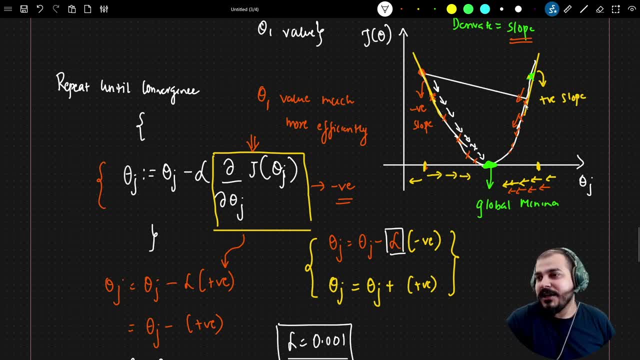 If it is a very big value, then it may happen in such a way that it may continuously jump here and there and it may never converge. So it you always have to make sure that you try to select a smaller value, but it should not be a very, very small. 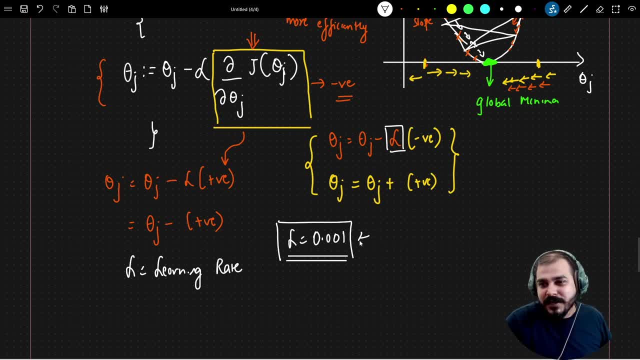 value. it should be like 0.001, which is a very good practice that we should try to select. OK, in simple linear regression, only alpha is equal to 0.001.. In a scale on library that we use is basically getting selected. 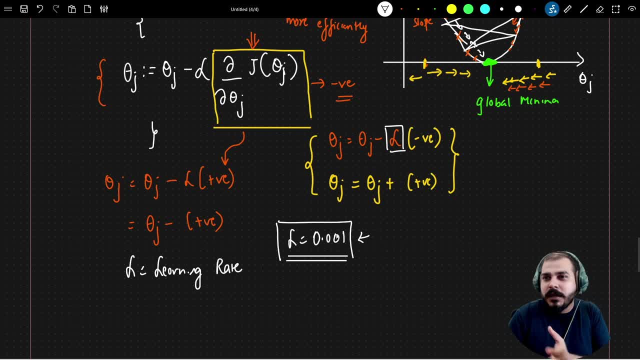 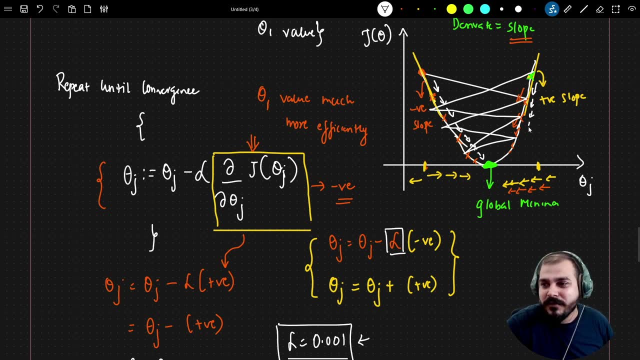 So if anybody asks you in an interview like: what is the importance of learning rate, You can definitely say that it actually controls the convergence- How slow the convergence should happen. OK, so this is what it basically says. So I hope you have understood about the convergence algorithm. 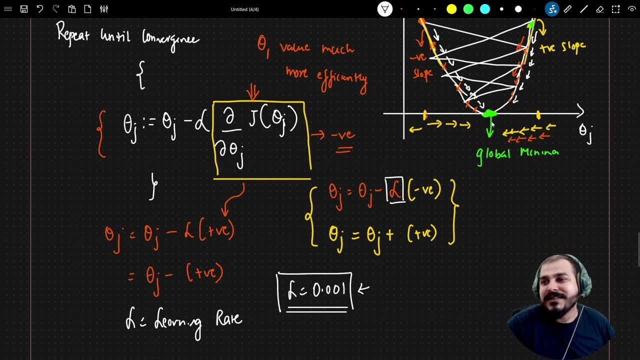 And this process continues unless and until we don't come near this global minima and we don't basically converge over here. As soon as we converge at this particular point, you will be seeing that we will try to get the best fit line, which is this specific line with respect to any kind of data points. 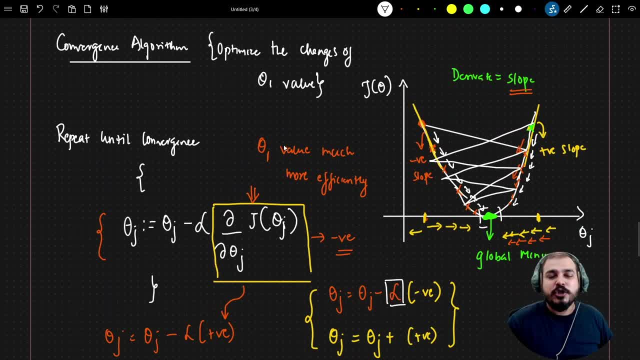 So this is the most important optimized technique that we should use. with respect to the convergence algorithm. OK, and this basically gets applied in an amazing way. And most important interview question is: when you're learning machine learning algorithm. So yes, in the next video we are going to also continue and understand about the performance metrics. 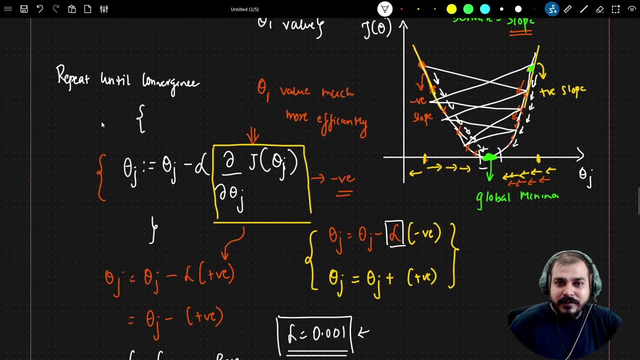 Finally, you know, in our previous video we have seen till here, We have understood what is the convergence algorithm and how we can actually update our theta value. you know which is my coefficient. you know, based on the positive and negative slope. 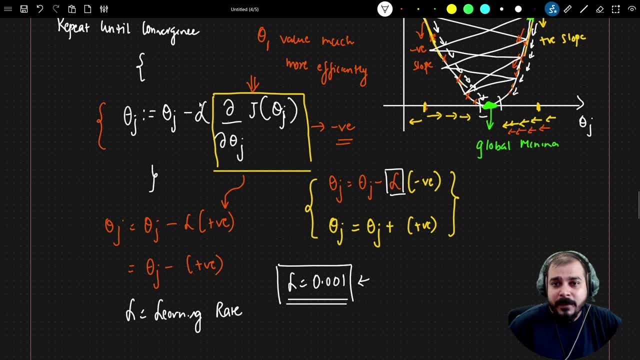 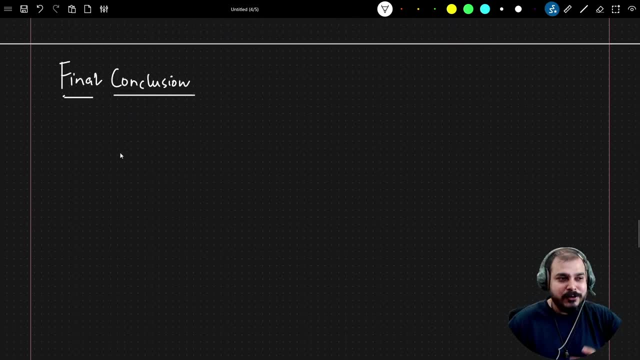 And this was the theta, or coefficient updation formula, Here, alpha also, we used it, and this specific alpha was nothing but learning rate. Now I really want to make one final conclusion And probably write some some more equations. you know, and we can just consider that till now, 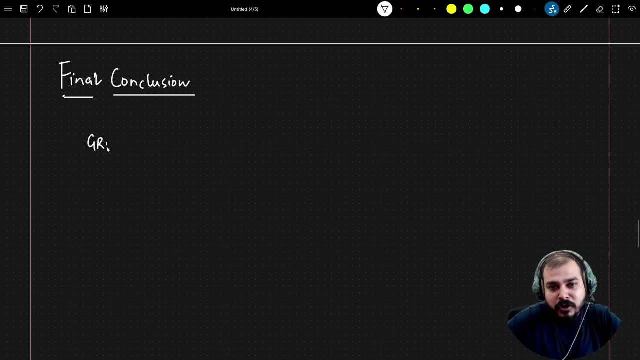 You know, we saw that we have actually covered something called as gradient descent Right And gradient descent whenever we talk about gradient descent. So, in short, we are talking about that curve. OK, so in short, we are talking about this specific curve. 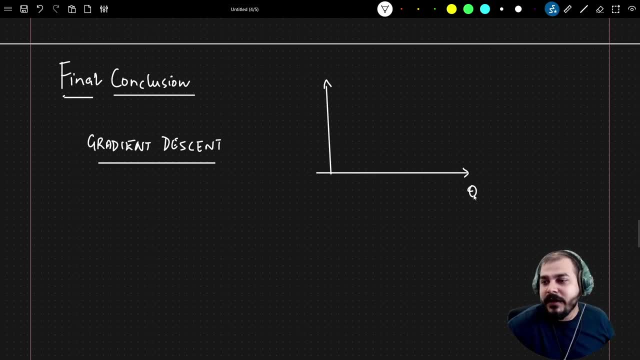 And this curve is basically we get it from when we try to plot with respect to theta and j of theta Right. So over here you'll be seeing that this is the curve that we usually get And our main aim is basically to come to this global minima. 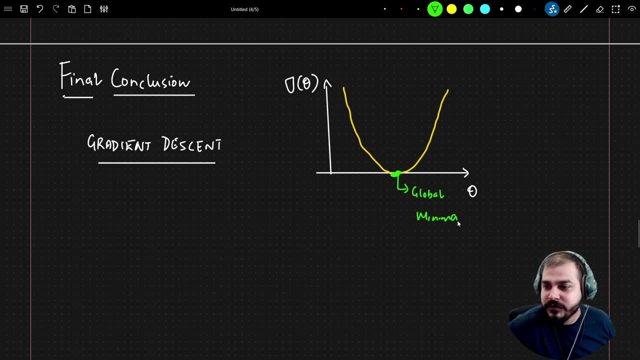 Right. So this global minima And we try to update our theta based on this. Basically, we try to find out whether the slope is positive or negative And based on that, either I need to update the weights, increase, increase this specific coefficient or decrease the specific coefficient. 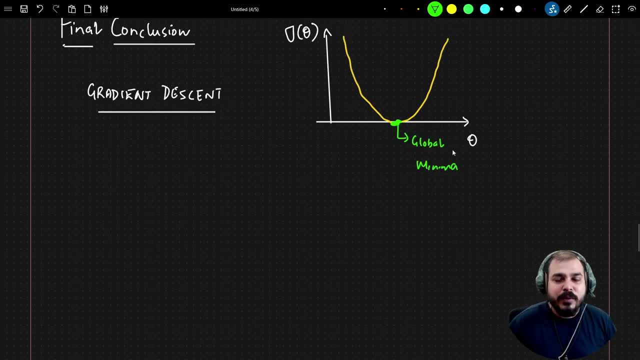 which I have actually explained over here. Now for our example. you know we had actually considered, you know we had actually considered what Our intercept is. zero. That basically means our best fit line passes from this to this And since it passes through this intercept, 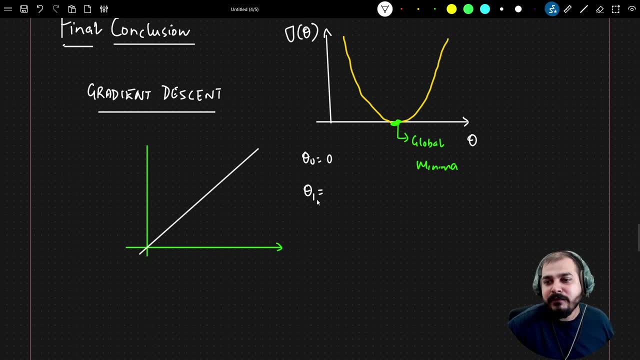 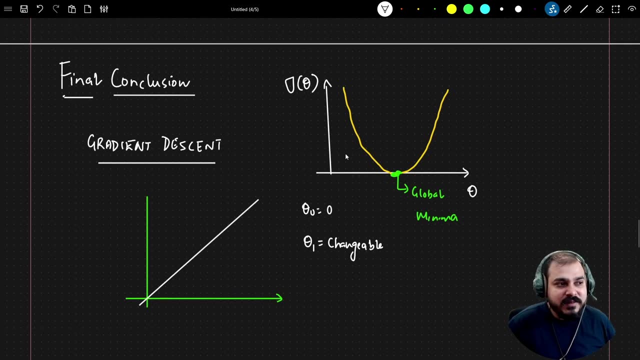 so we consider theta zero is equal to zero and we were changing theta one value. OK, so this was basically changeable. Right, We do not focus more on theta zero. The reason why I did this is that because I wanted to show you the gradient descent in the 2D diagram. 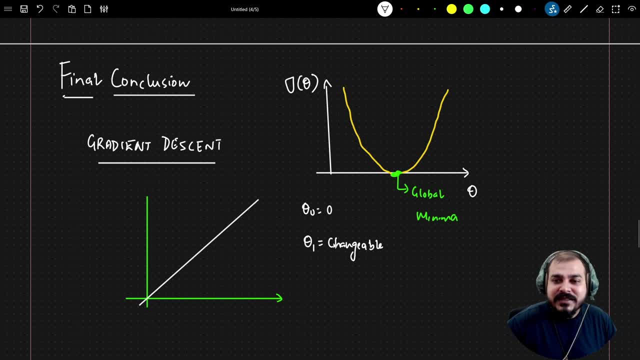 So over here when I'm drawing this, this is basically in the 2D diagram. Let's consider that theta zero is not zero. that basically let's say that if it is not passing through the origin, then this 3D diagram may look something like this: 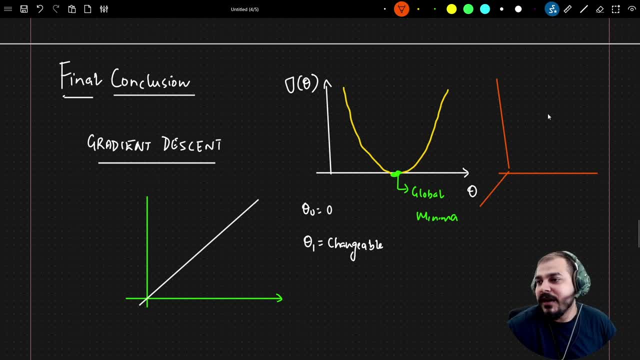 Right, So it let's say this: this entire diagram will look something like this. I am just creating for an example, So it may look something like this. OK, It may look something like this. Let's say: consider that it is coming. 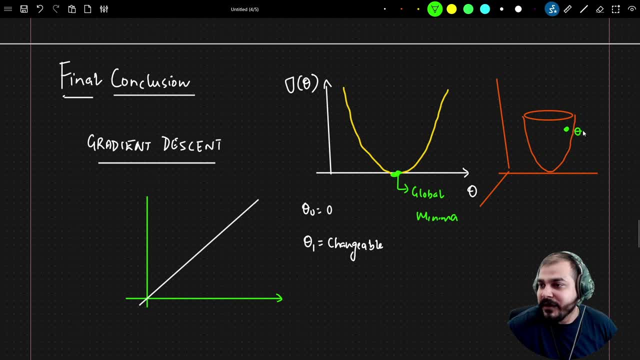 It looks like this. So one theta one may be somewhere here. OK, theta zero may be somewhere here. And our main aim is basically, to you know, merge towards this global minima, Right? So our aim is basically come to this global minima. 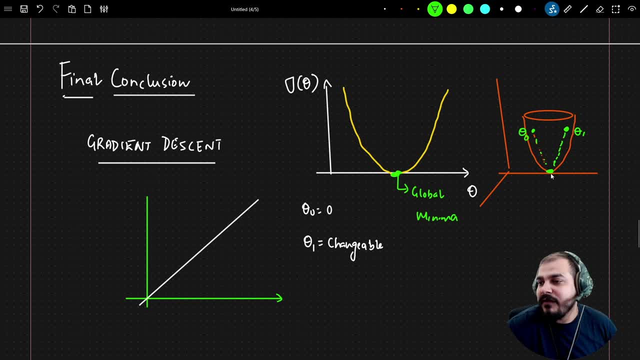 So this will also get updated like this, and this will also get updated like this, And finally we reach the global minima. So that we usually do in a 3D diagram- And obviously I cannot draw a 4D diagram, but just understand- it's like 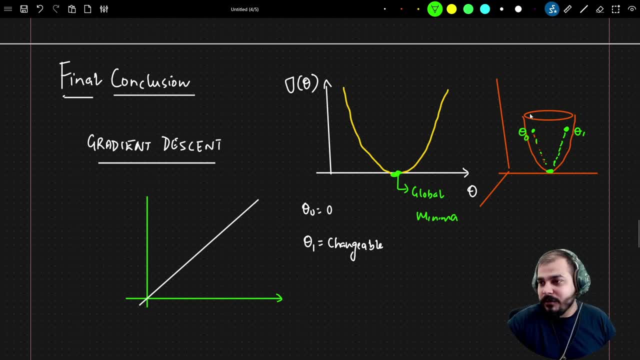 inverted mountain and from the bottom, from the top, you are basically coming to the bottom right. so bottom at one single point. So this particular point will be the global minima. Now, if I consider theta zero and theta one, let me go ahead and 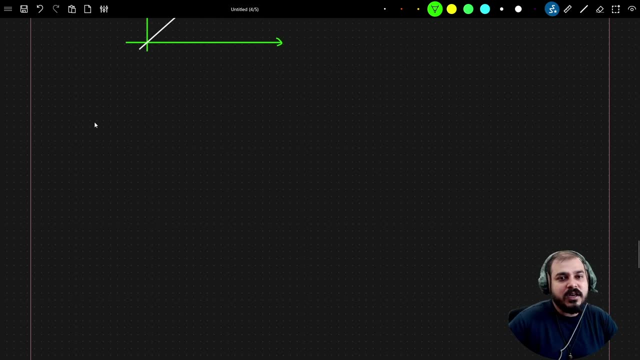 write my convergence algorithm. OK, so what was my convergence algorithm again? So I'm just going to update my convergence algorithm. OK, And the convergence algorithm was pretty much simple. Here I will say that: repeat Until convergence, the same thing what I have written on top. 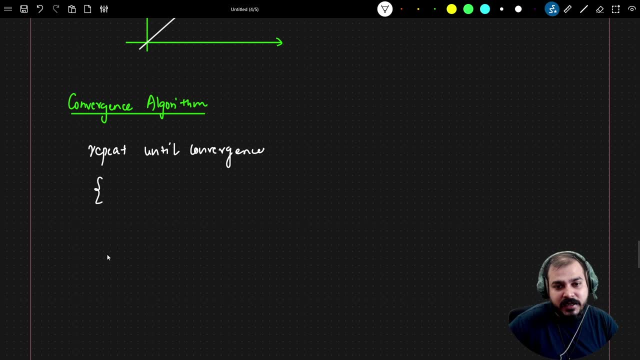 OK, repeat until convergence. But here my theta j will get updated something like this: Right. So theta j is see this symbol that I'm using right. This is a continuous iterative process, So that is the reason I'm writing this colon and equal to. 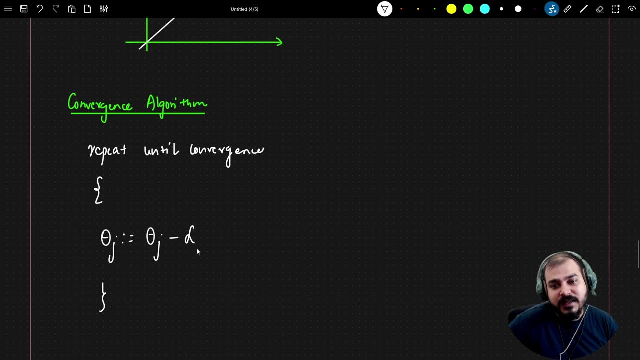 So it will just get updated with respect to this, theta j minus alpha, which is my learning rate, And then derivative of theta j. OK, And one point I have to use is nothing but j of theta zero, comma, theta one Right now, since my theta zero is not zero. 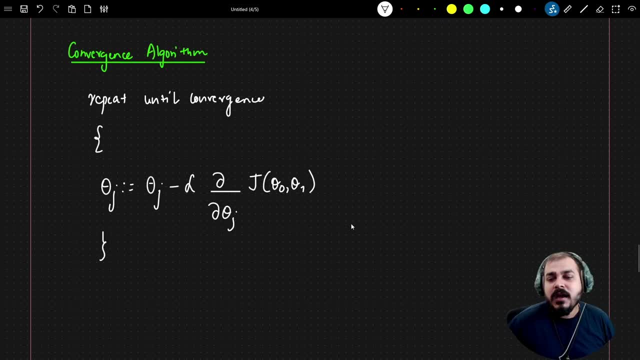 so I have to basically find out the derivative of both these things. And you know that. what is j of theta zero comma theta one? OK, we already explained it. So j of theta zero comma theta one is nothing but our cost function. So if I know my cost function, it is nothing but one by two m. 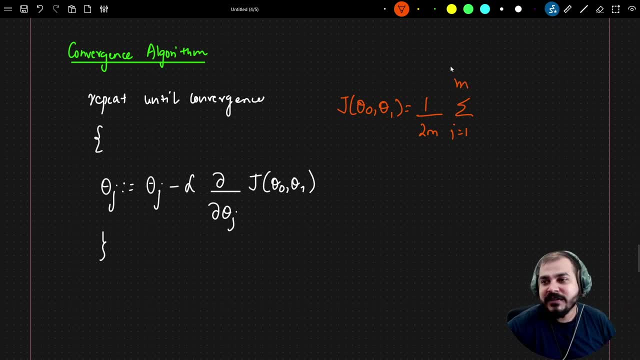 Summation of i is equal to one to m. m basically means how many number of data points I have, And then I have h theta of x of i minus y of i, whole square Right. So this is the cost function that I specifically used for j. theta zero comma theta one. 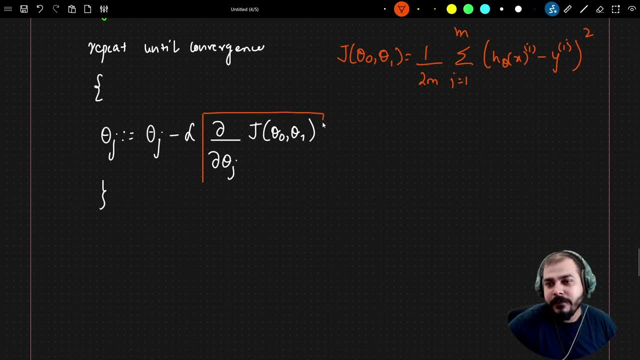 Now my main aim is basically to go ahead and calculate this derivative. Now I'll try to just show you. It's OK if you don't know derivatives also, guys, but understand, our main aim is to basically converge to the global minima. 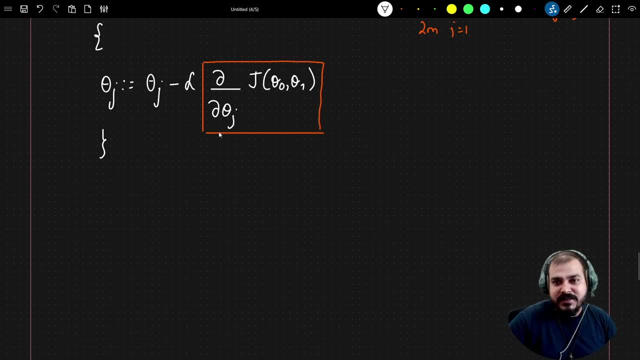 Right. So here I will just go to write something like this. I'll just try to calculate this And over here, you know that since you have theta zero and theta one, your j value will be zero and one right, zero and one. 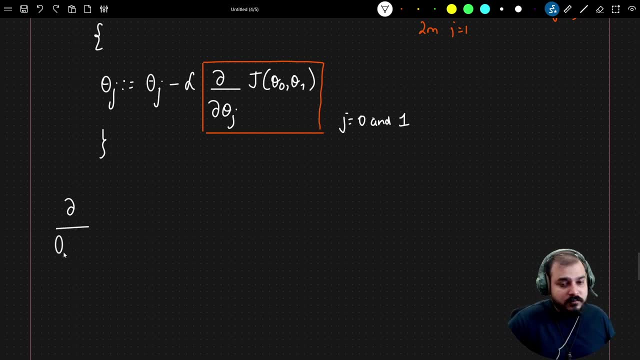 So let me just go ahead and write it over here. So derivative of theta j. OK, with respect to j, with respect to j, theta zero comma, theta one is equal to derivative of theta j. OK, and I have over here one by two m. 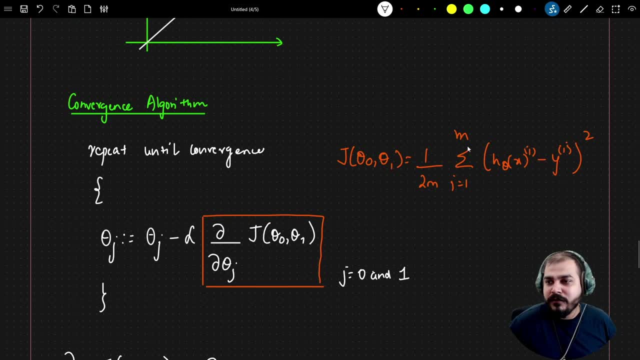 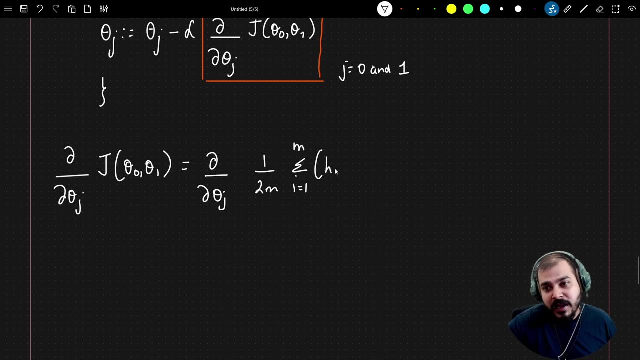 I'm just replacing j theta, comma one with the cost function, Right, Whatever cost function I'm writing. So one by two m summation of i is equal to one to m. OK, and then I have over here h theta of x of i minus y of i, whole square. 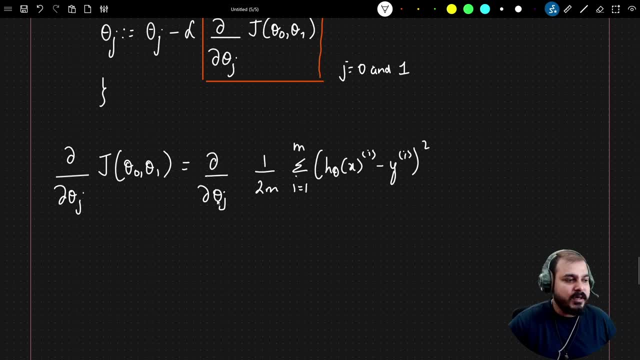 Right, So this is my entire derivative of j theta zero. OK, and you know, let's go ahead and try to find out the derivative of this. Now, guys, it is simple, Right? If I take an example, if, probably in high school, you have learned about derivative, 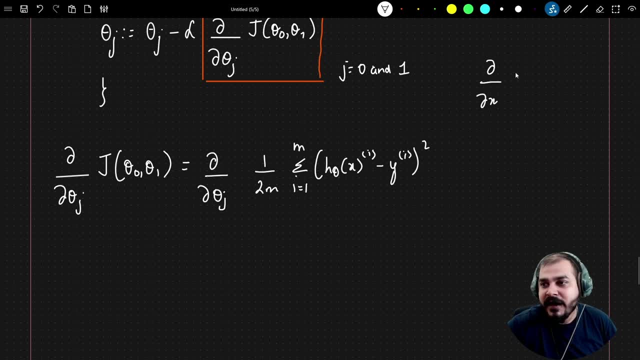 derivative basically means we're trying to find out the slope. Suppose, if I really try to find out the derivative of x square, Right, So what I will be getting, I will be getting with respect to this. See, I'm trying to find out the derivative of x square with respect to x. 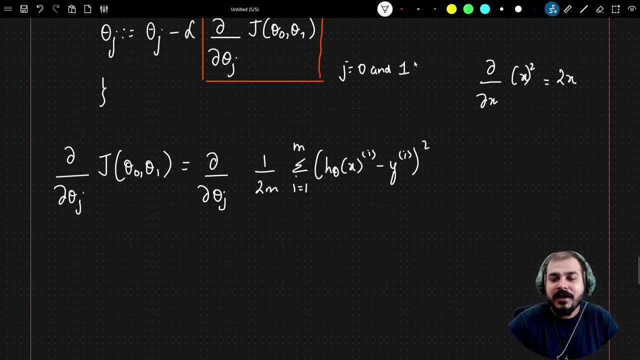 So this will be nothing but two x, Right, It's just like n. x to the power of n derivative is nothing but n multiplied by x to the power of n minus one. So this is what is the formula Right. So, similarly, I'm going to apply this derivative for this particular equation. 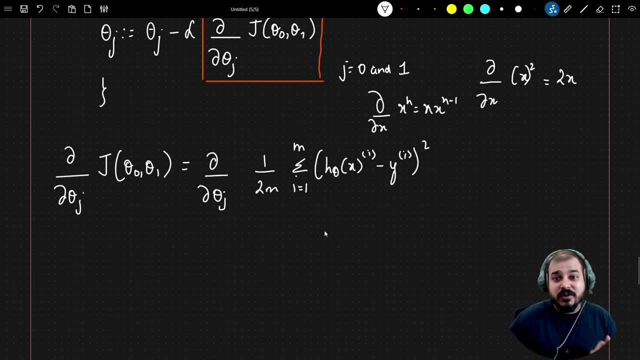 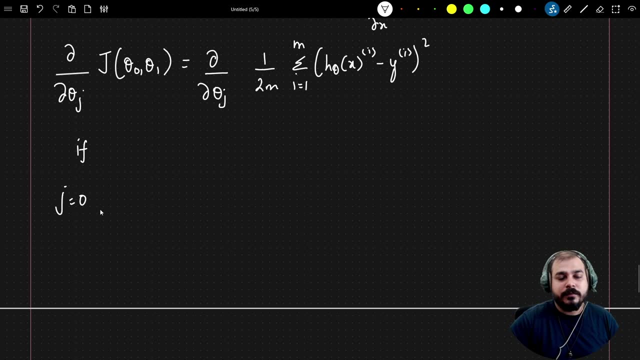 But when I'm finding the derivative, I have to find it, for j is equal to zero and j is equal to one Right. So I'm just going to write over here: if J is equal to zero Right. So if j is equal to zero, this entire equation. what it will become is this: 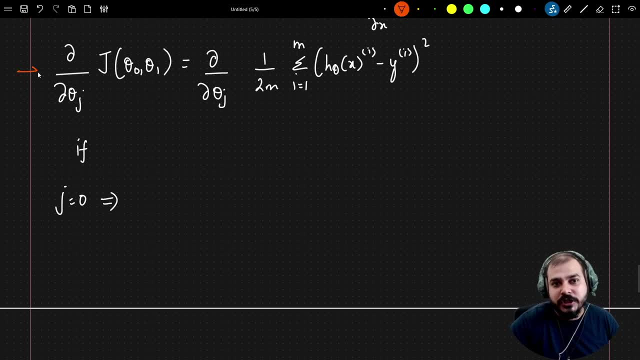 entire equation, this entire equation, the stop equation, this entire equation will be becoming derivative of the derivative of theta zero j, of theta zero, theta one, which is nothing but derivative of theta zero, one by two m. And here I'm basically going to use 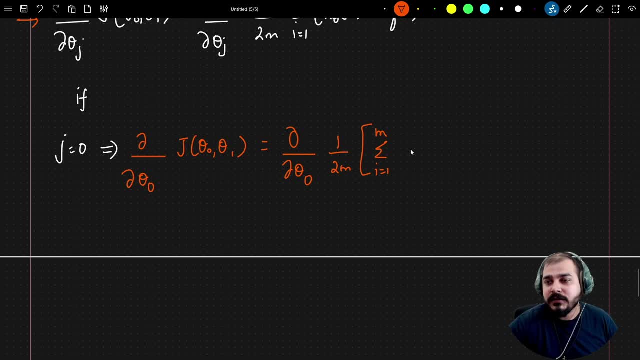 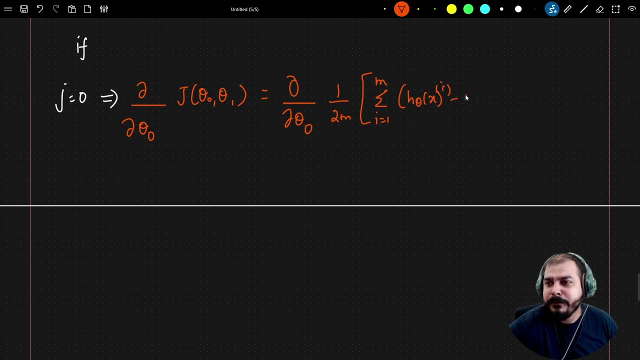 Summation of i is equal to one to m, and this will basically be- I'm just writing the same thing, right s theta of x of i, x. theta of x of i minus y of i, whole square Right. So this will be my entire thing. 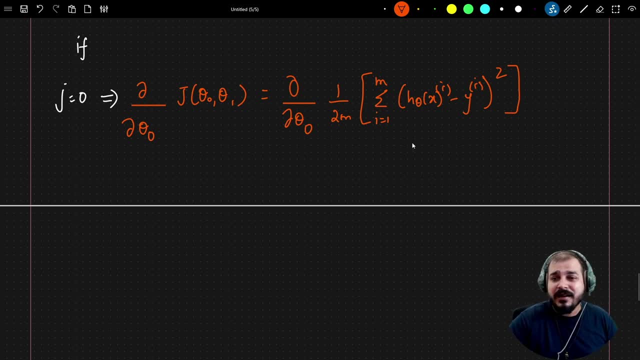 Now here you can basically see that. fine, I'm getting this exactly. Now I'll just go and find out the derivative with respect to theta zero. So if you know this equation, always remember this is just like your x squared. Let's consider: this is my entire x squared, Right? 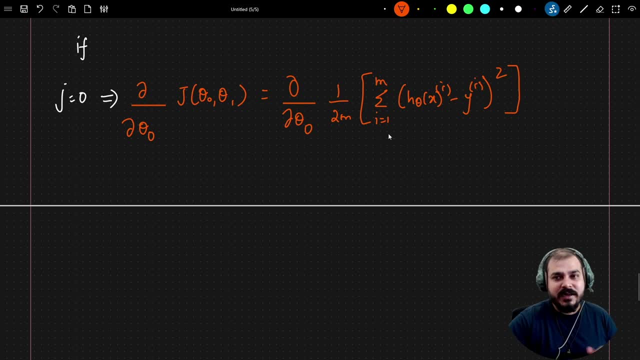 So x squared will be nothing but two x two minus one Right, Something like this. So whenever we have this x squared, whenever I try to find out the derivative with respect to this, it will be two x two minus one Right. This is what is the basic formula. OK. 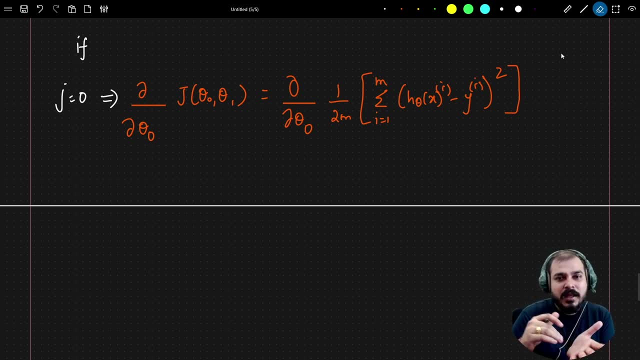 So these are simple derivatives, Guys. if you don't know, don't worry. OK, but just I'm trying to write out the convergence algorithm with respect to theta zero and theta one, because now we have a 3D graph, 3D curve, which will try to converge in one single point. 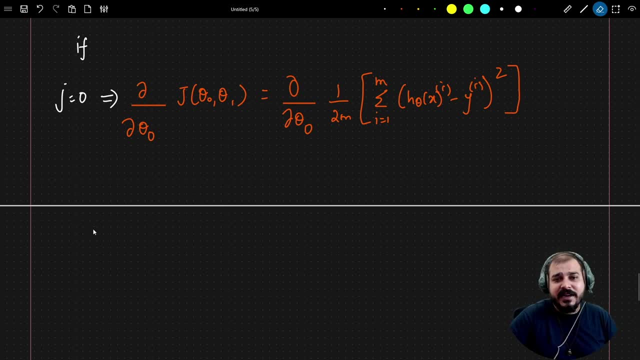 OK, so so, finally, here I can basically write after this, you know, in short, if I really want to write. So this entire value will get converted to something like this: So it'll be nothing but one by m, because two will be the same. 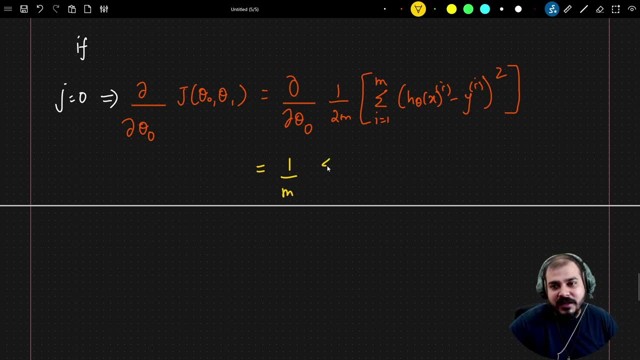 This two will come down. So two and two will get canceled, And here you can basically write: summation of i is equal to one to n. h. theta of x of i minus y of i, whole squared. OK, so yeah, sorry, not whole squared, because two will go down. 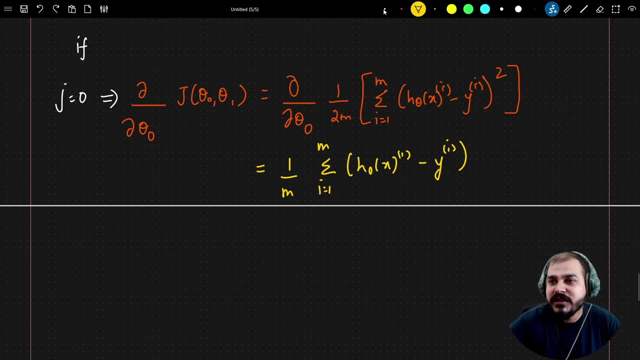 So this is my entire derivative and h theta of x. You know what is h theta of x? h theta of x is nothing but theta zero plus theta one x Right. So if I try to find out the derivative with respect, theta zero, so this will be one, and this is actually a constant right. this entire thing is basically a. 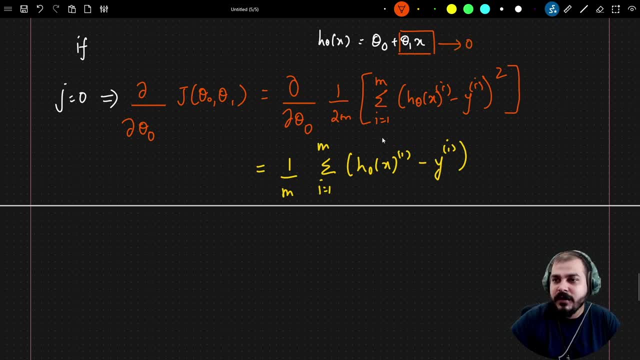 constant right, so this will basically become zero right. so theta of zero will be one, so it will be multiplied by one. so, in short, we will just be getting this specific term okay, so i hope you are able to understand it. what we will do is that, while finding derivative right, we'll replace this: 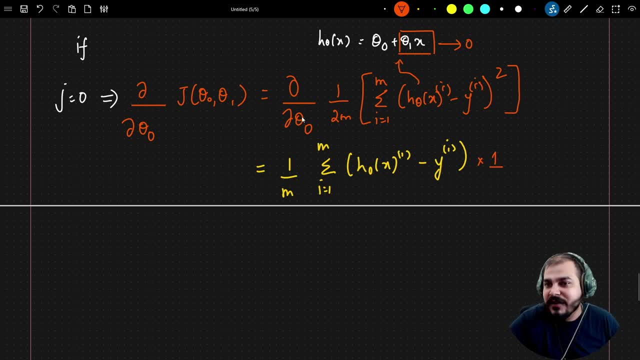 h, theta of x. with this equation, right, and since we are trying to find out the derivative with respect to theta zero, first of all it will be 2x, okay, and then we'll try to find out the derivative of this particular equation. okay, and here we know that if i try to find out derivative of theta, 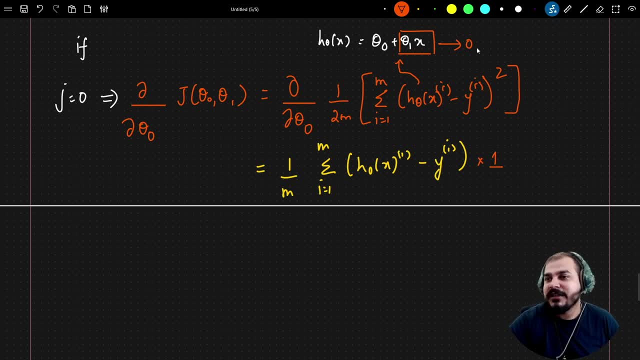 zero with respect to this zero. so here i'm going to get one, and this is a constant. this will become zero. that is how derivative actually work now. similarly, with respect to, j is equal to one. i'm just going to find out a derivative and this will now change as derivative of theta one. 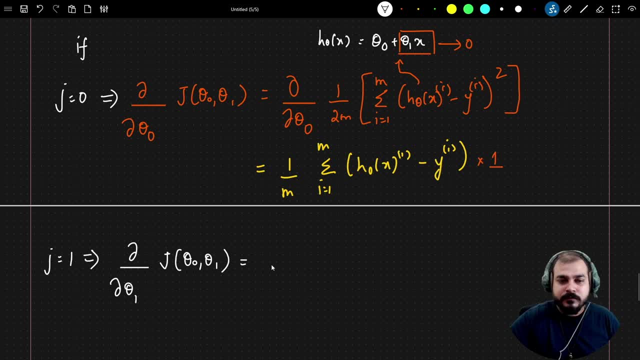 j of theta zero comma: theta one, okay. so here you can see derivative of theta one, okay, and then i'm going to just apply for this specific equation and it will be same thing. summation of pi is equal to one to m, and let me just equate this as theta of x with theta zero plus theta one into x. okay, theta zero plus. 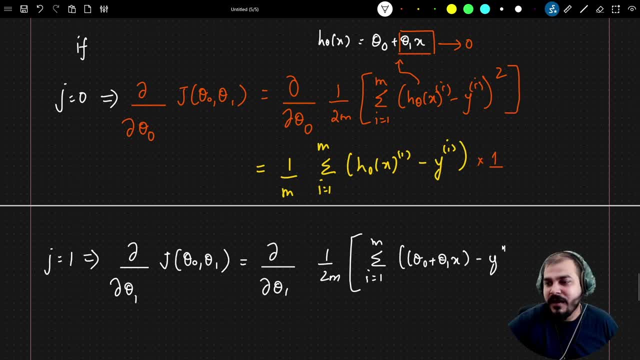 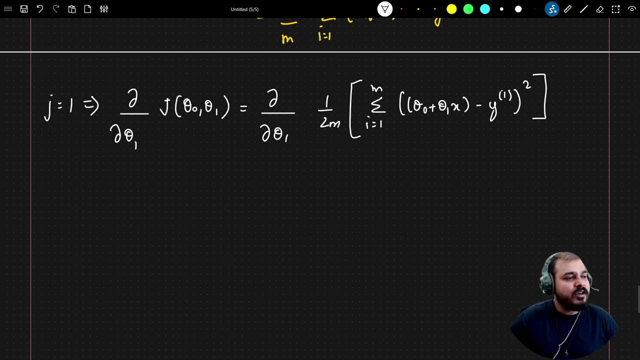 theta one into x. i could have replaced it over here, but it's okay, this is what i will be getting right now. we are just going to find out the derivative with respect to this specific equation. now, in order to find out the derivative, it's very simple. uh, again, i'm going to take this entire two. 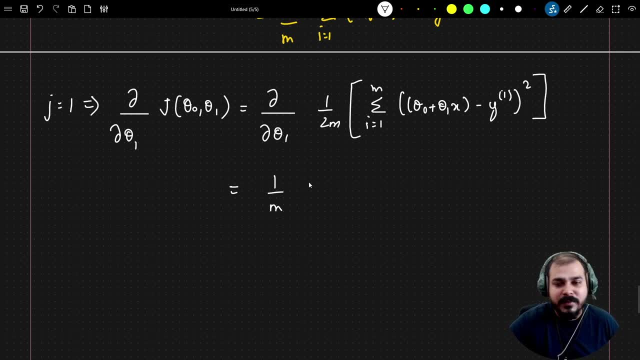 down, so this will be one by m and uh, here i'll be getting. summation of i is equal to one to m x. theta of x, which is nothing but theta zero plus theta one multiplied by x. okay, then it will be plus- sorry, minus- y of i. okay, so this will be my. 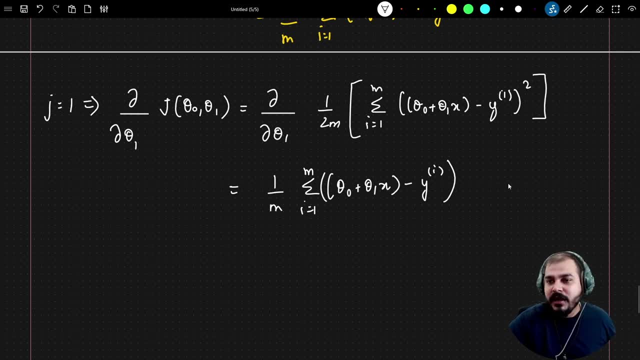 entire thing, then this entire thing will be going to the next step. okay, and from this you know that now theta one is not a constant right, because we are trying to find out the derivative with respect to theta one. so just just imagine, like, if i'm trying to find out the derivative of theta one, 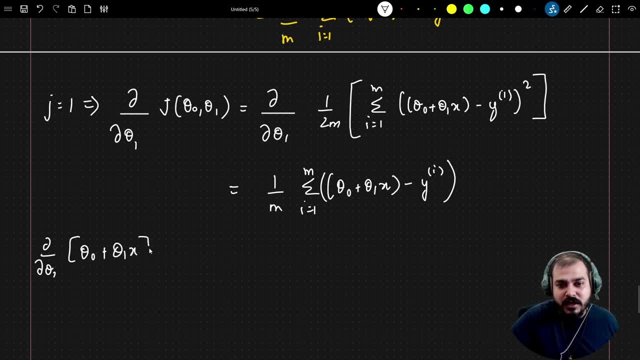 1 with respect to theta 0 plus theta 1, x. so what will happen? so, over here, theta 0 will become constant, theta 1 will be basically getting a derivative. so here, in short, if i try to find out the derivative, this will be x. so i'm going to just multiply by x over here, right? so this in? 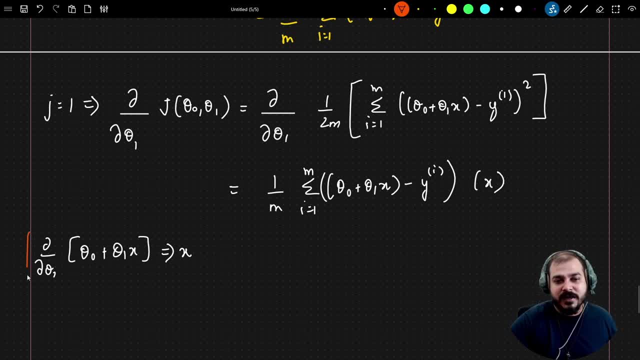 short will be actually helping us to find out the derivative with respect to theta. 1. right, so this is my entire derivative with respect to j is equal to 1. okay, i have just taken this and found out the derivative. it is x, so i have multiplied with x. okay, so these are the two things that we really 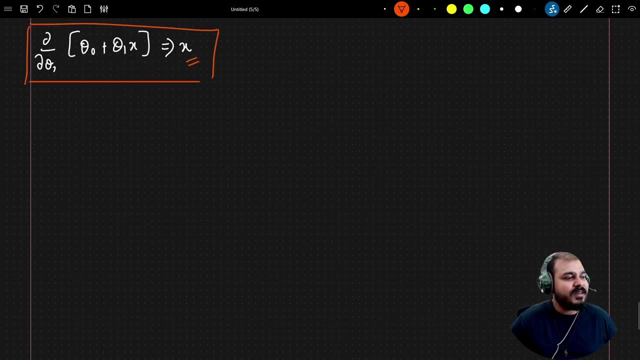 need to write. so, finally, i can quickly write something called as repeat until converge. this will be my final statement, a final conclusion with respect to simple linear regression: repeat until convergence. okay, and here we will be basically using two equations, two important equations. first of all, we need to keep on updating theta 0, so theta 0 will be nothing but theta 0. 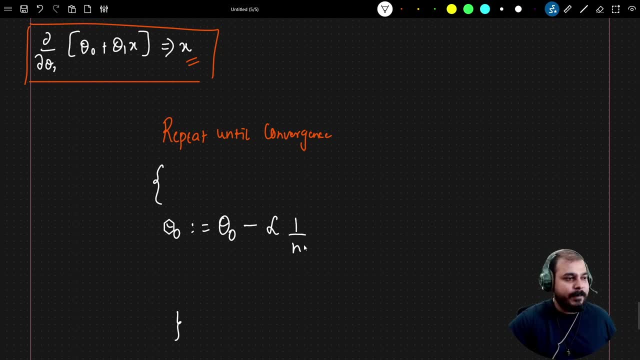 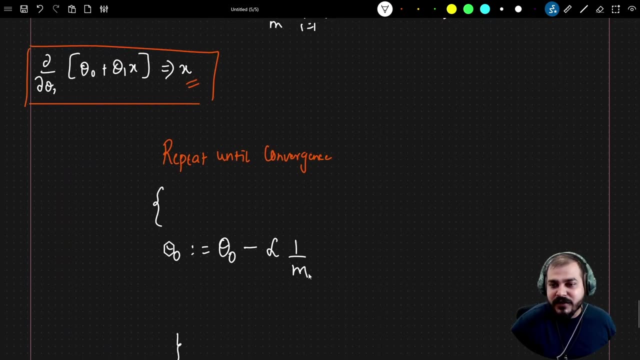 minus learning rate 1 by n, right. so what is theta 0 see with respect to theta 0? this is what over here i need to replace derivative of theta 0 with respect to j. j of theta 0 comma, theta 1. what is the derivative of j of theta? 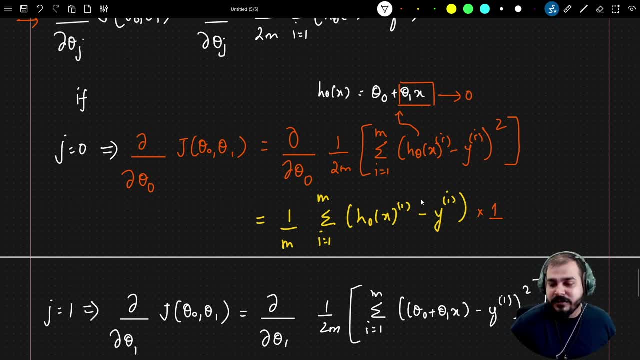 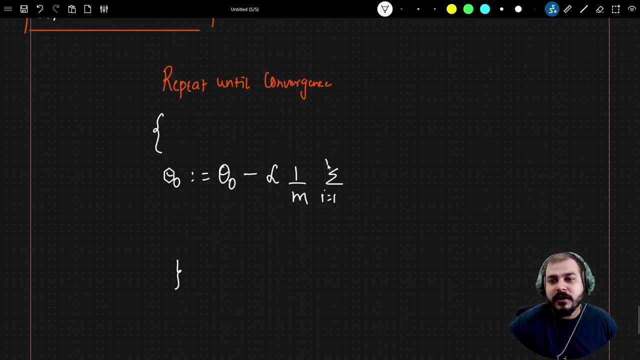 0 comma. theta 1 with respect to j is equal to 0. this is my entire equation, right? so i'm just going to write this entire equation over here. so it will be nothing but 1 by m, summation of i is equal to 1 to m, and here i will be seeing h theta of x of i minus y of i. 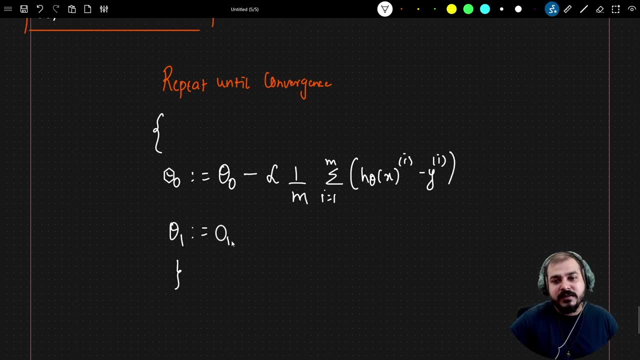 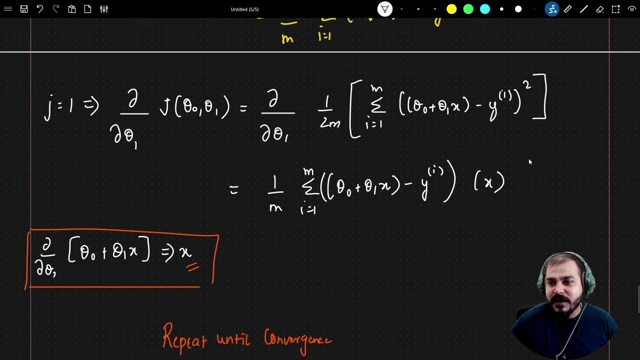 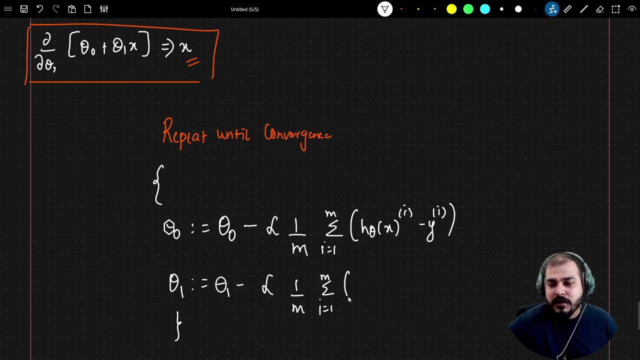 okay, and then theta 1 will get updated as theta 1 minus learning rate and derivative of j, theta 0, comma theta 1: what is the derivative? we got over here this particular equation, right. so here i'm going to basically write: 1 by m, summation of i is equal to 1 to m, and again i'll be having h theta. 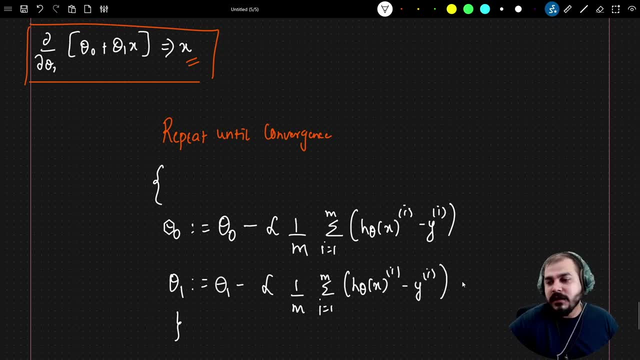 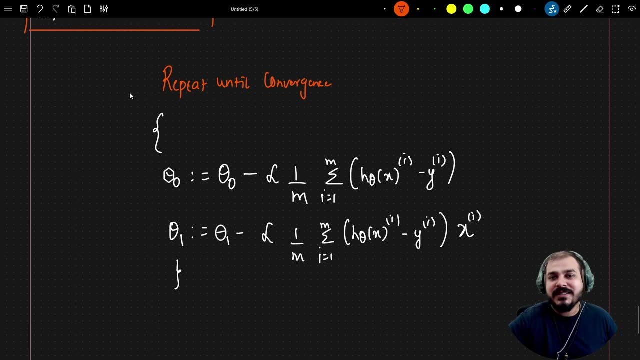 of x of i minus y of i, and here i'm going to use x of i. okay, so this is my entire equation that i specifically get, and this conversion is going to be the derivative of j theta of x of i minus y of i. convergence will be happening unless and until we get the best fit line, or we get the- uh, we basically. 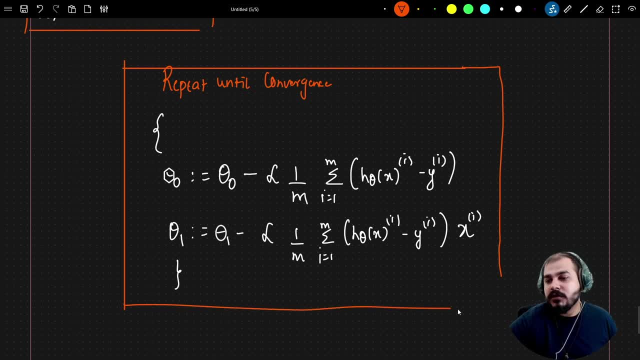 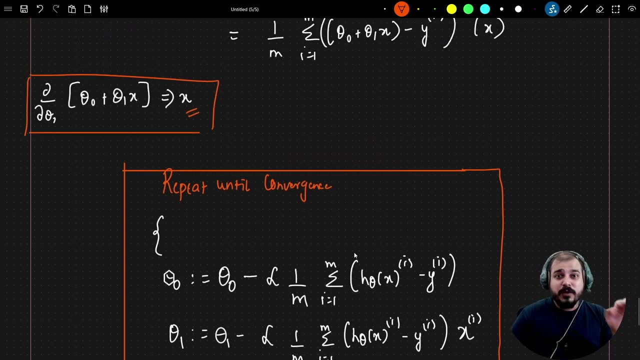 get the best fit line or we converge to the global minimum. so this is the entire thing that you really need to know. i know there are a lot of equations that have been used, but again, understand the phenomena, what we are actually doing. we are converging. we are converging in this gradient. 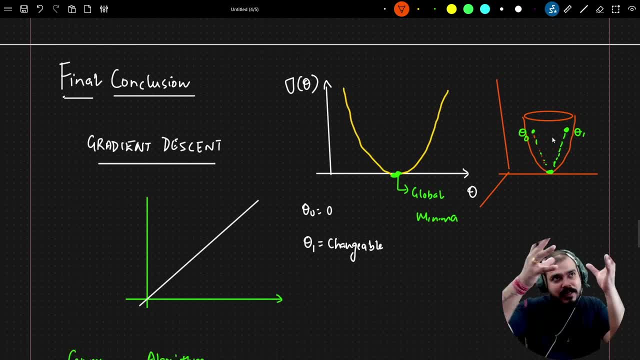 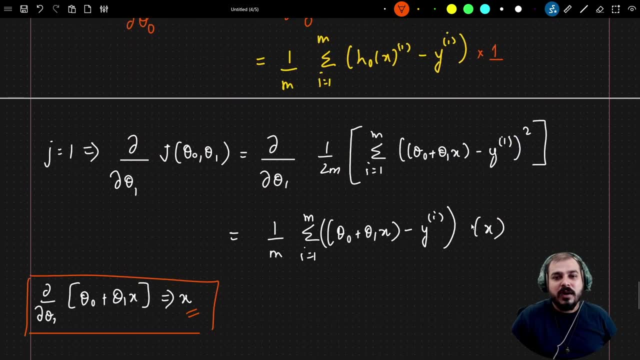 descent right. if i use theta 0 and theta 1, then it becomes a 3d curve- right 3d curve- and, at the end of the day, theta 0. wherever it is, we have to come to the global minimum. so, uh, i hope you have understood it. if you find any difficulty with respect to the equations, don't. 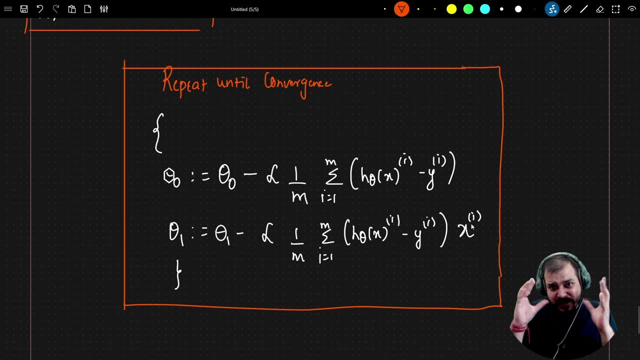 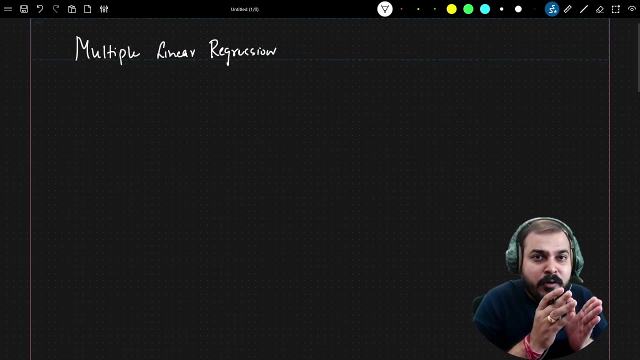 worry, okay, uh, because implementation of some amount of theoretical knowledge is required if you don't know the equation. also, implementation will be quite easy with the help of a scalar right. so, yes, uh, this was uh with respect to simple linear regression, and in the upcoming videos we'll see some kind of practical implementation. in our previous video we have 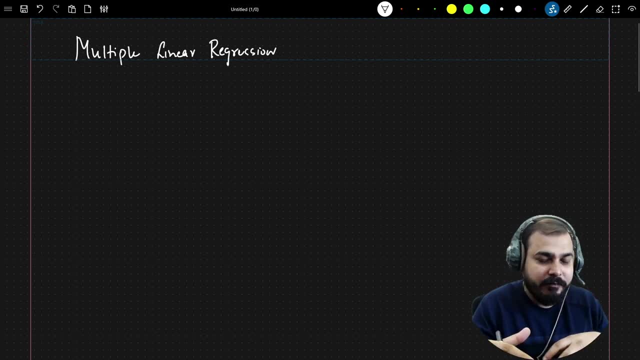 actually seen the convergence algorithm of the simple linear regression. in this video, we are going to talk about the convergence algorithm of the simple linear regression and in this video we are going to talk about multiple linear regression and we are going to just understand what is the basic difference between simple linear regression and multiple linear regression. in our previous 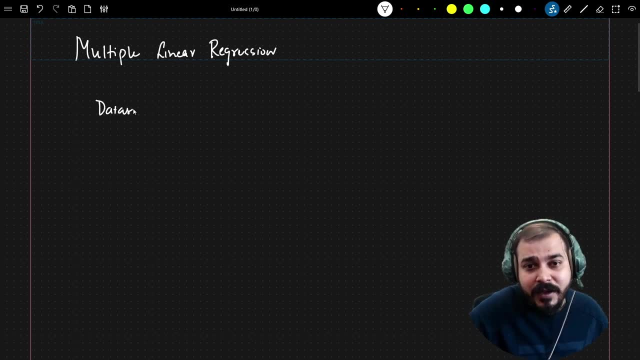 example. uh, when i consider our data set right, we have taken the example that my input feature is probably, you know, weight, so i really need to predict height. okay, and for this, you know, this is specifically one input feature over here, one input or independent feature, and this is: 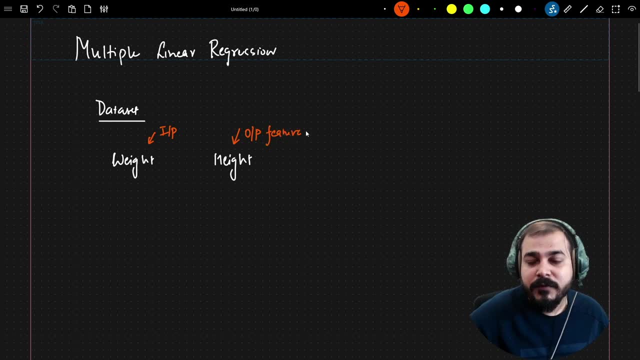 specifically my output feature. so what we did, with the help of simple linear regression, is that we tried to find out the best fit line and we understood the equation, the cost functions, the convergence algorithm of updating the slope. now, in this particular case, since i just have one input feature, so my- if i talk about the 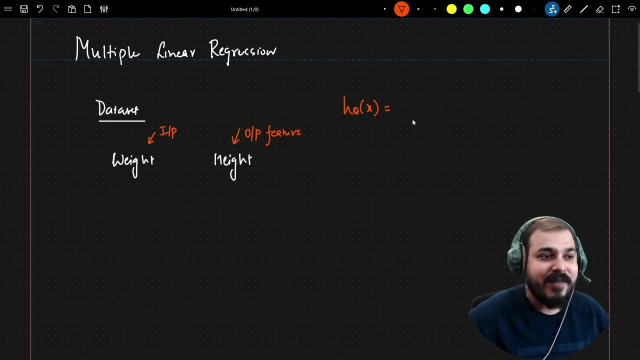 h, theta of x, which is the equation of the straight line which we have actually discussed. we are indicating something like theta 0 plus theta 1 multiplied by x. right now, over here, this x bcd basically indicates my input feature right. input or independent feature. independent feature right. 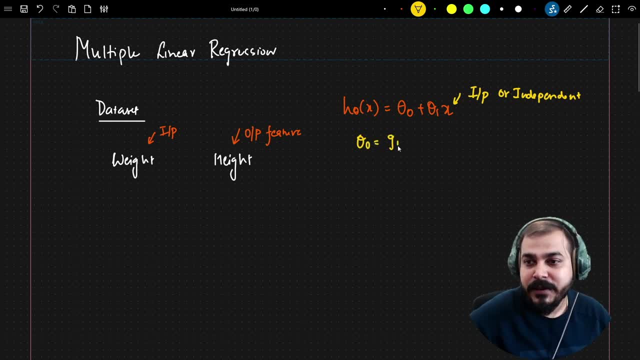 and obviously you know what is theta 0. theta 0 is basically intercept and theta 1 is nothing but slope. right now, what we were doing is over here is that we were trying to change theta 0 and theta 1. we will not change x, x, whatever is there in this training data set. 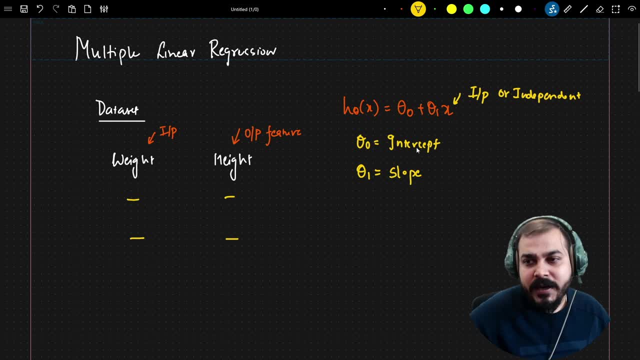 that only thinks we are going to take and probably train our model, right. so in this particular case, what we will do, we'll just change theta 0 and theta 1 and we'll try to find out the best fit line. now, what if in your data set you have multiple input feature? so let's 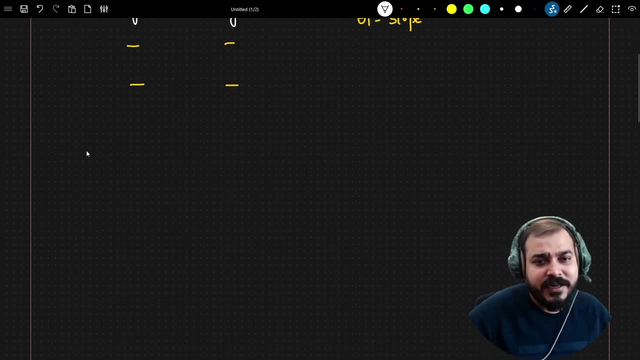 consider one simple data set. i call this particular data set, which is called as house pricing data set. okay, now, in this house pricing data set- and probably i'll show you this- all kind of data set when we do the practical right. let's say i have multiple features, like this number of rooms. 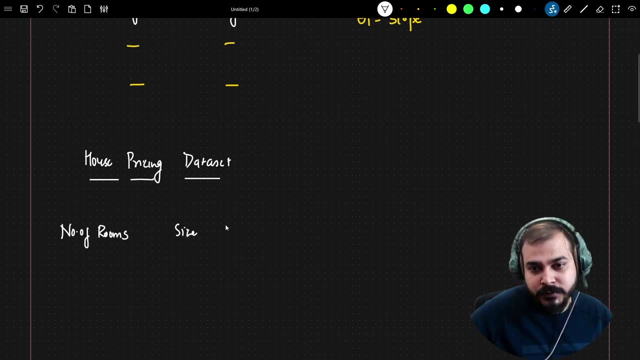 in the house, size of the house, okay, and let's say what is the location of the house and finally, i have something called as price of the house. so over here, in this particular problem statement here, you can see that i have four, four features over here, four features in total. 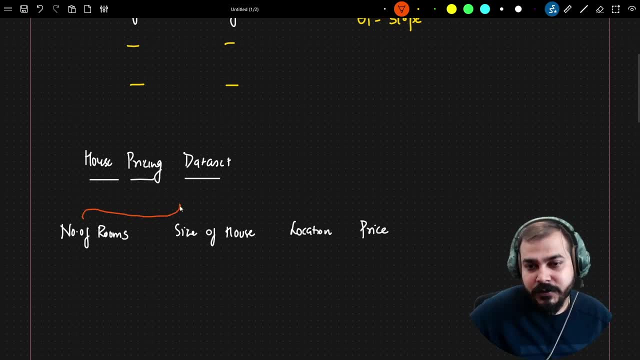 and this first three features are basically my input features. right, this first three features are basically my input features or independent features, so i'm just going to write this as now. in this particular case, you can see that i have more than one input feature or independent feature, and this is my output feature. 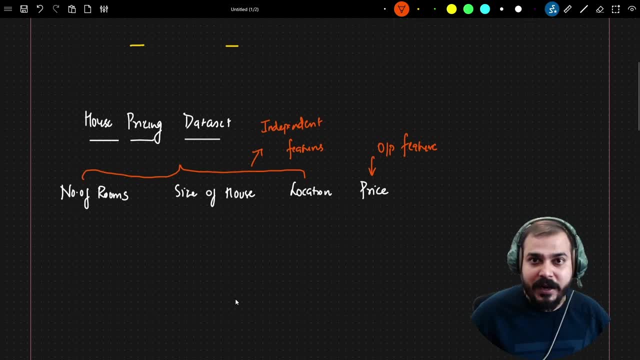 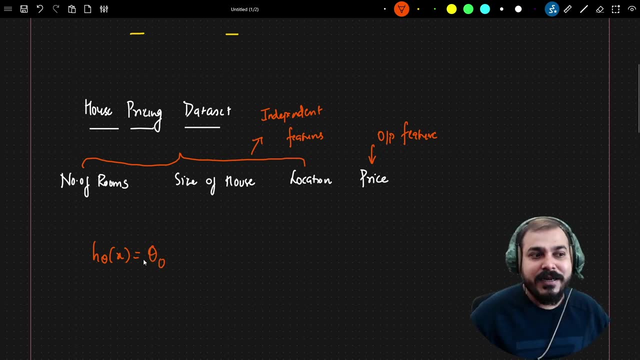 now, in this particular case, when we try to find out our best fit line, how does the equation of the best fit line look like? so now i'm going to basically use the same equation: h, theta of x, which is nothing but theta 0. theta 0 is always an intercept. there will always be one intercept for. 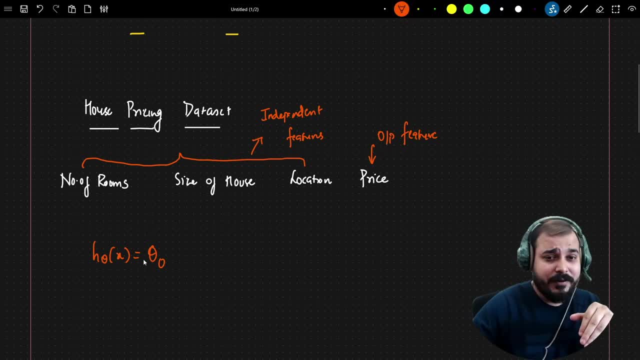 If I'm basically using a simple linear regression or multiple linear regression, there'll always be one intercept that we really need to use it Along with this, based on the number of features. right, Let's consider. number of rooms is my X1 feature. 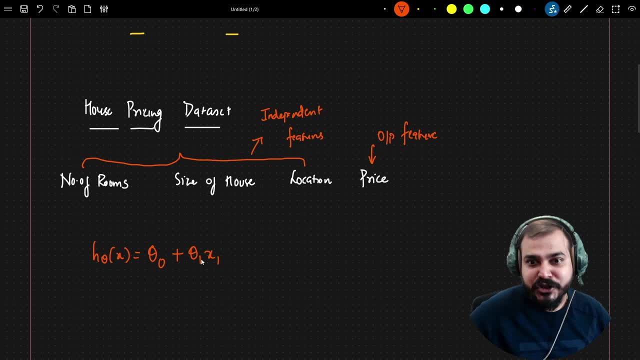 So for this we will be having another slope, which I'm mentioning over here as theta1.. Then I will be having, for my second feature, theta2.. So theta2 is the slope for size of house or coefficient of the size of house. 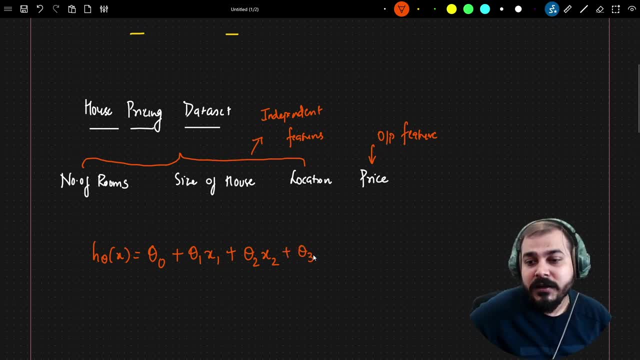 Okay, And similarly, location will be theta3, X3.. X3 basically indicates location, right, And theta3 is basically the coefficient. So this equation basically indicates my multiple linear regression. Okay, So in the case of multiple linear regression, 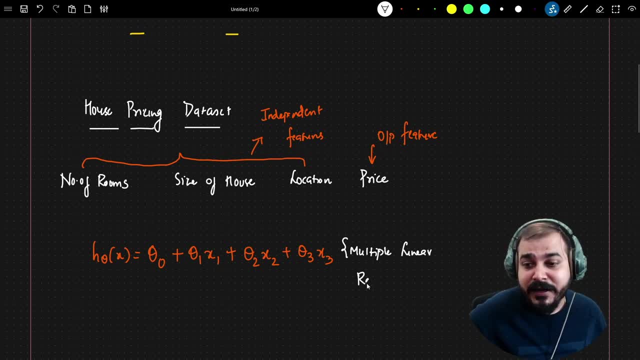 one important thing that you really need to understand is that we will definitely have many features. Okay, Here, in this particular case, I've taken three features. So, with respect to these three features, I will be having three coefficients. So over here, theta1, theta2, and theta3. 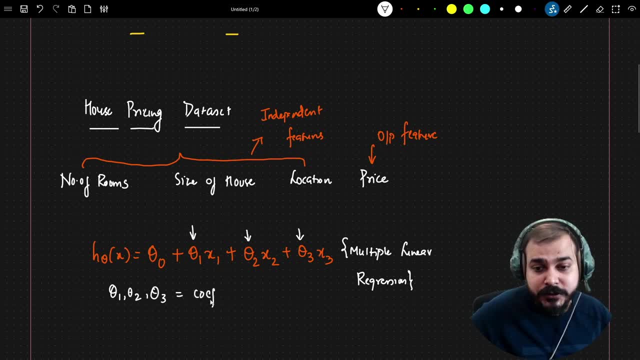 are basically my three slopes or coefficients. Okay, So as the number of input features increases, that many number of coefficient will increase, but your theta0 will always be the intercept and you will have only one intercept all the time. Now, in this particular case, if I probably talk about a gradient descent, 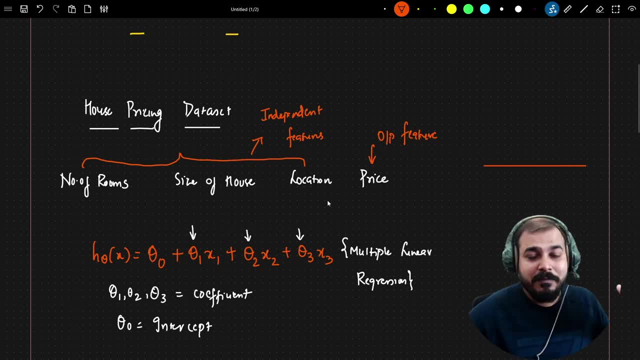 our gradient descent. you know, let's say, since there are three input features, you know, in this particular case, when I draw with respect to theta, theta0, not theta0. So let's say theta0 is here, Then I have theta1 over here and probably we cannot draw a 4D diagram. 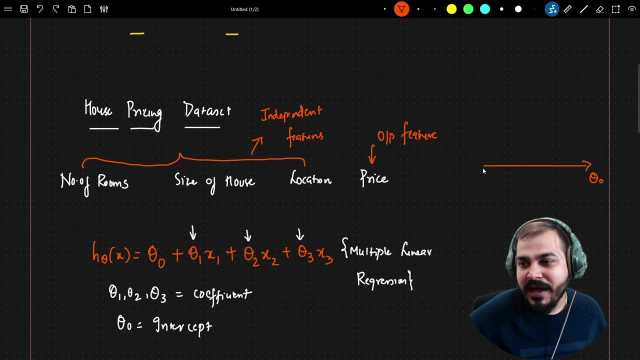 So let's consider just two features Here. I'm just considering theta0 and theta1.. Okay, And with respect to this, suppose I have j of theta over here, right? So we usually get a different types of diagram which will be looking like a inverted mountain.